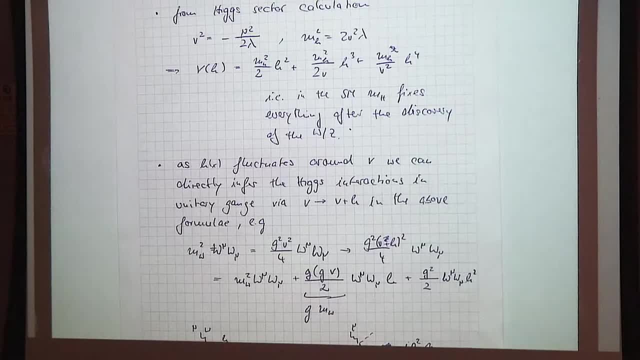 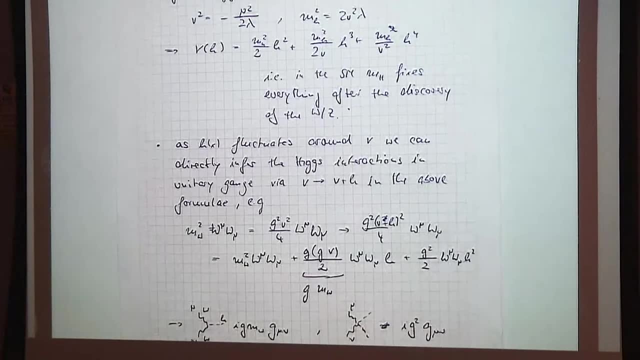 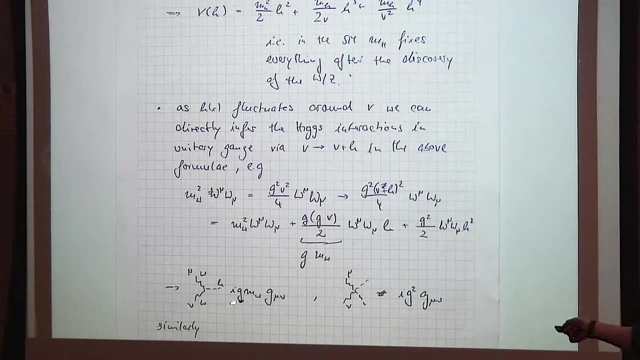 space times, the dynamical higgs field. okay, so this is always the sort of characteristic thing that arises when you do a electroweak symmetry breaking, so you end up with a Feynman rule that looks like this: so two of the w's are coupled to one: higgs boson and the coupling strength. 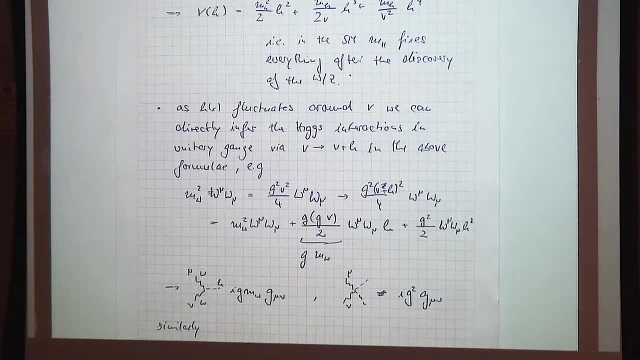 is given by some phase that actually never really matters, unless you- you do it inconsistently- times the weak coupling strength, times the mass and then of course the Lorentz structure. here this guy is just rising purely from a gauge interaction, so you only deal with the g squared, g, mu, nu, okay, and in a similar way. 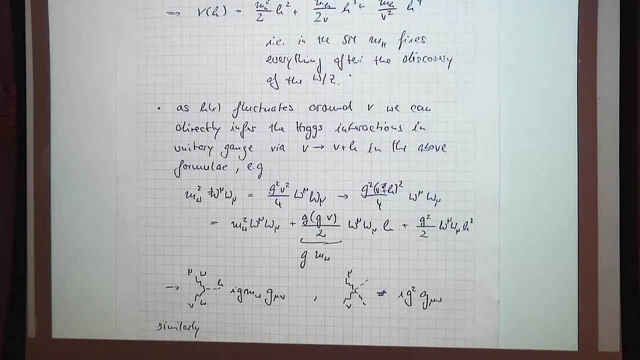 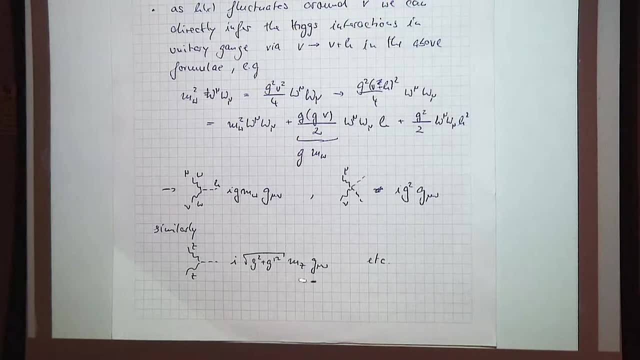 we can already guess what will be the interactions of the z's with the, with the higgs. its characteristic coupling was the square root of g squared plus g prime squared, where g prime squared is the u1 hypercharge coupling. and then you have the g squared, g mu, nu, and then you have the g squared. 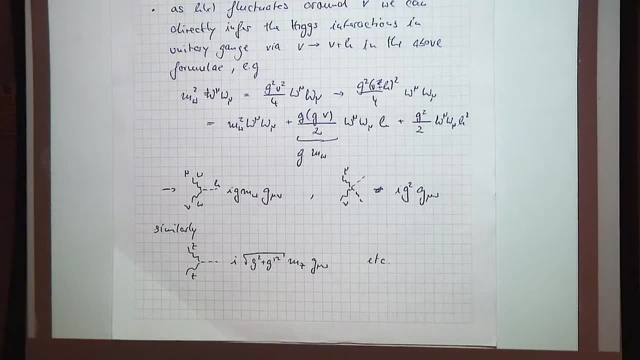 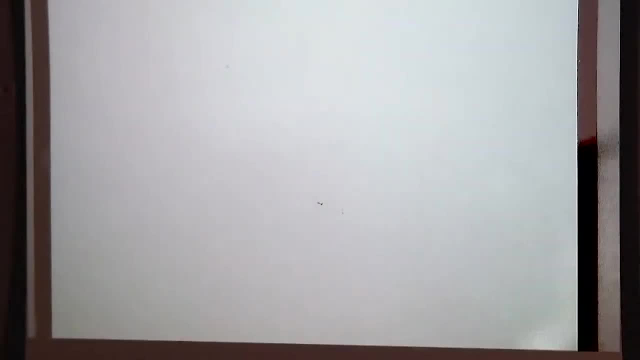 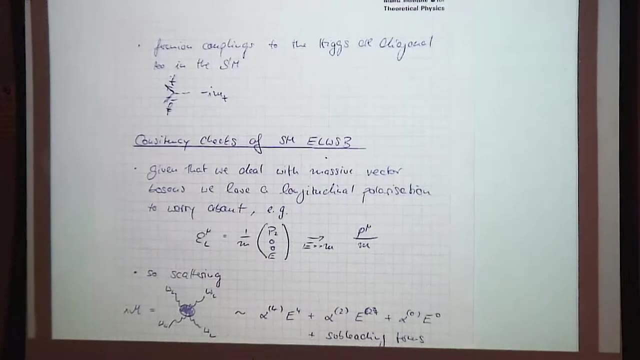 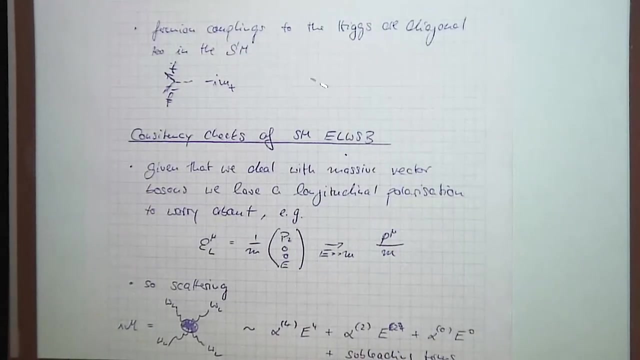 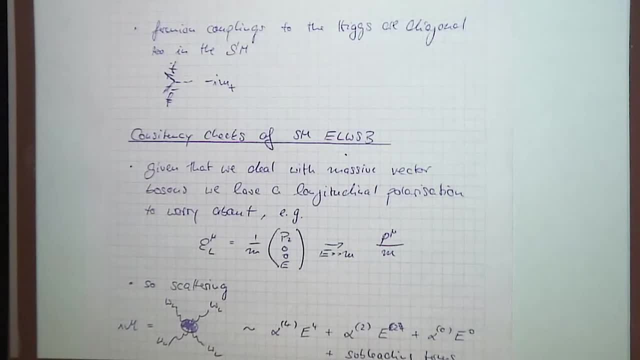 vector section. this is the vector section. so now you need just one value. we can even around the fermion mass and you see that the Higgs couple is proportional to the mass itself. So this is fairly straightforward and I'm not going to show you all of this here. but 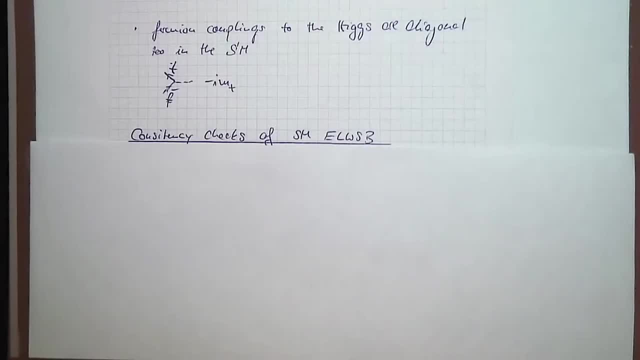 you can see that now we want to deal a little bit with consistency checks of electroweak symmetry breaking. Are there any questions concerning Feynman rules? Fairly straightforward. So what we want to achieve now is: well, what we have achieved is that we have all these. 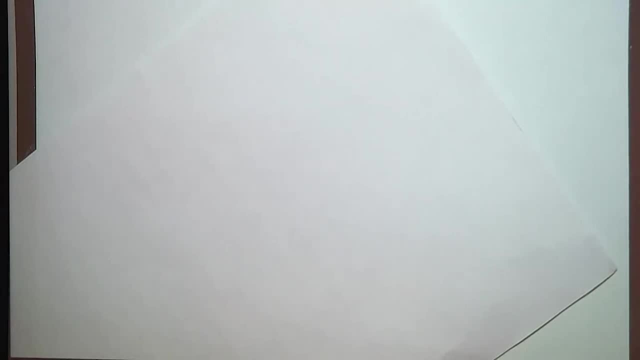 interactions. we have masses. now we need to worry about whether this entire thing in a quantum field theory sense, especially when we apply perturbation theory as expressed through these Feynman diagrams- really makes sense. And for this let's have a look at: 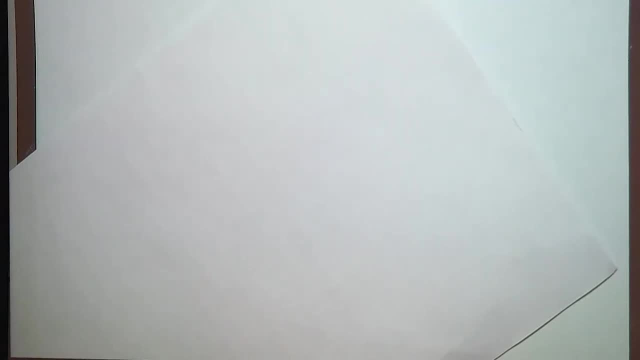 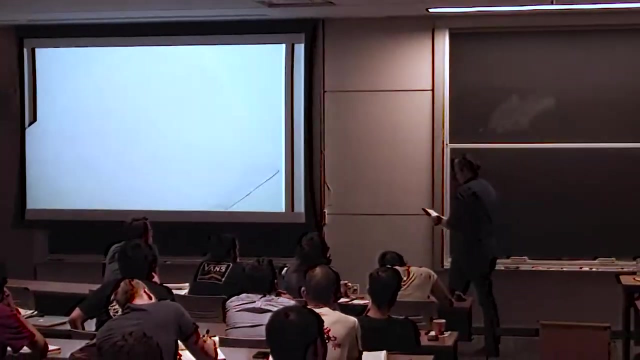 a few consistency checks And they were quite. they gave the entire field field quite some direction and it makes sense. essentially that's the main motivation of how we built the LHC and how the LHC was conceived as a machine. So let's have a look at what 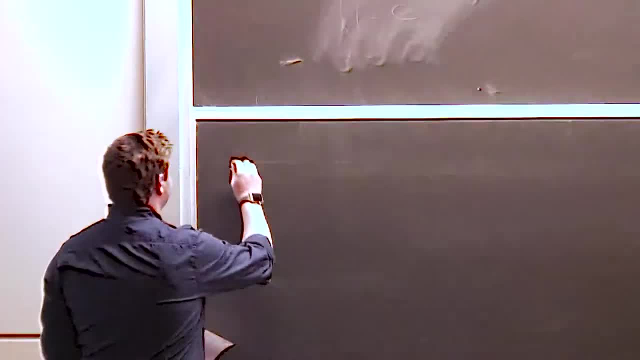 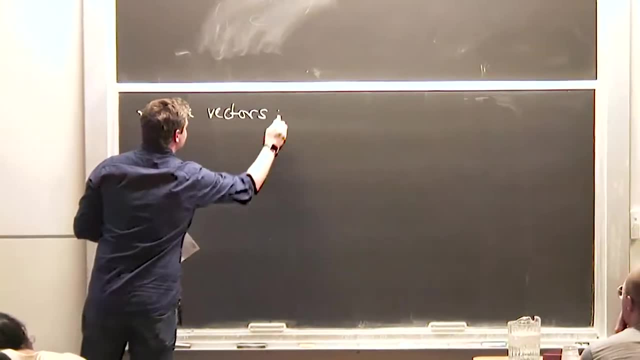 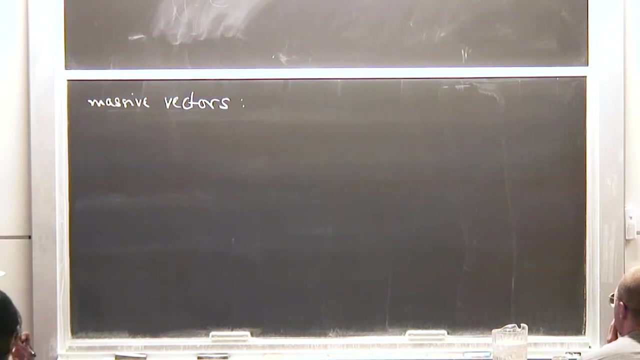 we have now at our disposal. So now we have massive vectors and you can think of it in unitary gauge. So we now have to deal with 3 degrees of freedom for our gauge fields because they are massive. So the photon field- we had this last time- has two transverse polarizations. but now 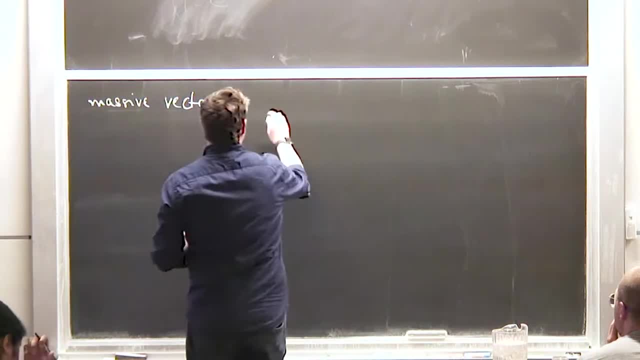 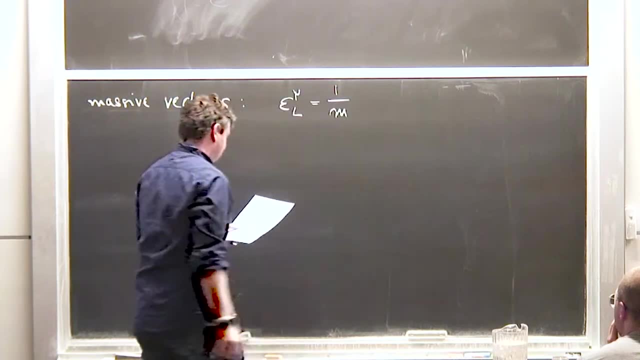 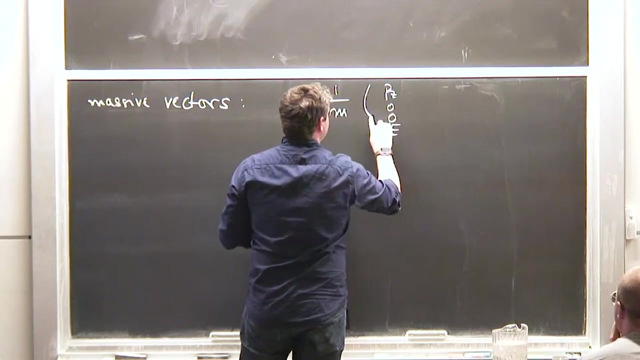 the massive vector picks up a longitudinal polarization, And that longitudinal polarization can be written as like this: in its rest frame, where you have Pz, and then everything is just aligned in z direction for convenience, And that of course only exists if the mass 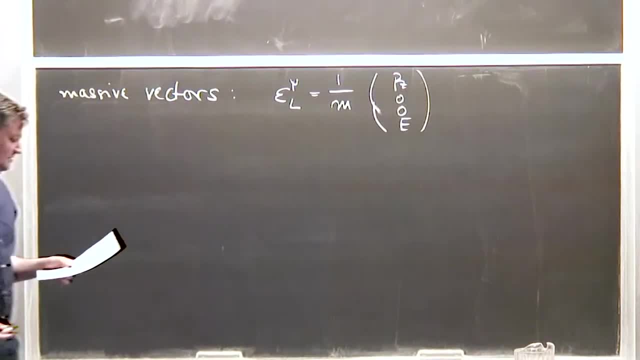 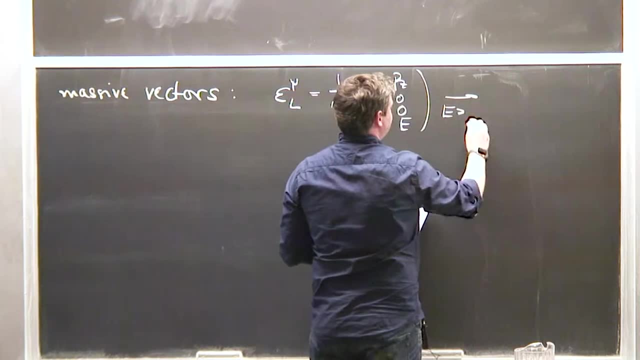 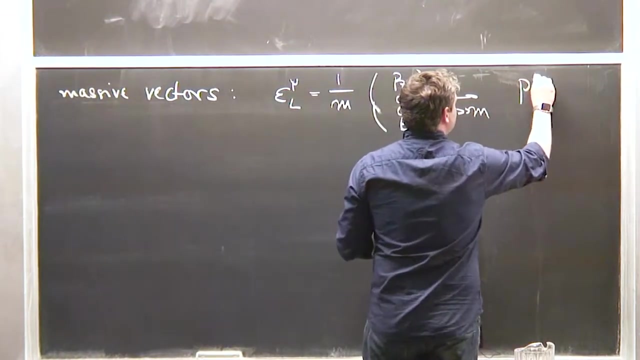 is really non-zero. If you set the mass to zero, it doesn't really work. So the thing that we can see here now is if we go to energies of these gauge bosons which are much, much bigger than their mass, then this will scale like the full momentum itself, divided by the 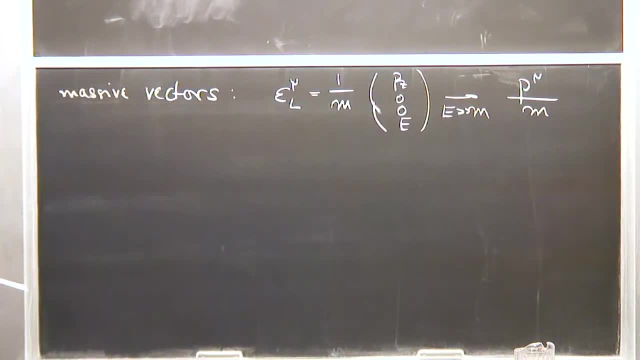 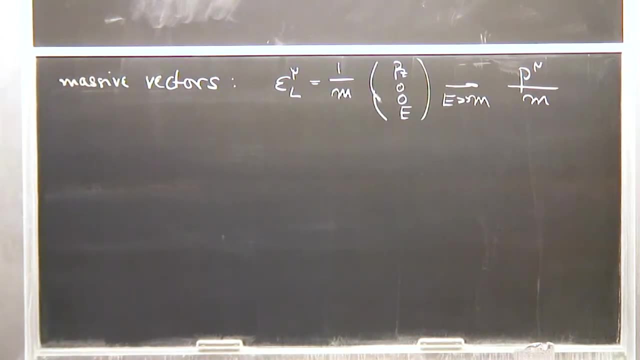 mass, All right. So, and that is potentially dangerous, okay, Because you know the mass, the mass of the mass is very big And that is very, very dangerous. And so what we can do is we can do the function of the H-vertices And we can do this with the H-vertices. So 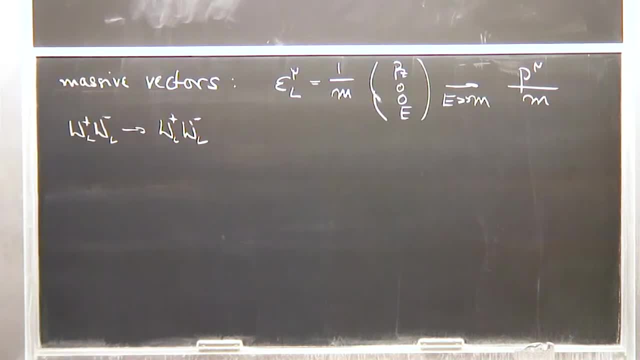 this is the H-vertices, And when we think about quartic H-vertices you have, for instance, WW scattering, And if you look at the longitudinal degrees of freedom, then you can write down a whole bunch of Feynman diagrams that contribute to this. So, the first of all, the first one, 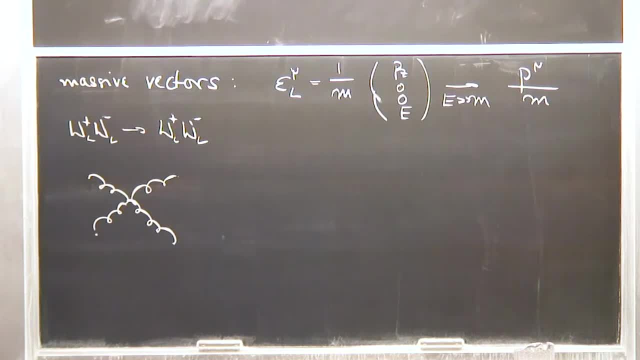 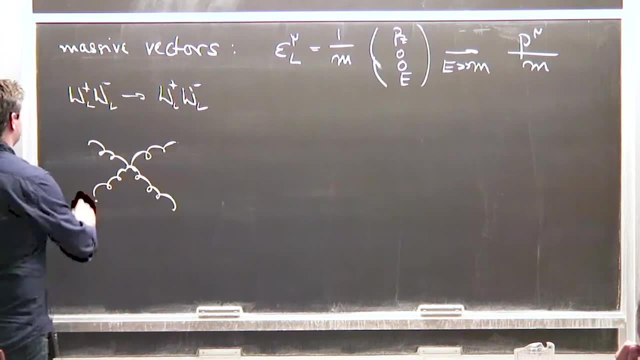 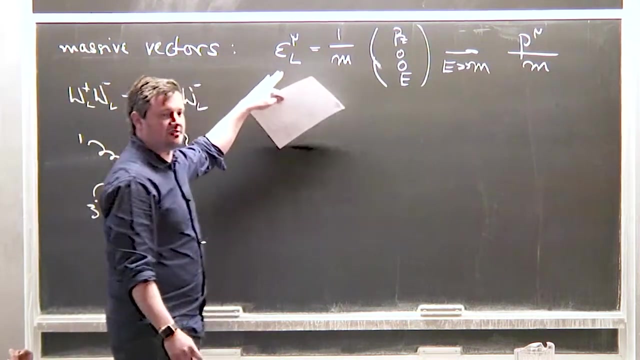 is of course, the quartic vertex, And that is just a series and cobbled together versions that you can look up in a quantum field theory textbook, and but in the end it boils down to products here of of scalar products of the involved longitudinal polarizations of the gauge bosons. 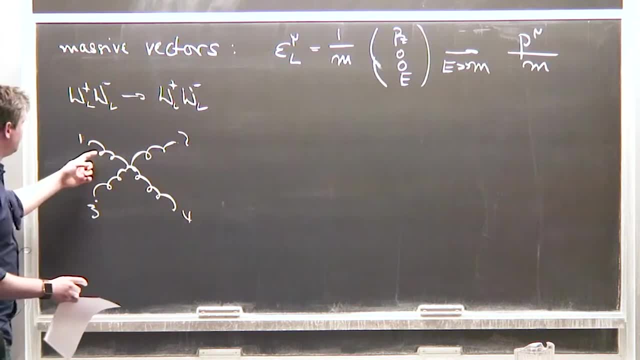 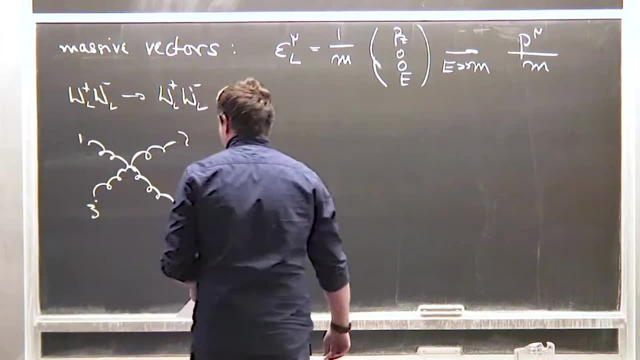 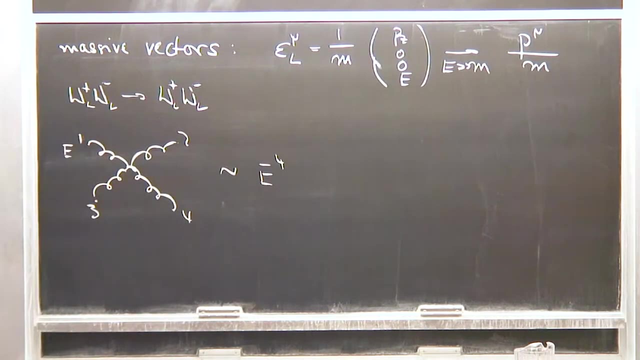 and because now each individual leg scales proportional to the energy. this Feynman diagram here scales proportional to the energy, to the power of 4 if these legs carry an energy characterized by E. so this Feynman diagram alone will create a massive enhancement with the energy of the incoming longitudinal W's. 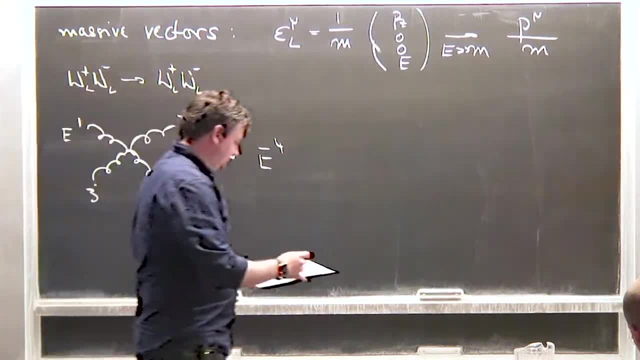 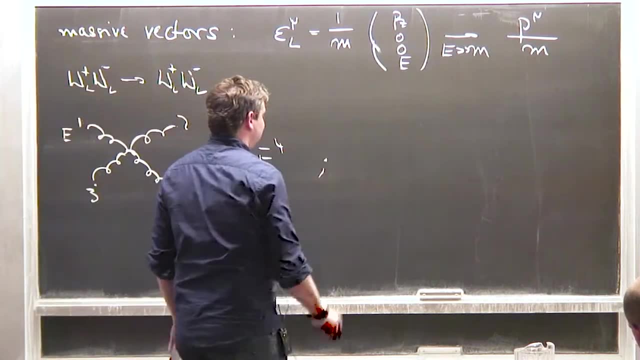 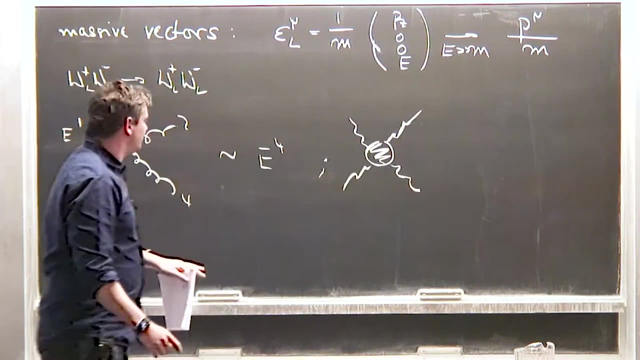 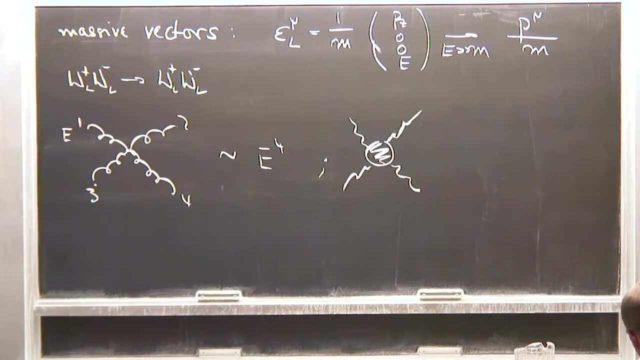 so if you now look at the complete amplitude, so this is just motivating as one part of W-W scattering. so if you look at the whole thing here, you can see that just by looking at the what is the maximum amount that you can increase your amplitude at high energy. 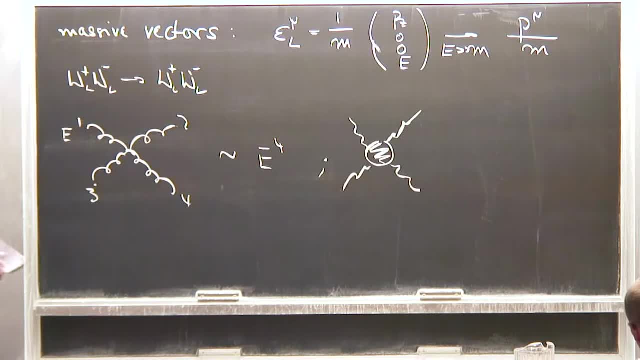 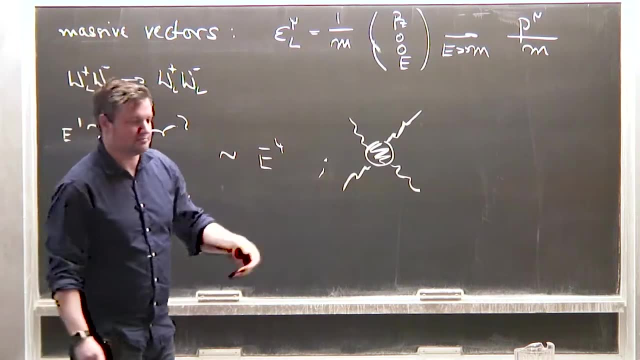 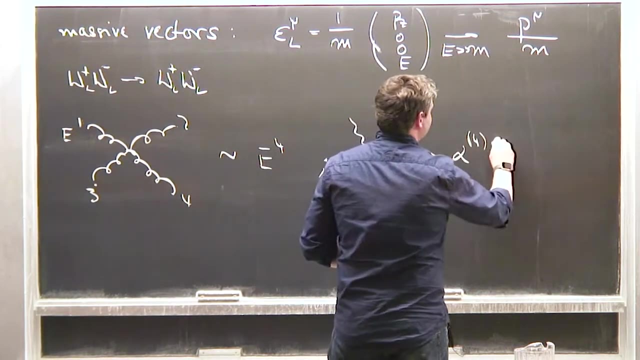 so essentially what I am trying to do is write down a Taylor expansion of this particular amplitude. so I know naively there will be terms: E to the power of 4, then everything below that, so this will have a form that scales with: alpha to the power of 4, E to the power of 4. 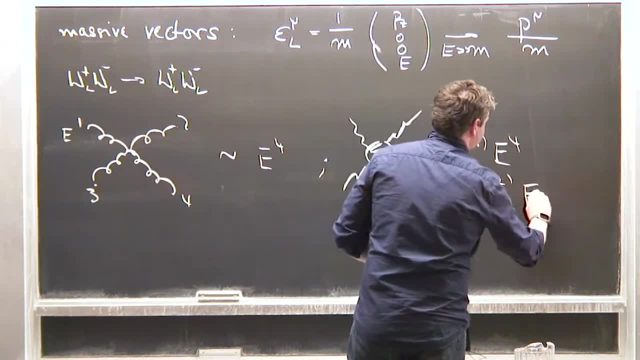 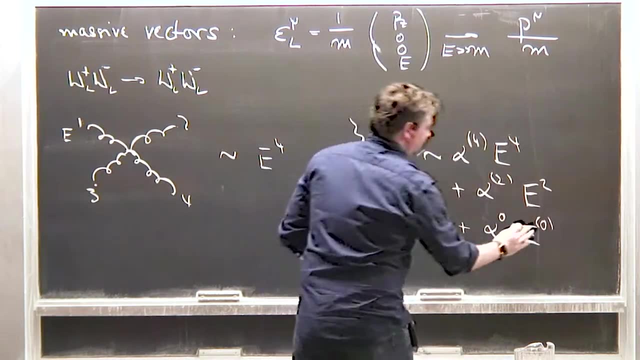 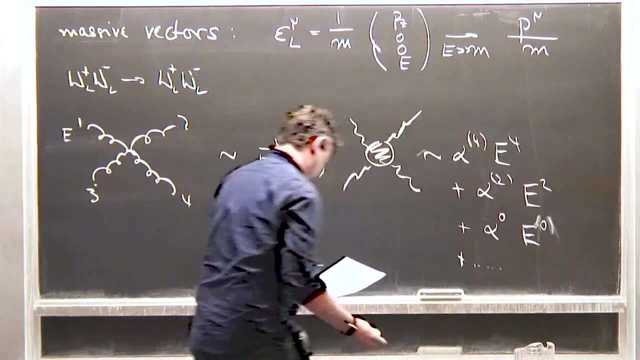 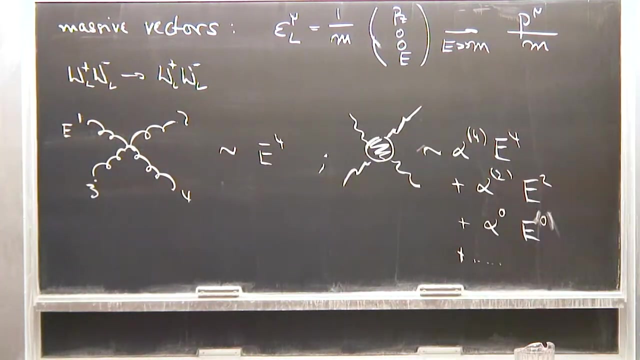 plus alpha, 2, e squared. plus alpha naught, e naught. And then so constant terms and I'm not really worried about additional terms here. So these terms I don't really care so much about because they are not really dangerous. So these terms proportional to e, to the power of 4 and e squared, 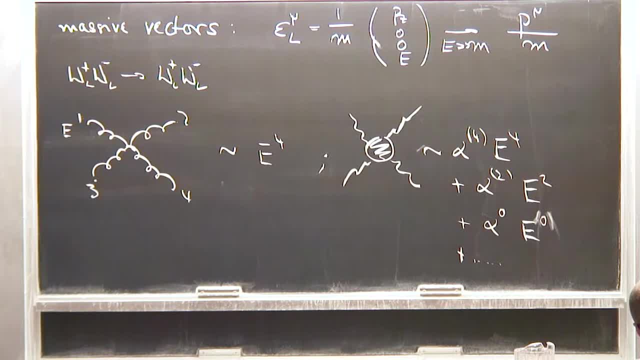 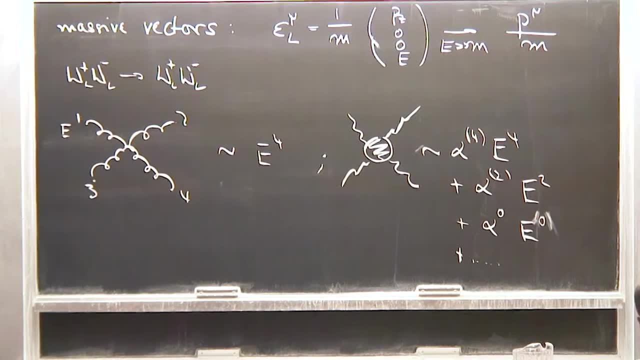 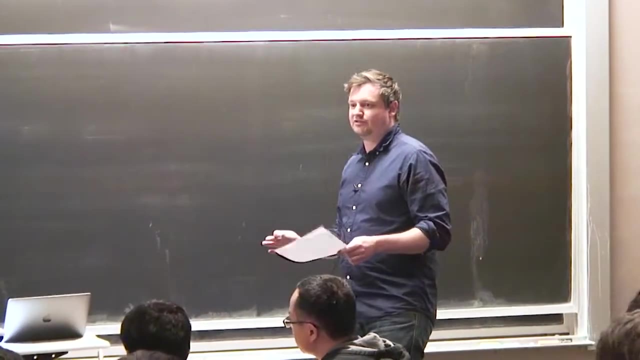 they can really harm our probabilistic interpretation of the scattering process, because diverging amplitudes means diverging probabilities, and this should not be the case. We started with a Hermitian Lagrangian. This implies a unitary S matrix, But now I truncate my series expansion here. 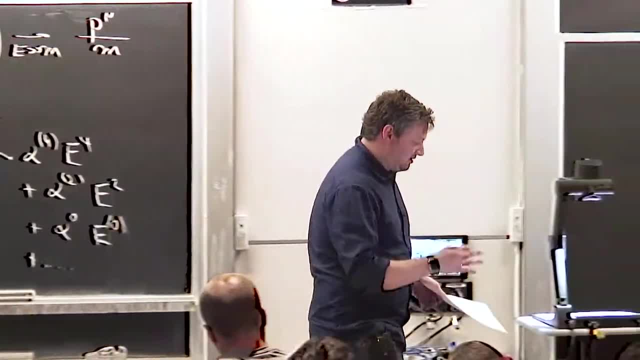 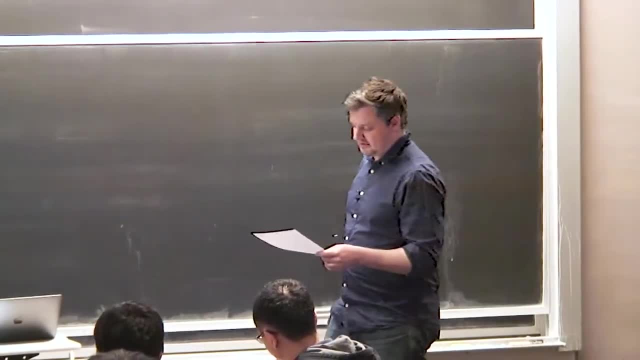 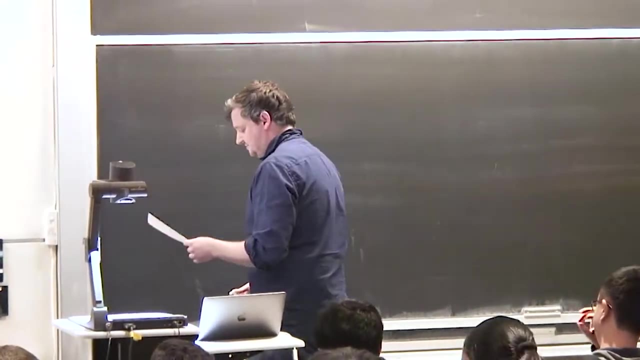 maybe at leading order. so just purely applying perturbation theory might actually violate this concept of unitarity, ie probability conservation. So I need to make sure that nothing crazy happens here, Otherwise we are at dead end and we can't do calculations for the LHC. 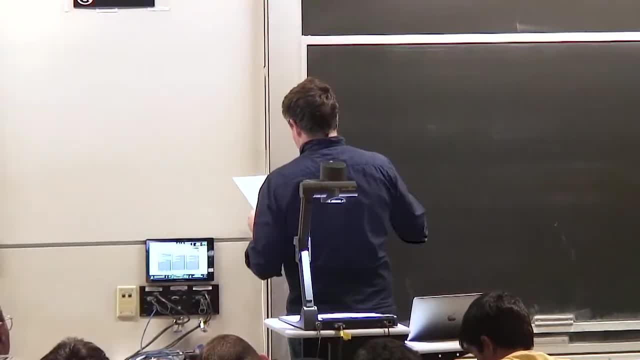 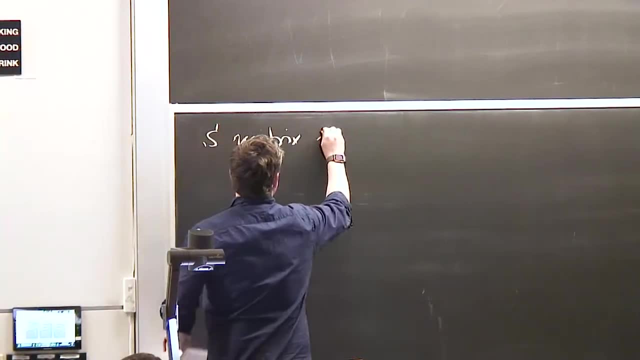 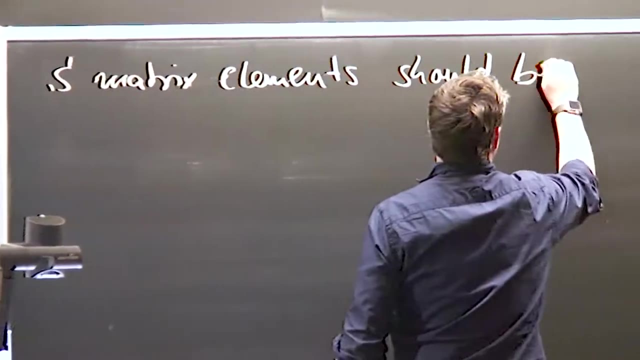 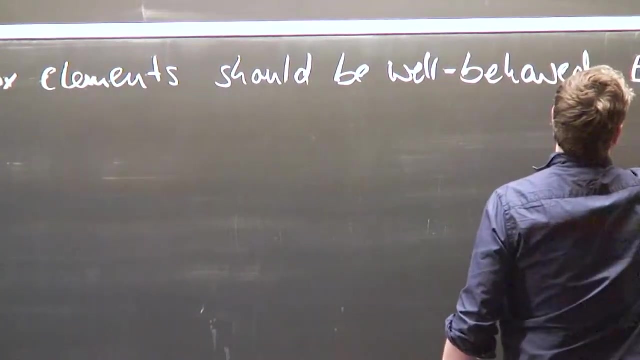 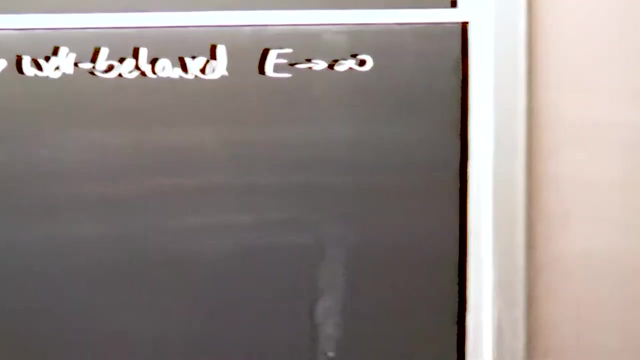 Okay, so S matrix element ie 0.7V Nz should be well behaved in the ultraviolet. so if you go to e, to infinity, so, and they will be, but maybe nonperturbitantly okay. 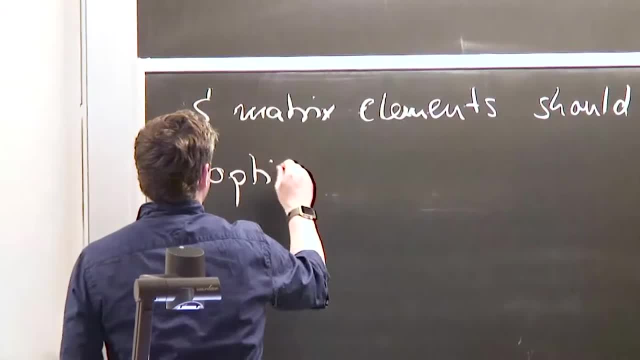 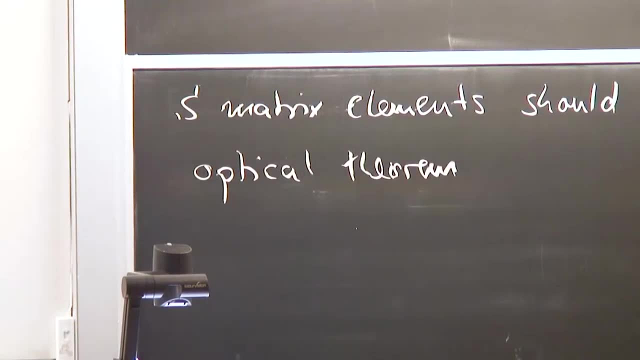 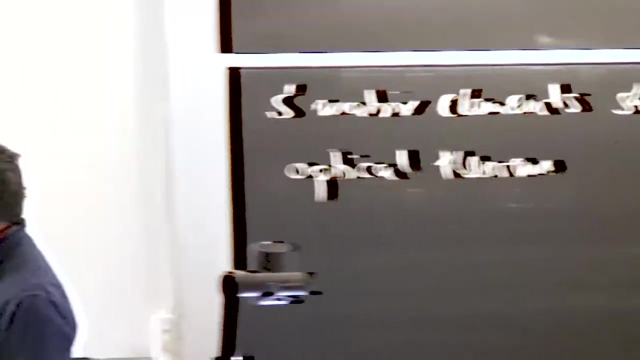 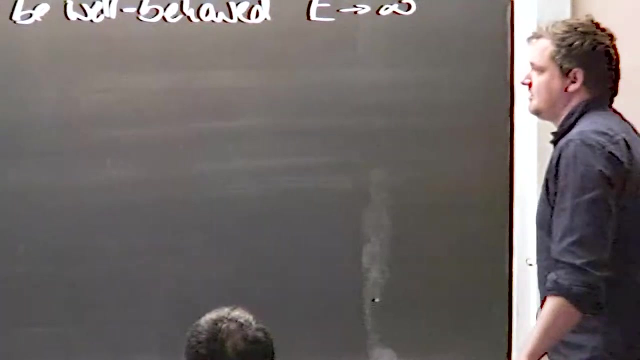 And this is what we want to check. So the optical theorem allows you to make a sort of strong statement based on zero-path wave scattering here. So you essentially write down this amplitude and you project it onto Legendre polynomials. So you look at angular momentum decomposition of that amplitude. 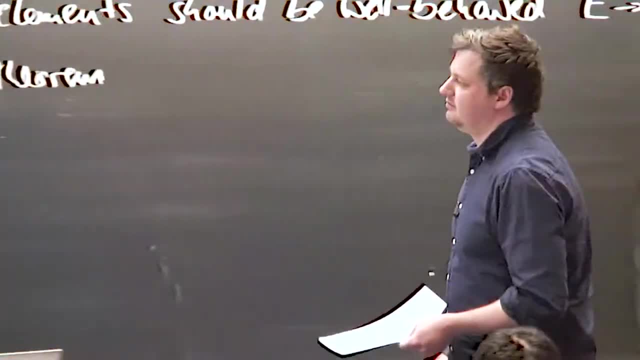 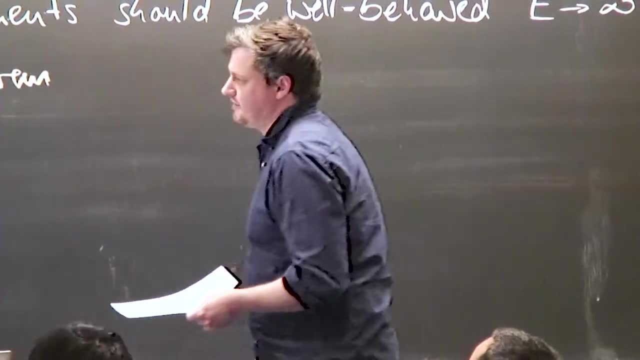 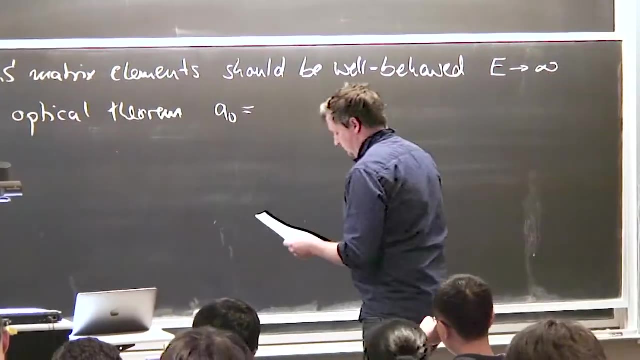 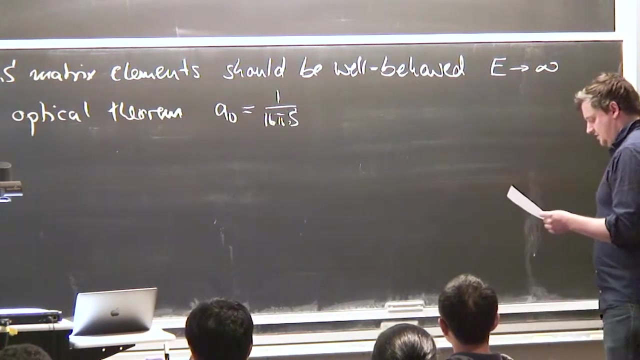 And then with increasing angular momentum typically the impact decreases. so the zeroth partial wave is really the most dominant one here, And that tells us that you can write A naught as 1 divided by 16 pi S, where S is just the Mandelstammi, so the center of mass energy squared. 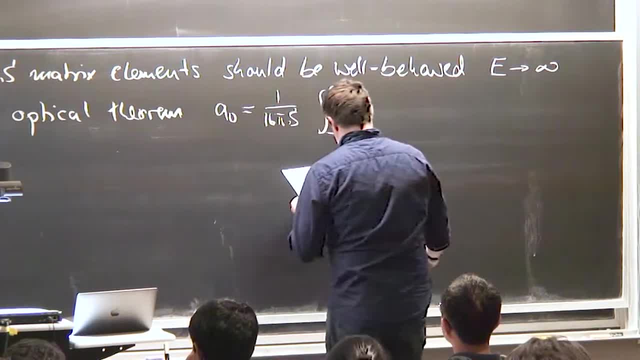 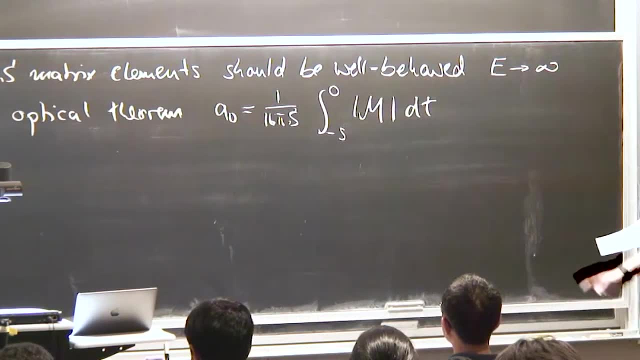 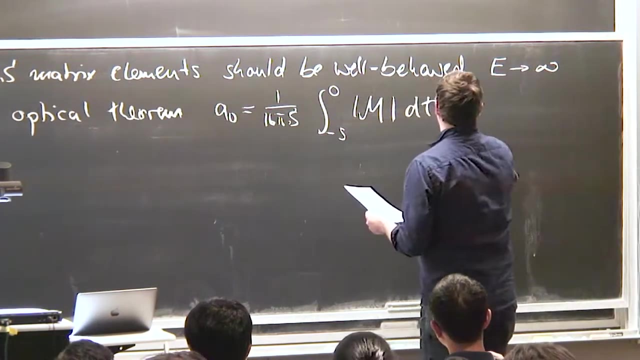 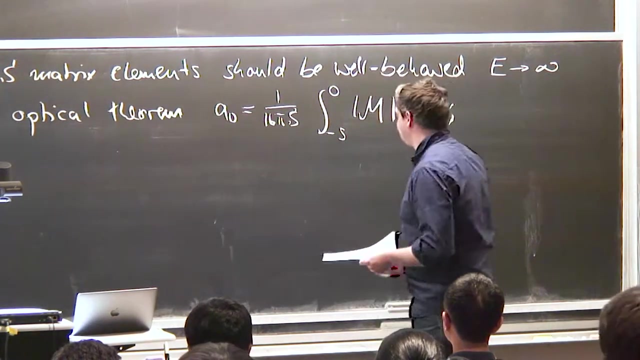 And you integrate from minus S to zero The absolute value of M over Mandelstam T, So where M is the complete amplitude, And if you look at this then you can. Unitarity conservation then means a constraint on A naught. 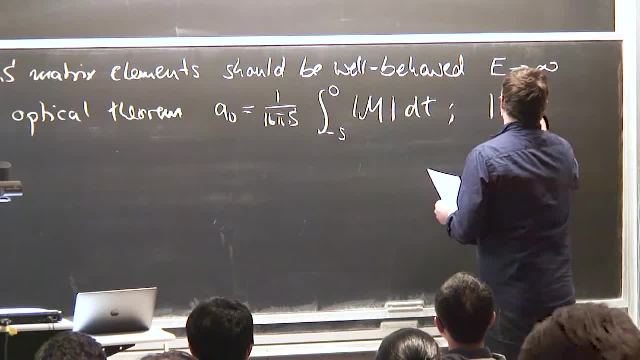 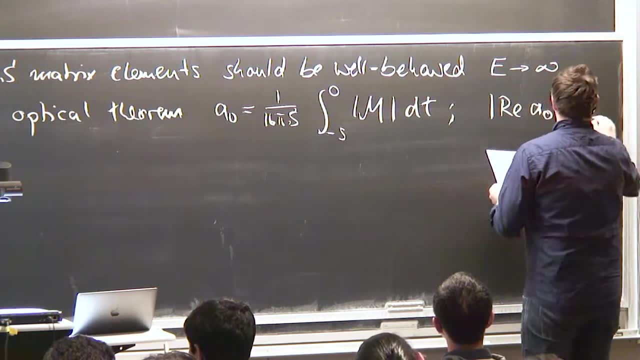 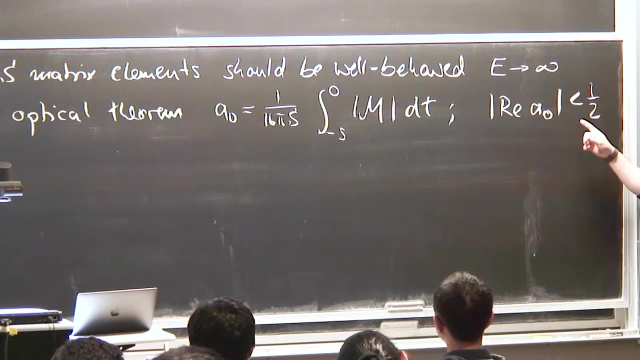 And there are various versions of this and we can have a look at any of them. really, And we One of this would be that the real part of this is smaller than 1 half. So if you violate this, then you break unitarity in a perturbative sense. 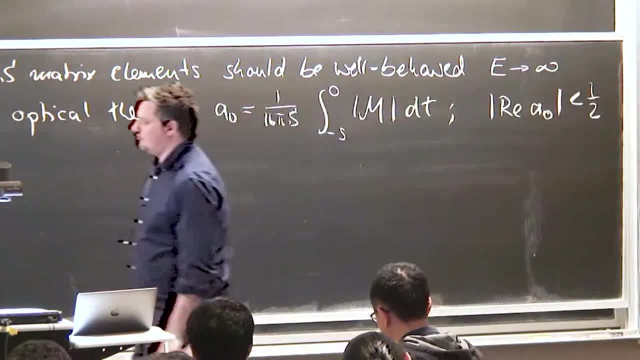 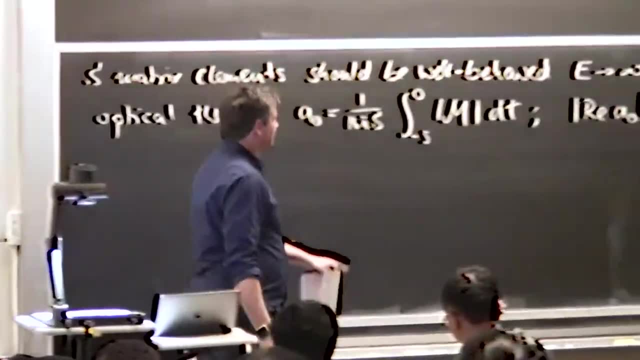 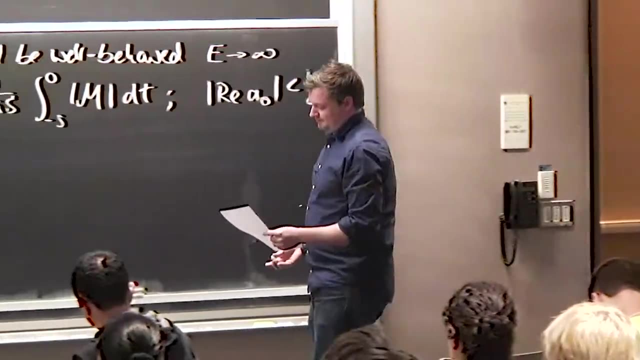 So you can already see that this can happen, really, if you allow for increases of energy with power 4 or 2.. So if you go to high enough energies, this will grow and this will be violated. So something has to happen In order to circumvent that. 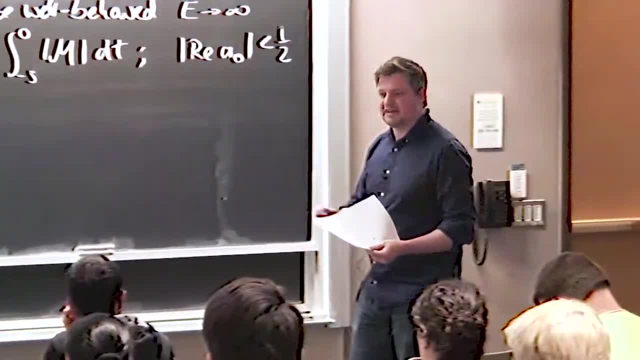 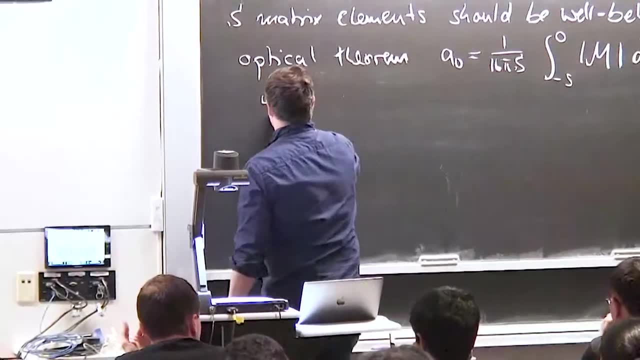 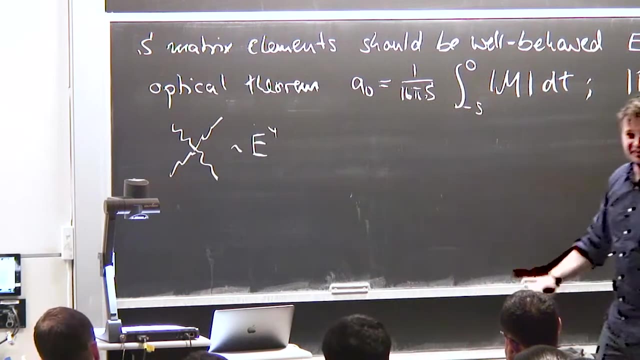 And this is really where gauge invariance but also spontaneous symmetry breaking now go hand in hand. So first of all, we have this term: The scale's proportional to e, to the power of 4.. And this is a calculation that I think every grad student has to do if they are interested in Higgs physics, really. 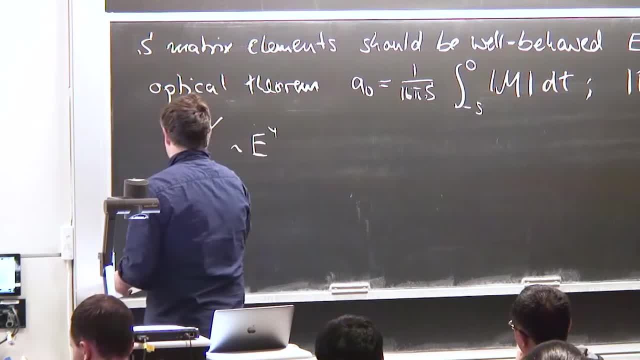 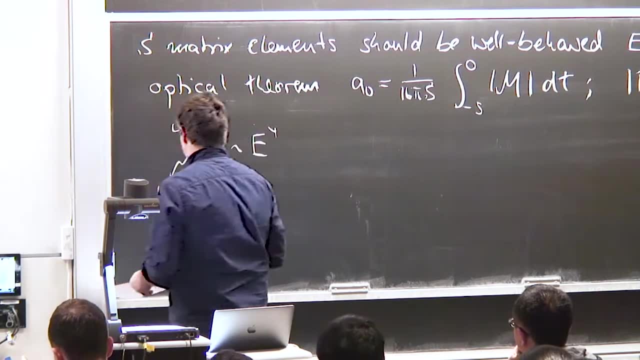 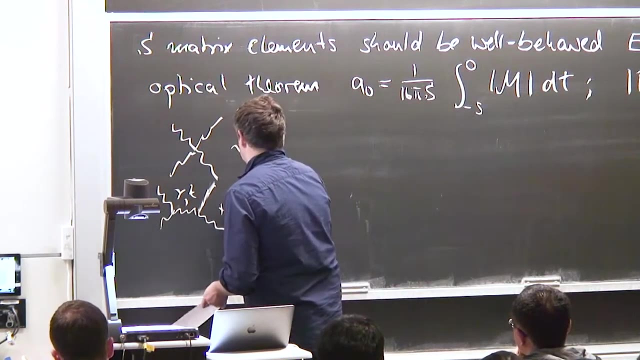 Then of course You have other gauge interactions. But this could be a photon or a Z, And if you evaluate that plus its T-channel partner, then you see this grows with e to the power of 4 as well. So bad. 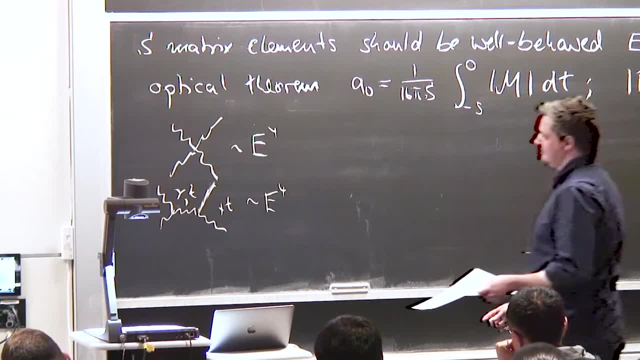 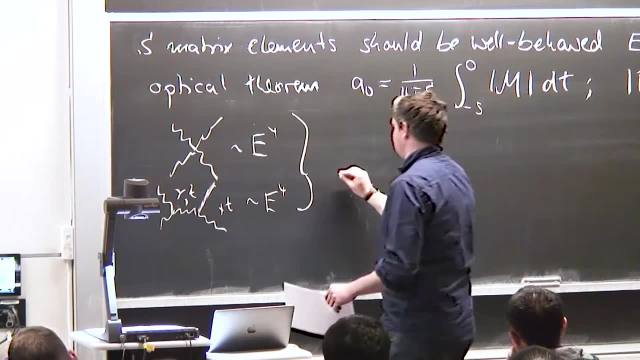 Bad, bad, bad. However, the magic of Gauge invariance. If you sum the two of them, you see that the total overall growth is just proportional to e squared. So why is that? Well, you can do the calculation. 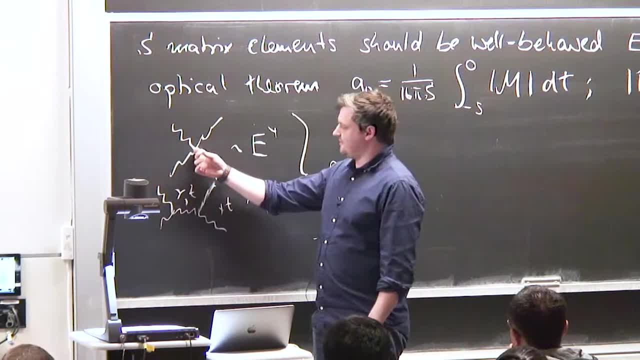 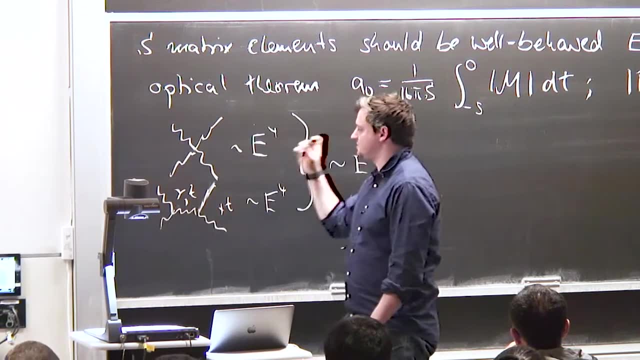 You'll find it out. But essentially this vertex here is just the squared vertex of this times. cosine squared, sine squared. So if you go to large enough energies, the mass suppression here of the Z boson doesn't really matter anymore. Then you have 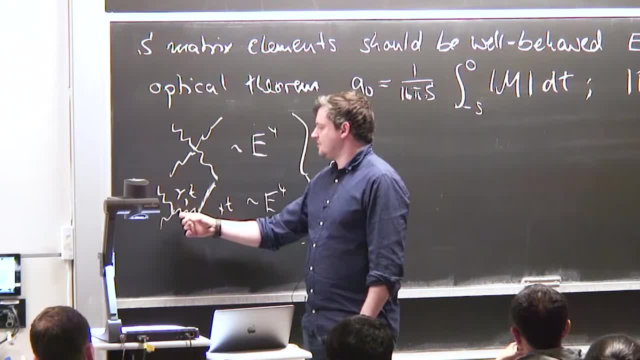 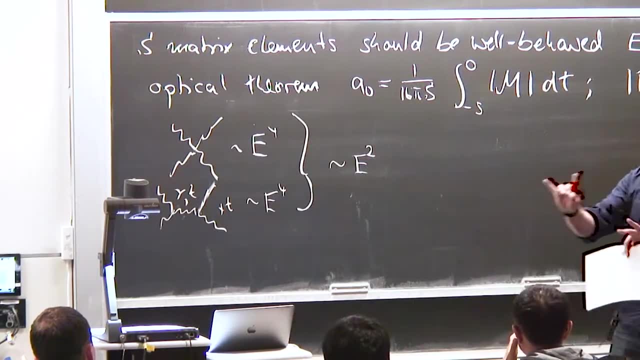 The sine squared or cosine squared if you deal with a photon or a Z, They add up And essentially you deal with the same two copies here of the coupling there, And this is how you sort of merge and only leave you with an e squared growth. 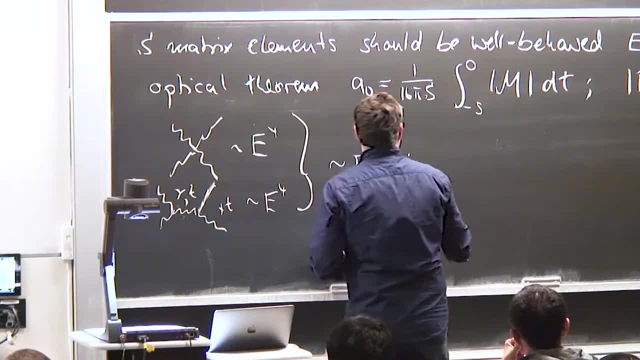 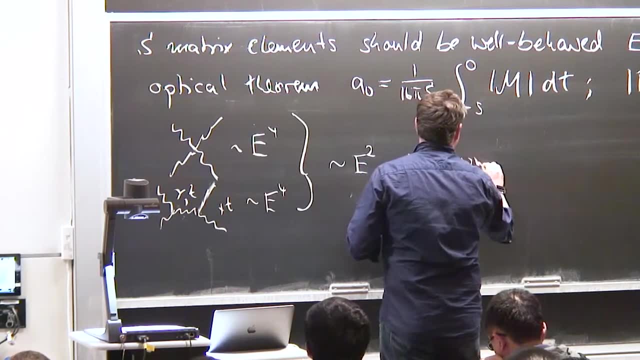 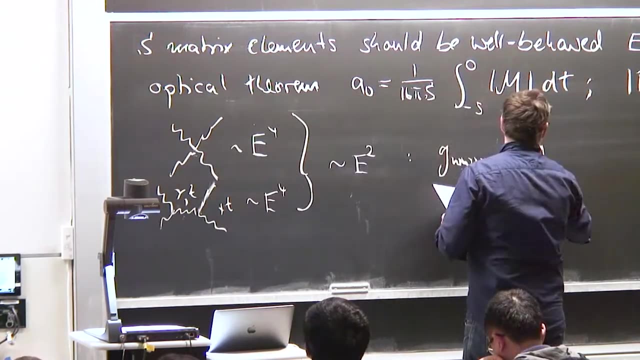 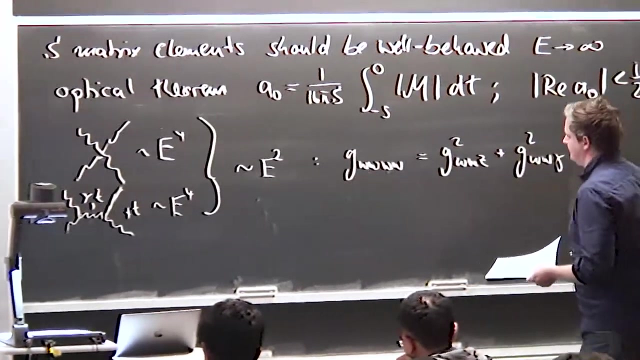 So you can write down a sum rule that guarantees the absence of this e to the power of 4 growth, And this would be the interaction vertex of the 4-point. And the interaction here is g w w z squared plus a, g w w gamma squared. 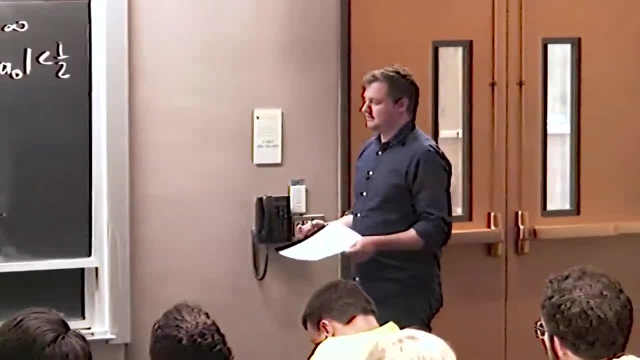 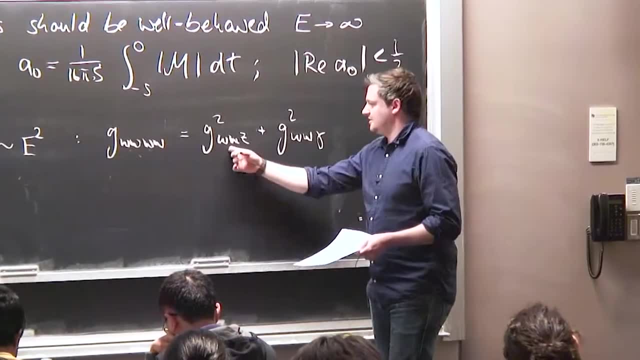 So if you go back and have a look at the quantum field theory textbook, So this is just a g squared. This is a g squared times cosine squared. This is a g squared times sine squared. Sine squared plus cosine squared is equal to 1.. 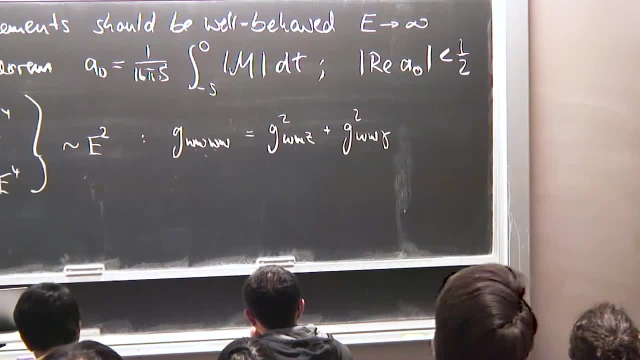 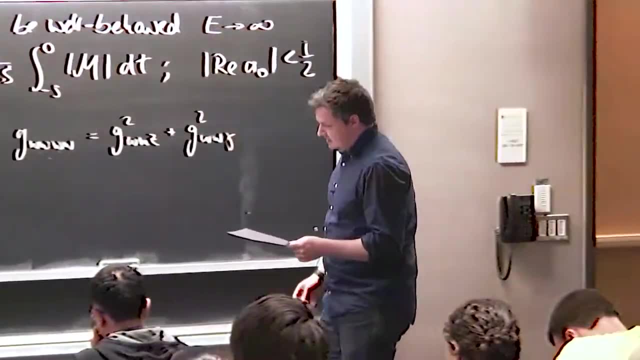 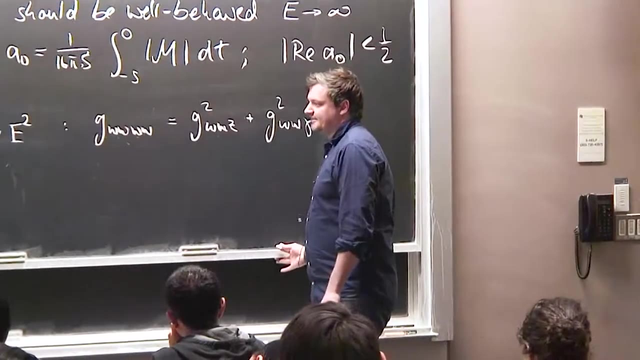 This sum rule is fulfilled just by having a gauge- invariant field theory in the gauge sector, By construction if you wish. But of course we still have to worry about this e squared term. And this is where the Higgs now comes in. 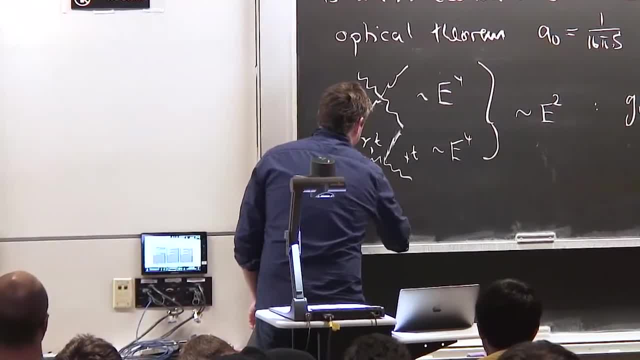 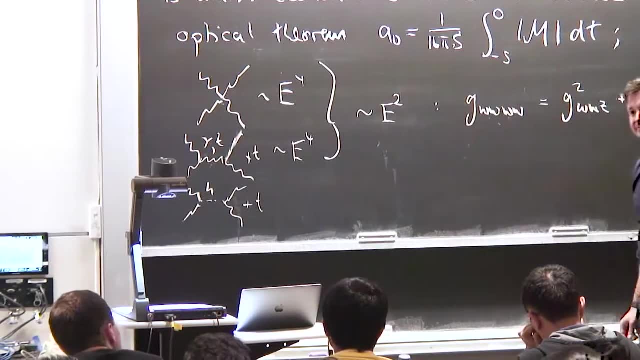 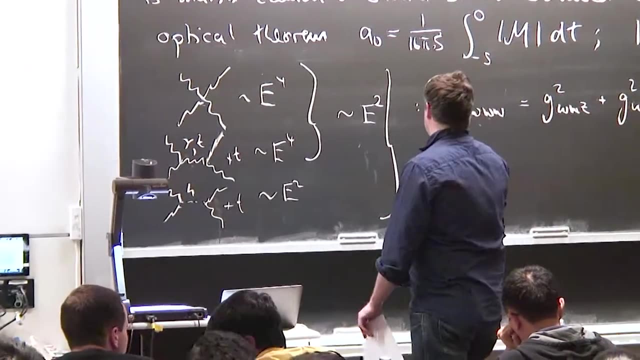 Because we have the Higgs here in the S channel But also in the T channel And I suppress, And if you evaluate that diagram, you'll find that this also scales with e squared And in such a way that these add up to e, to the power of 0 in the high energy limit. 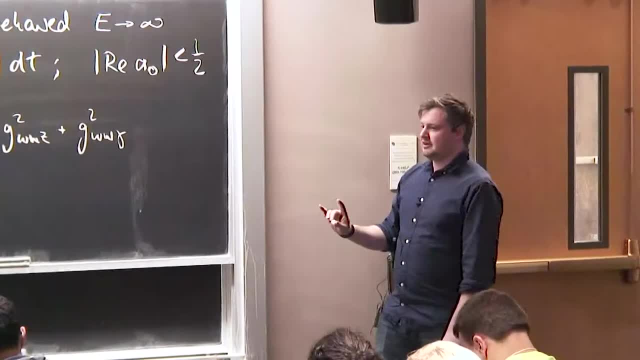 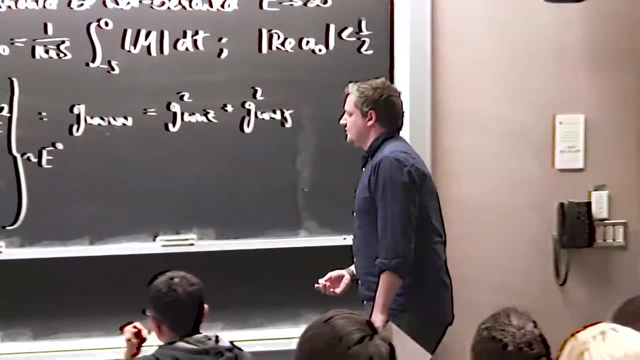 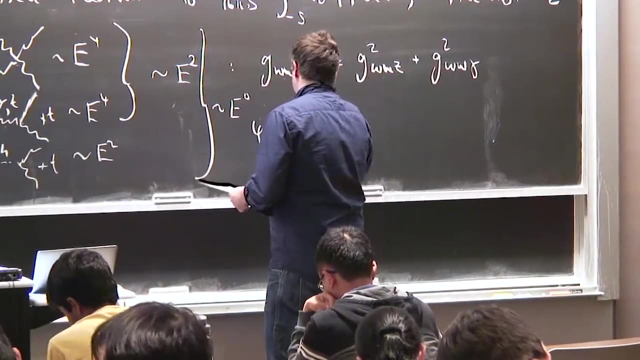 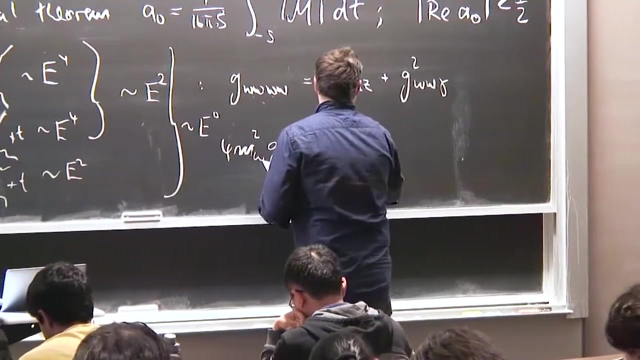 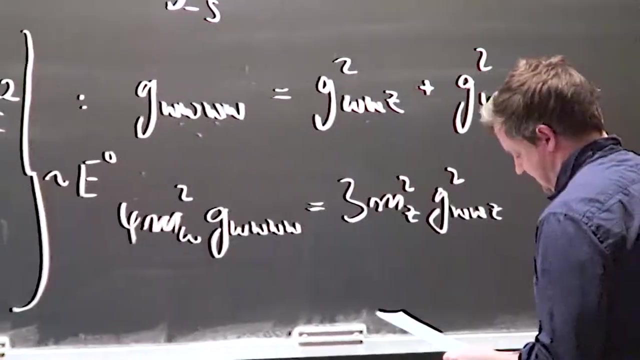 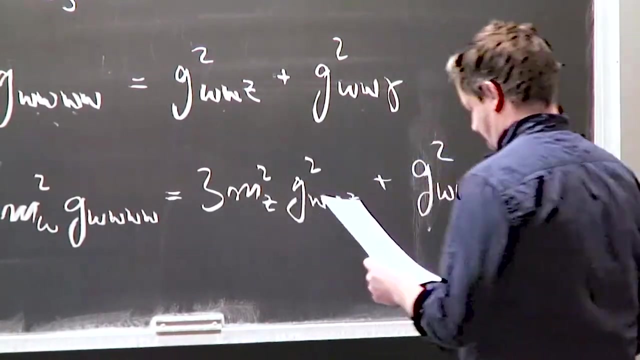 And high energy limit means that we are looking at energies or center of mass energies much higher than particle thresholds here, And the associated sum rule that you can find for that would be 4 times m w squared times. the vertex is equal to 3 m z squared, g w w z squared, plus g w w h squared. 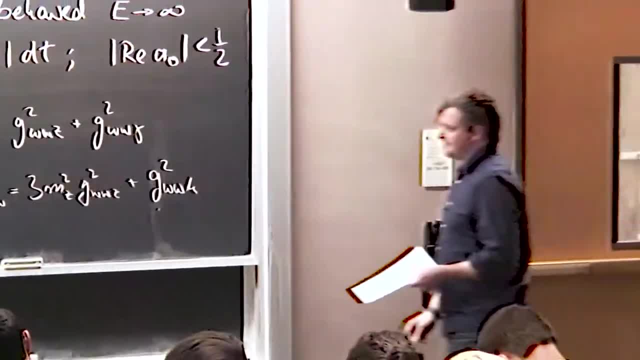 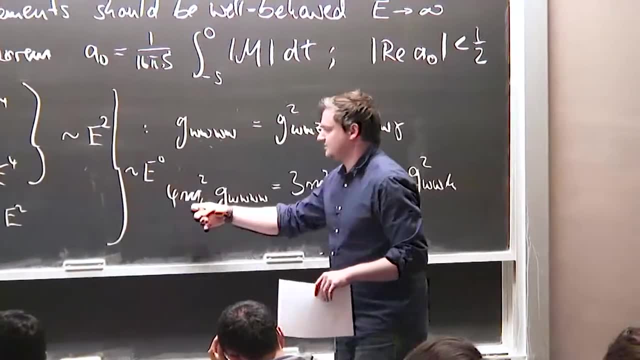 Okay, So you can see that there is a nice sort of geometric understanding Of this sum rule. So you deal with 4 w's And the quality coupling, The w mass, is m w squared. You have 3 polarization states of the z. 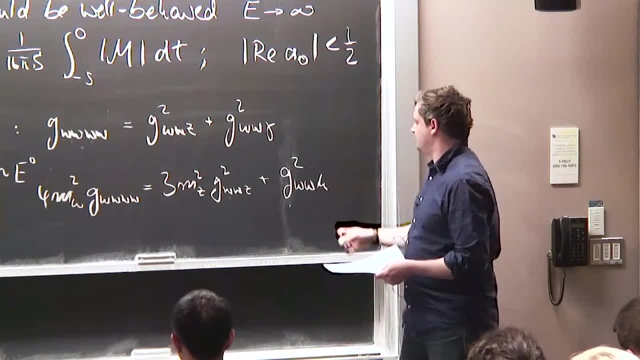 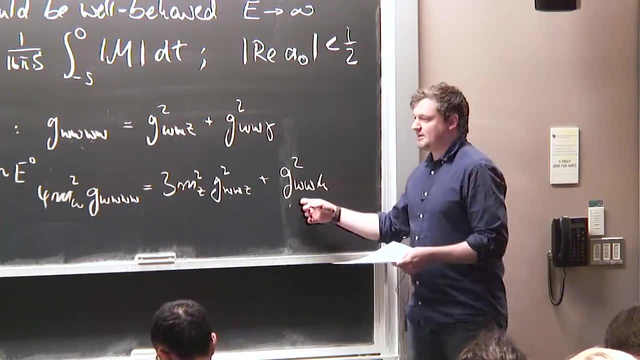 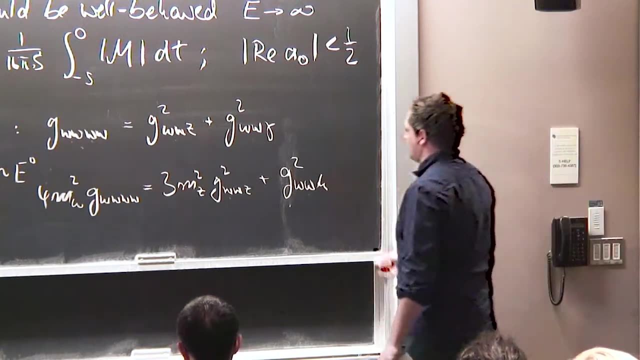 That get mediated here. W w, z coupling. You have no mass for the photon So it doesn't appear here. But g w, w h is just related to the w mass generation. So you get a g times m w essentially. So all of these things add up. 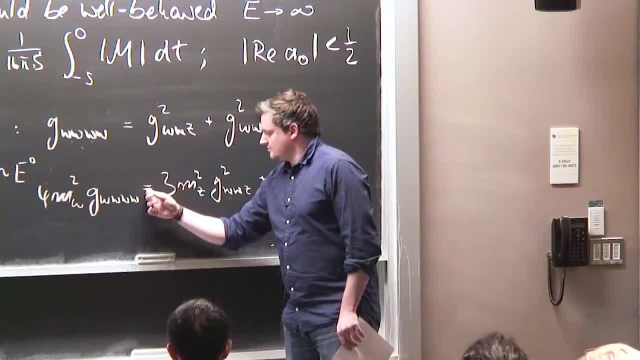 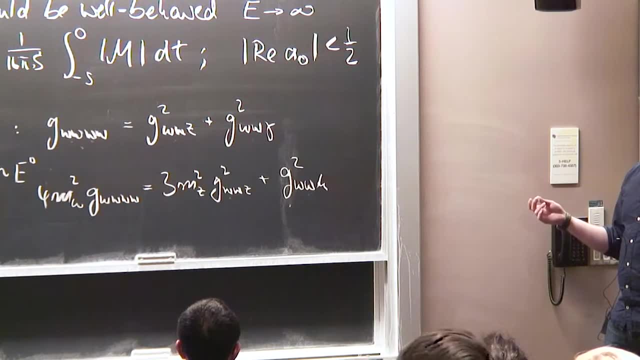 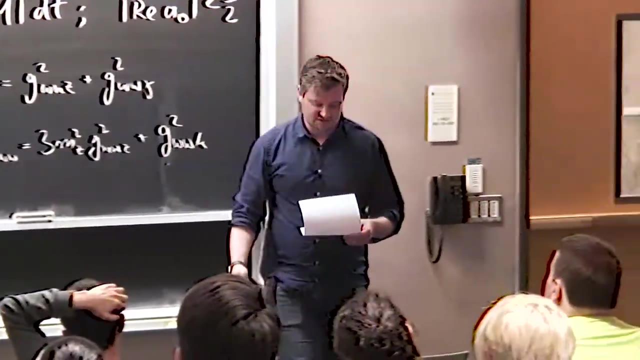 And this sum rule is enforced through exactly that mass relation. That m w squared divided by m z squared is the cosine squared of the Weinberg angle. Okay, So this is very sensitive to the tree level way How you generate gauge boson masses with the doublet width. 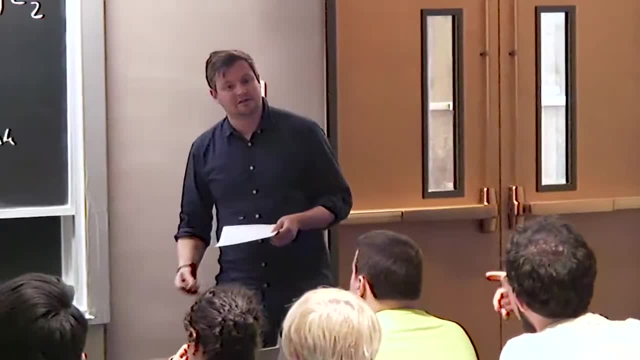 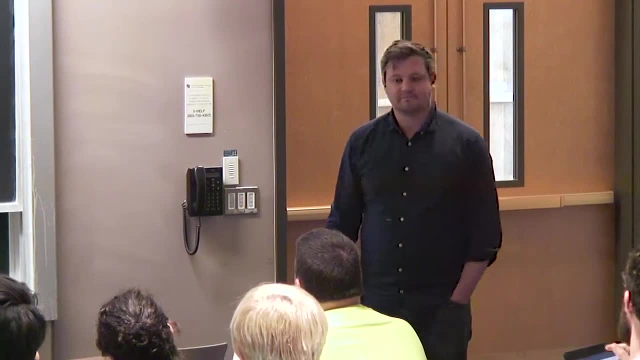 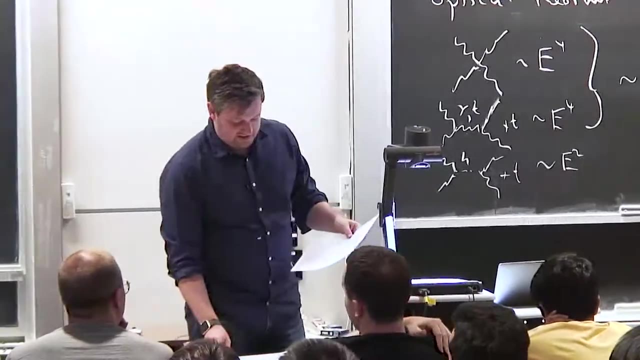 Yep, So I think you might have just answered it, But like we were talking about the mass relation before, That only works with the g's and the 2. So does this also Like? do these sum rules also? No, So that's just an implication of spontaneous symmetry breaking itself. 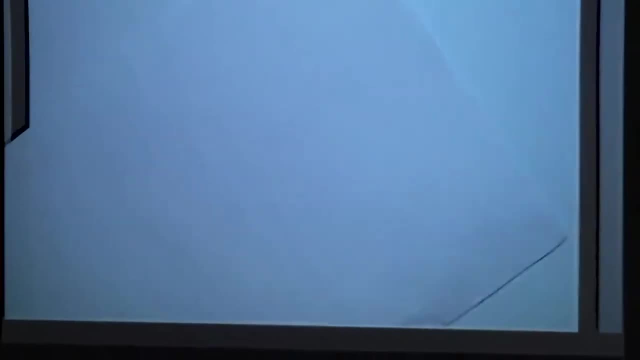 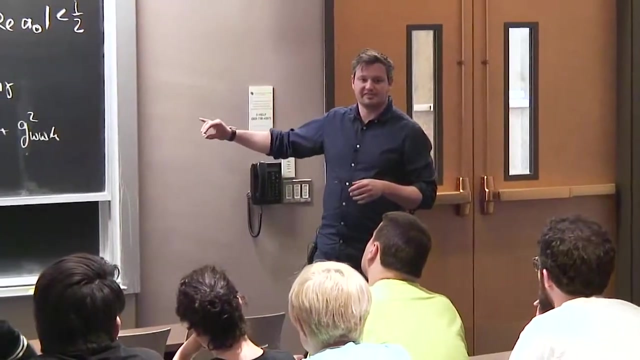 Which means that if you were to break electroweak symmetry with triplets, You would get identical Some rules. that would look different though. So this is the whole idea that Combeau, Levin and Tektopoulos took in the 70s. 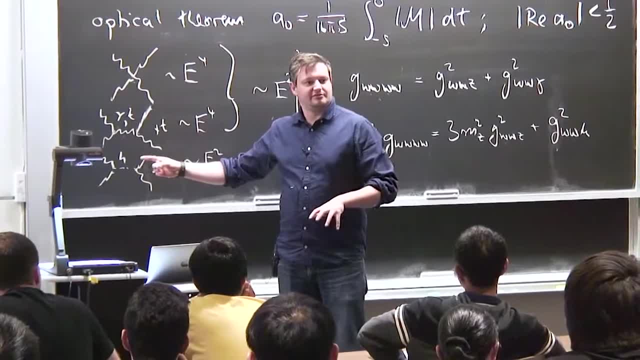 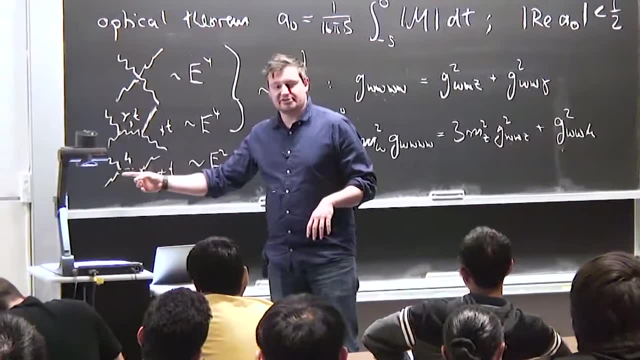 Right down this amplitude And then you try to sort of reverse engineer what the couplings might be here And you can see there is no choice Other than that the Higgs coupling to the 2 w's is exactly like that. It's exactly like g times m, w. 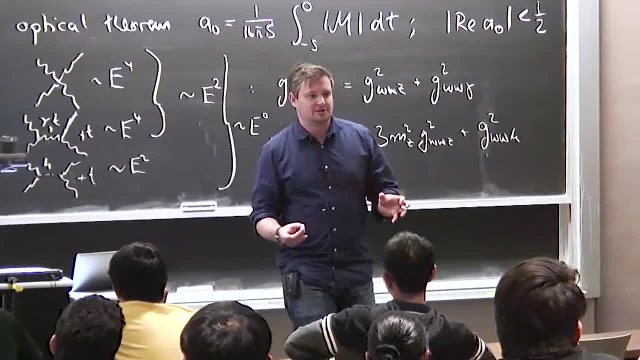 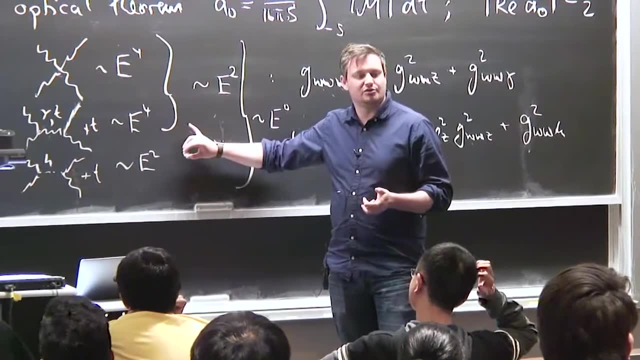 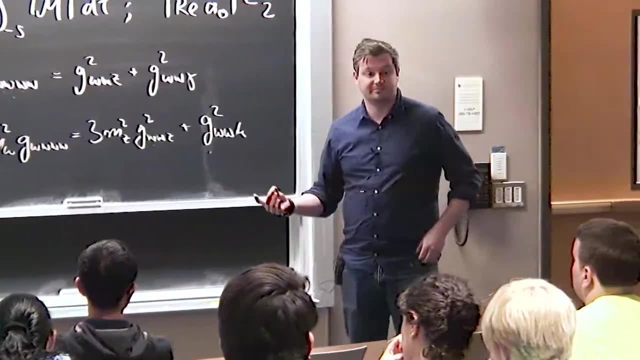 And that you can only create through spontaneous symmetry breaking. So this is sort of you know In a hand way, the argument proves that this is something particular to spontaneous symmetry breaking, But not constrained by how you break electroweak symmetry. So if you dealt with a triplet, 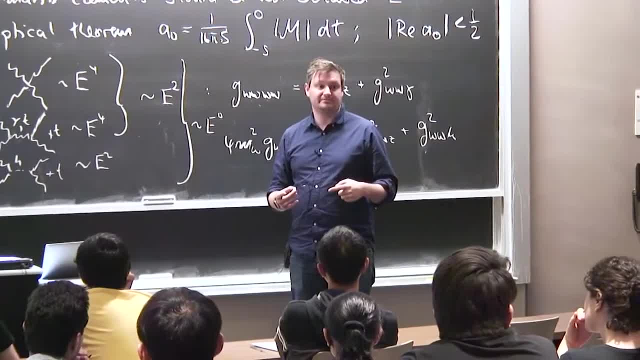 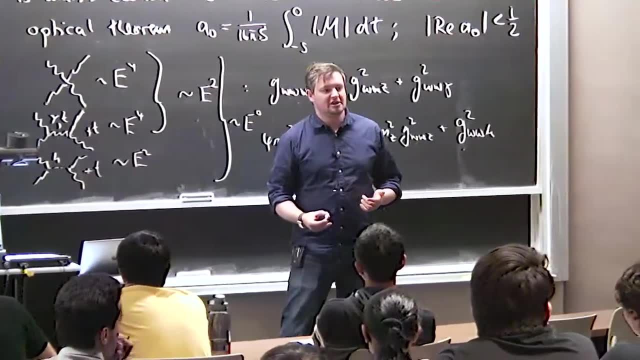 You would have same sum w scattering Right, And that does not appear in the standard model- Well, through photons and stuff, Okay. But then you get doubly charged Higgs's in the S channel, And then of course, you get new sum rules. 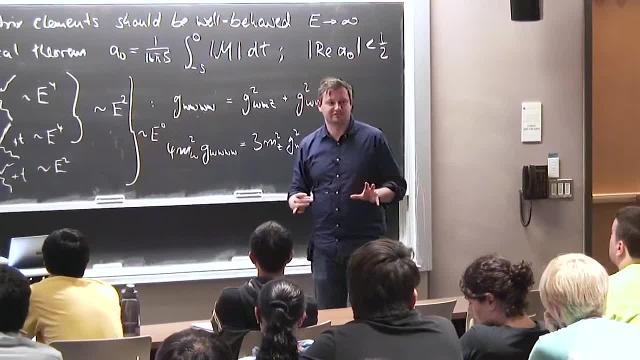 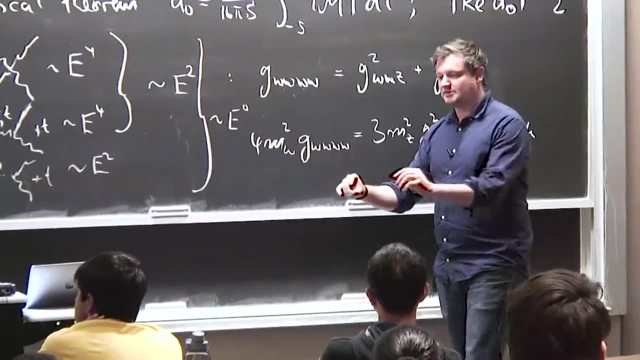 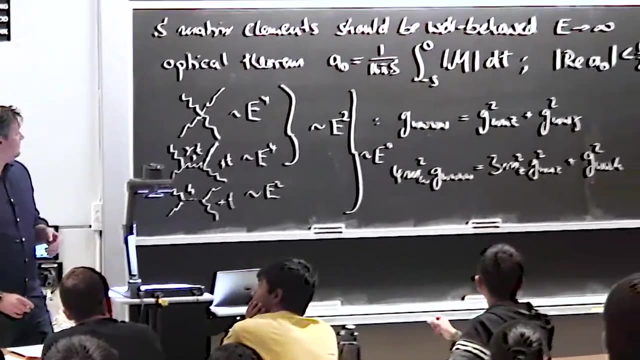 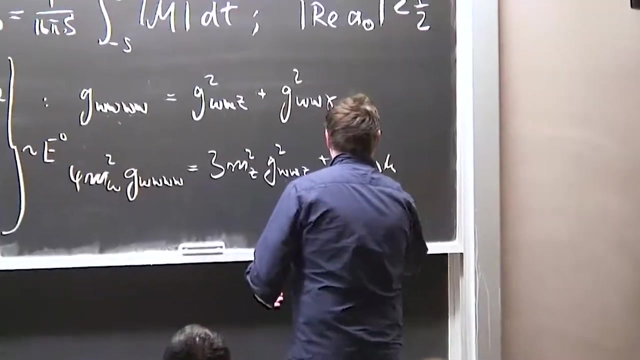 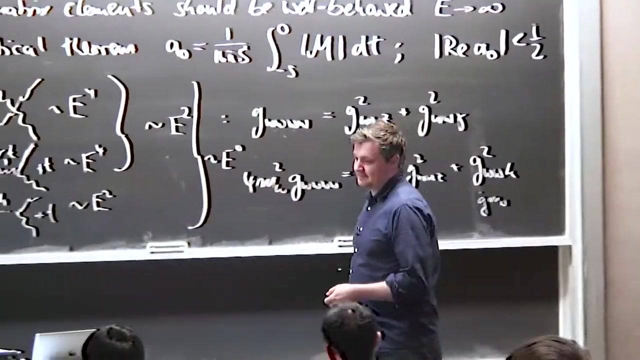 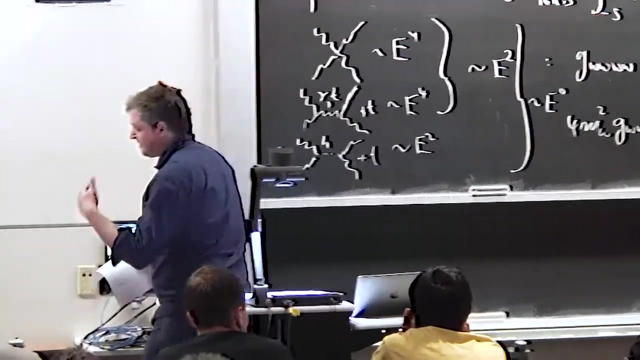 And you know the way this is implemented becomes non-trivial. But irrespective of how you do this, You always end up with a good high energy behavior. Sorry. So this guy is proportional to g times. m w Right. So from this we see: 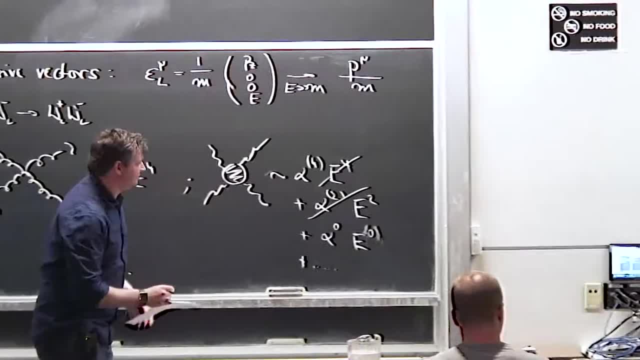 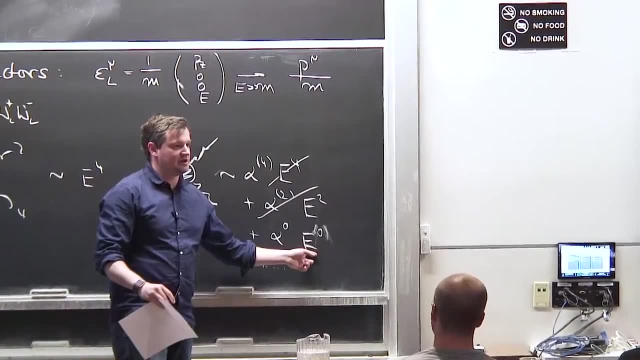 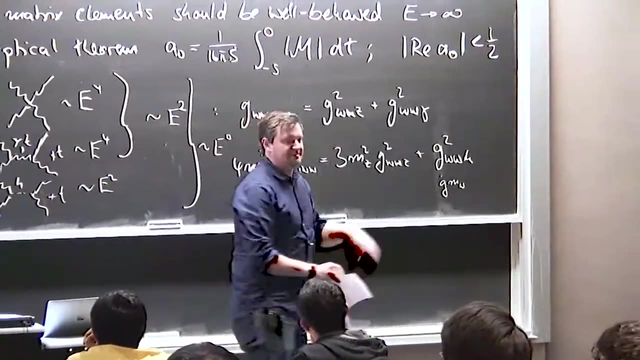 This term is gone. This term is gone. So the only thing that's left is Is e to the power of zero In the Taylor expansion. So that's, That's okay. You know this will not violate The perturbative unitarity bound on a zero partial wave unitarity. 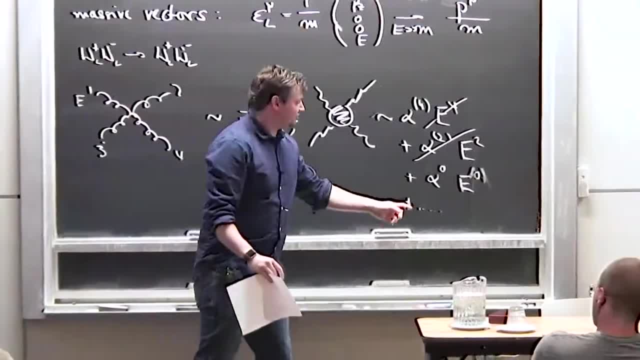 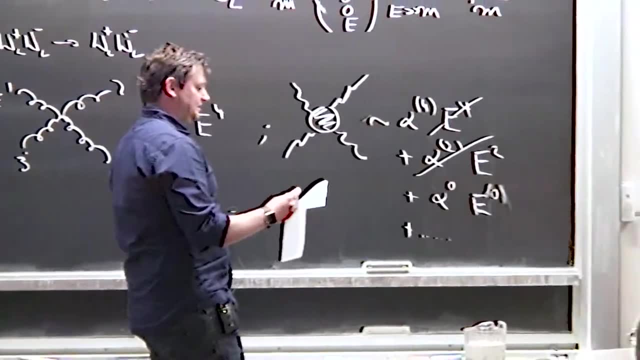 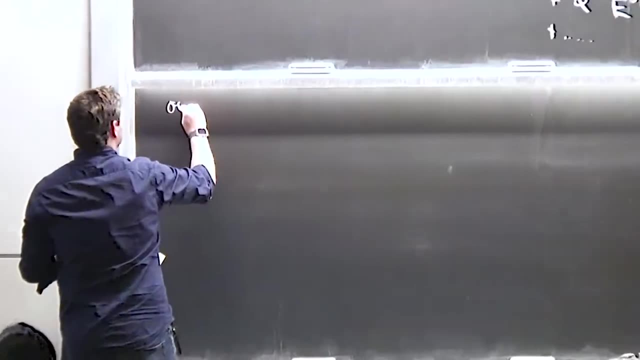 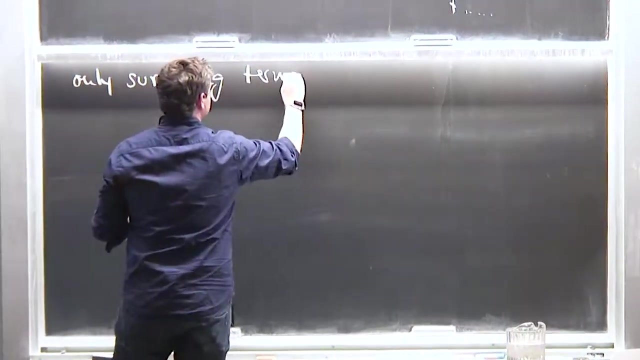 But in principle you could Argue that maybe this alpha naught Is so large That this one divided by two Actually gets saturated, And then you're in In the pickles again. So the only term that survives here Is this alpha naught. 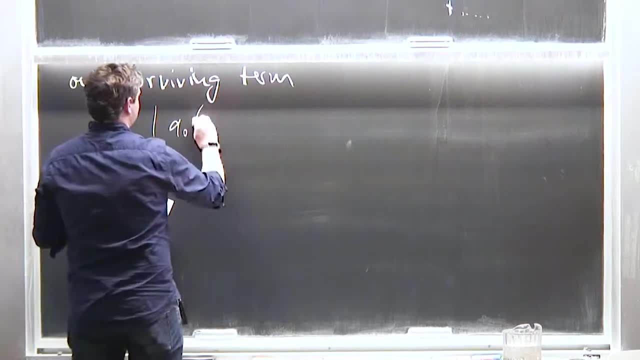 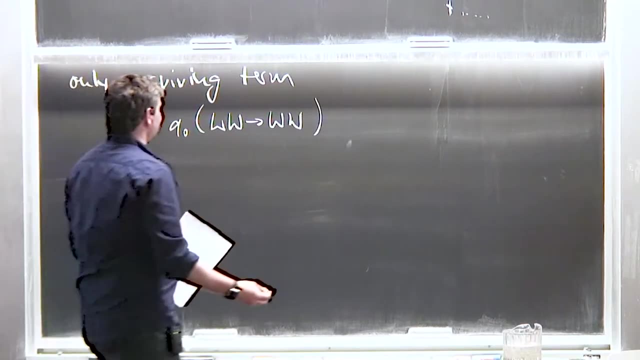 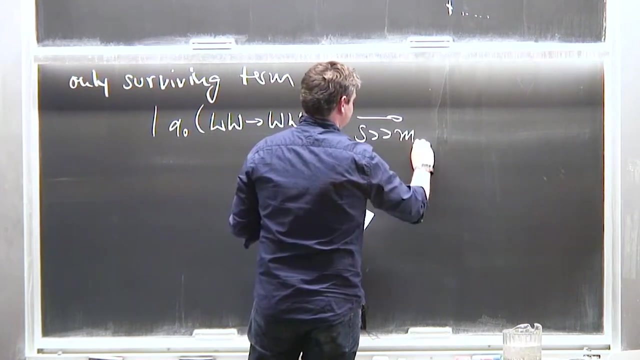 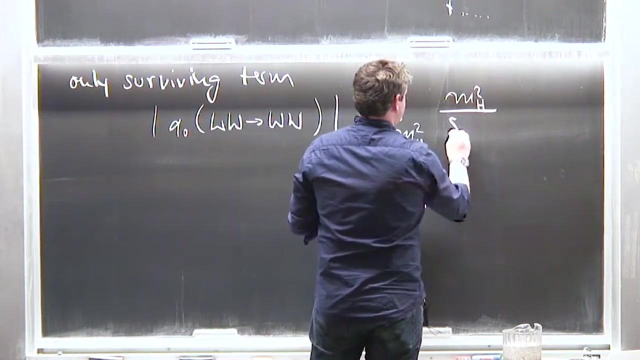 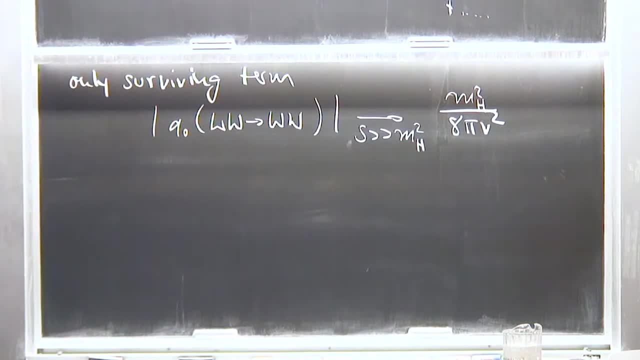 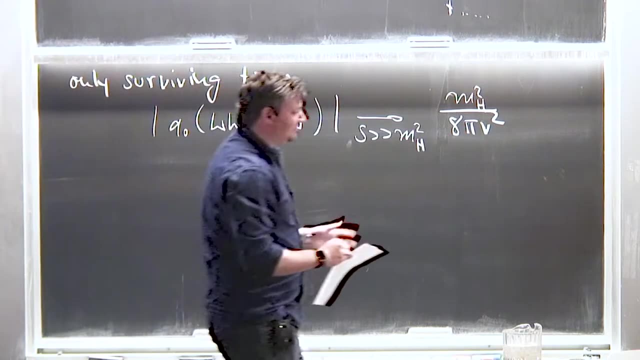 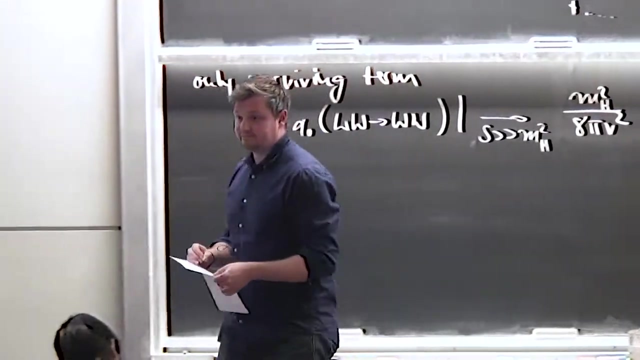 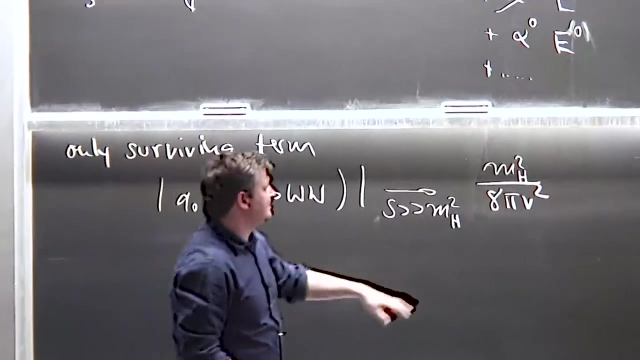 squared. so if the Higgs mass is too big, then you break unitarity. well, you don't really break unitarity, but what this tells you is that higher order corrections become relevant, and they become relevant in such a way that the next leading order electric corrections, which sort of meant exactly this growth. 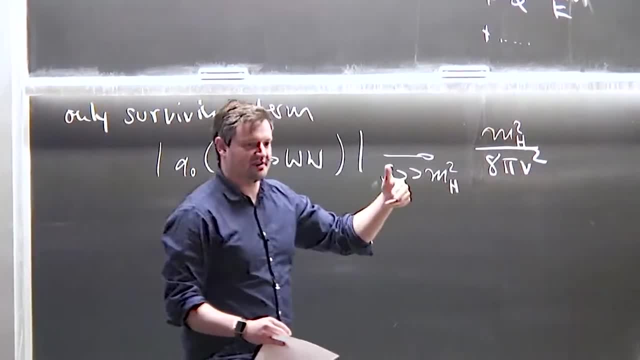 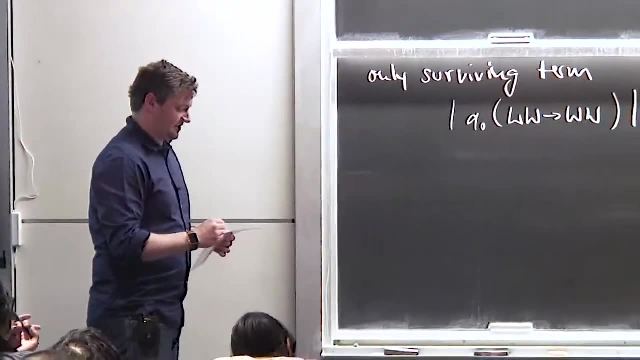 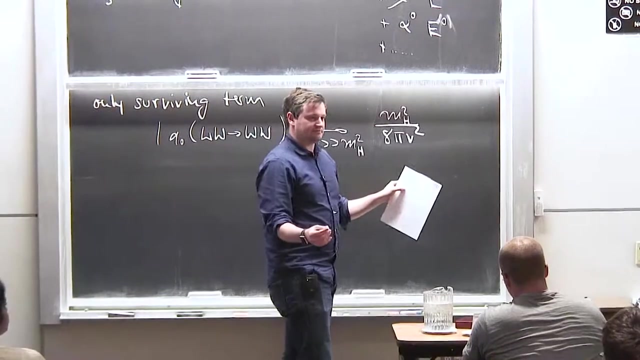 so each order of perturbation theory will become naively of the same order. so you start actually pushing into the strongly interacting limit of your electric sector. so you, if perturbation theory is a, is a good thing, and if nature chooses to live in a in the region of parameter space, where, where it admits the application of 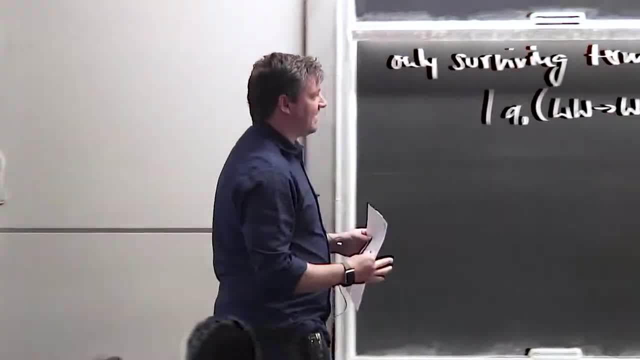 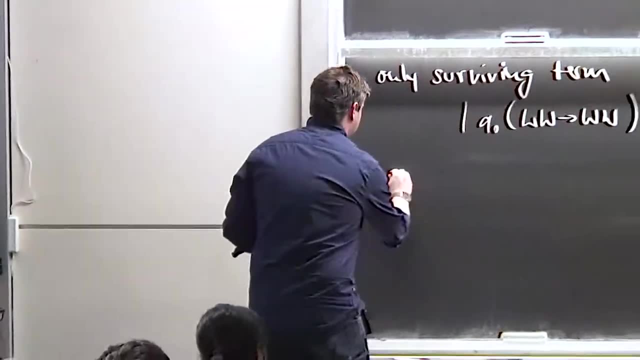 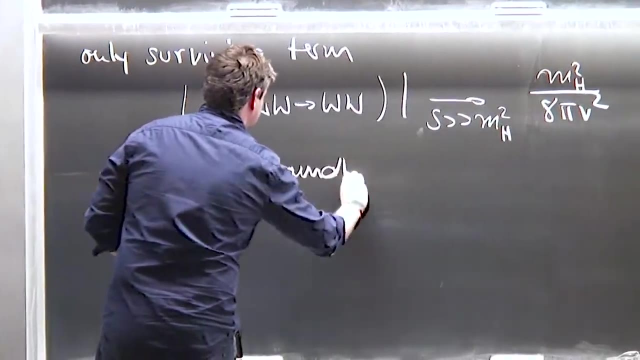 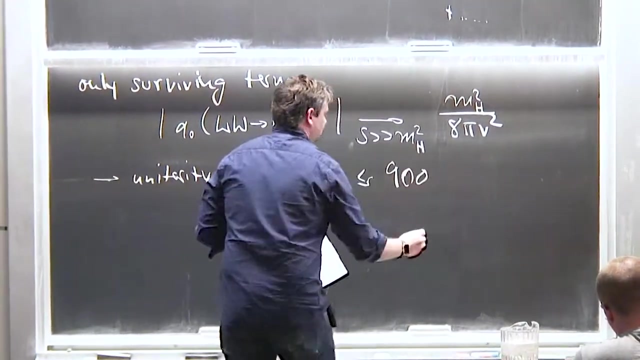 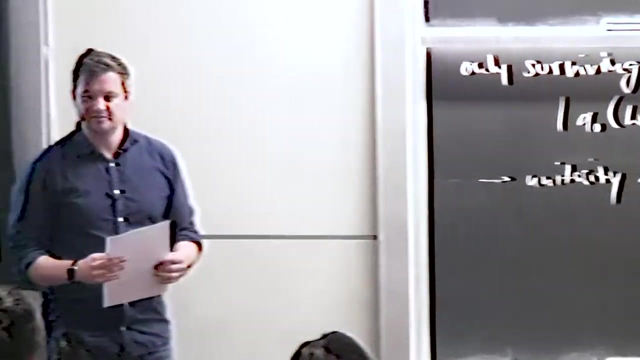 perturbation theory, then something has to happen before this constraint gets saturated by the Higgs mass. okay, and this is called the unitarity bound, which limits MH to be lighted in roughly 900 GeV. there are other processes, that it's not only WW scattering, is also w zed scattering and so on, so forth. so in principle you 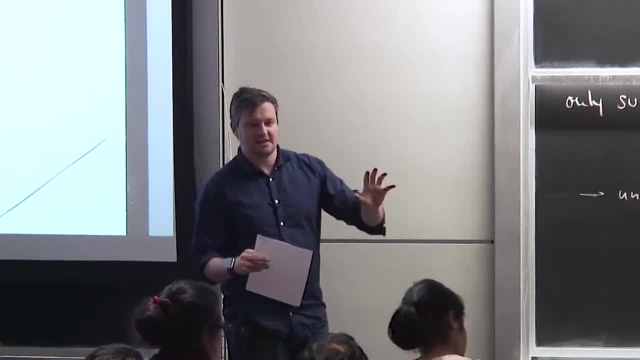 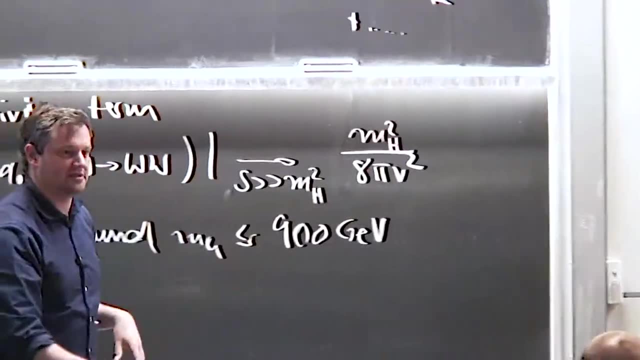 have to look at all these scattering processes and then take the maximally constraining one. okay, so in this space of longitudinal gauge Poisson scattering amplitudes and limit gauge Poisson space amplitudes, that's. this is just to show you that that's. 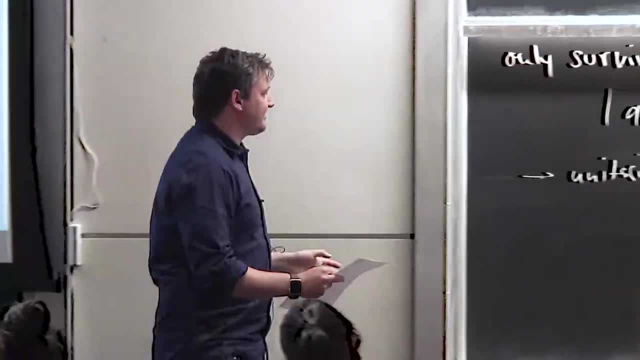 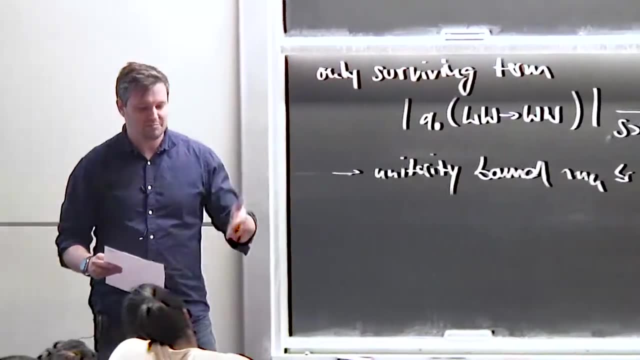 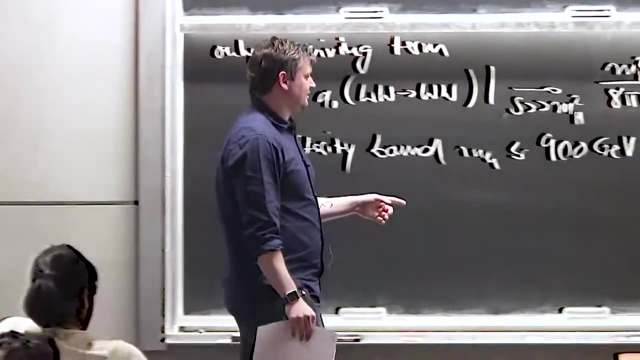 And you now can see that there is actually not really a coincidence that all these Higgs exclusion bounds that you see, start at 114 or so. This is where LEP lost its sensitivity, And they go up to 1 TeV. This is exactly where perturbation theory breaks down. 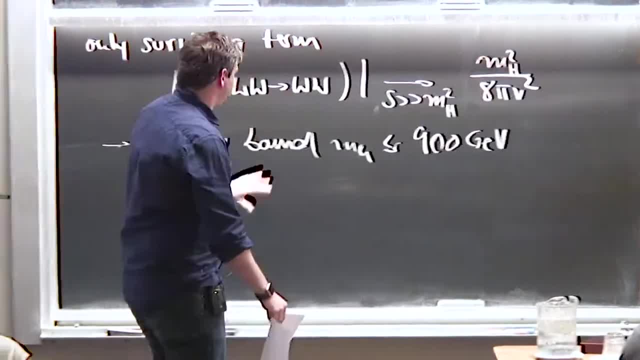 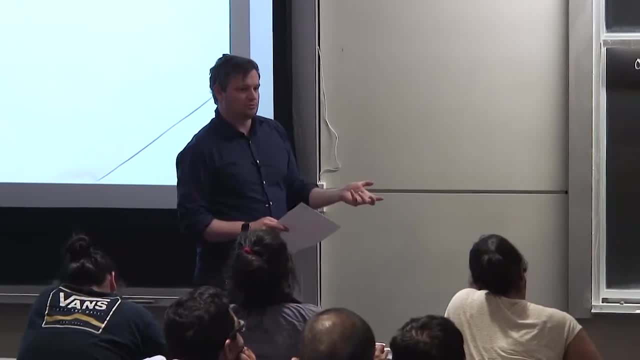 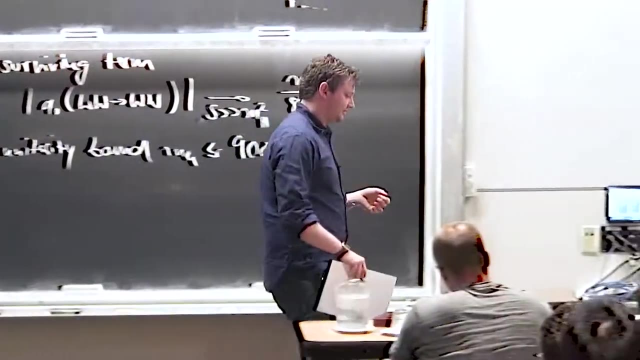 and you would see some strongly interacting sector, And this is really the motivation behind the LHC being a no-loose experiment, because we knew the Higgs is either there or we find something else, And we find something else, for instance, so something that was quite fashionable when I went to grad school. 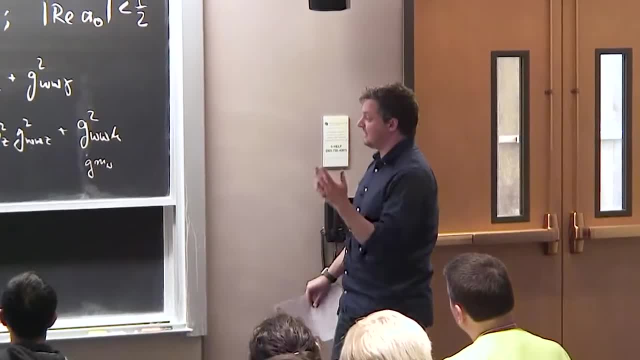 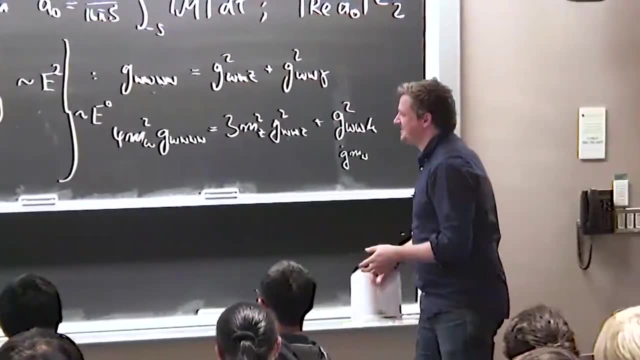 were models of extra dimensions. So my name is Englert and I worked on Higgs-less models during my master's, So people find that funny and it is funny. So essentially what you can do is you can throw away this guy here entirely. 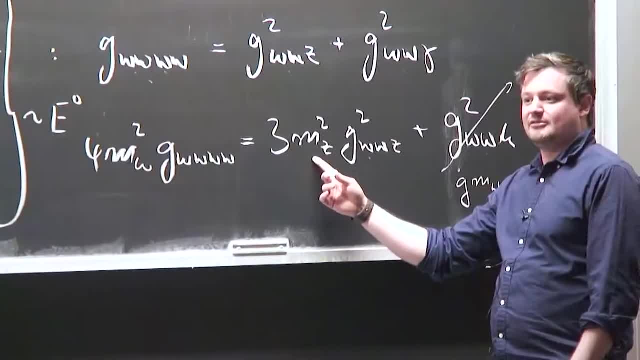 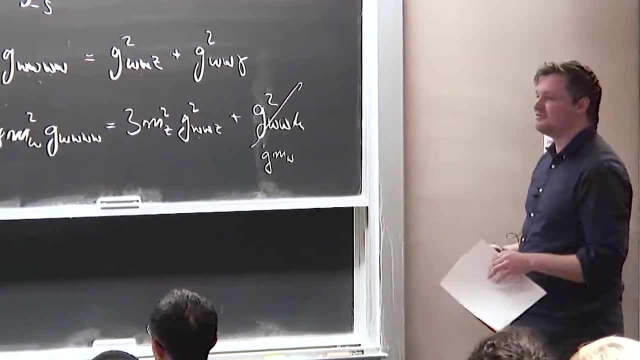 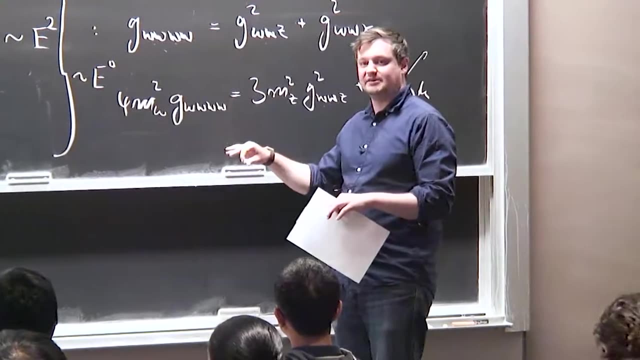 And replace it with copies of gauge bosons of type spin 1. And you can write this down as a 5-dimensional ADS-CFT-inspired theory. And then you get tight constraints on where these extra vector resonance should sit. You can think of it as strongly interacting, Higgs-less scenarios. 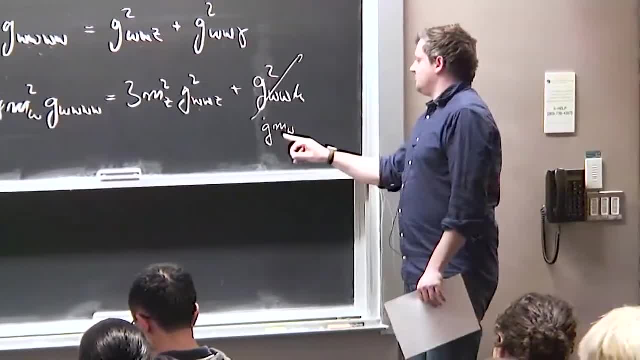 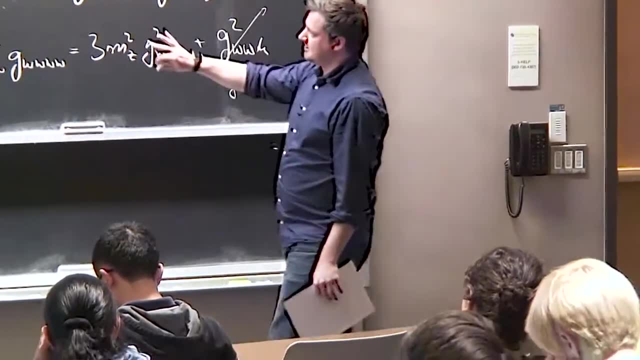 You can bring the Higgs back in, So you can dial away part of electro-heximetry, breaking from the Higgs into strongly into a strongly interacting sector, for instance. So you can take these sum rules and really play with them phenomenologically. 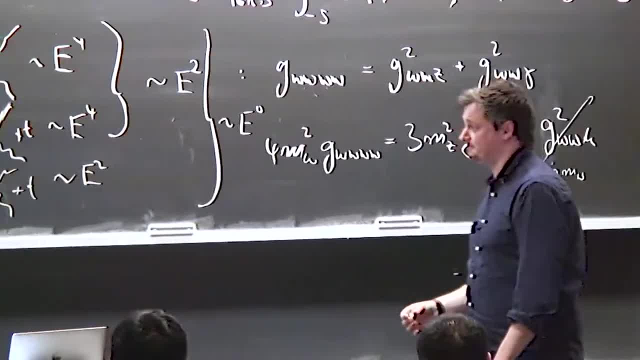 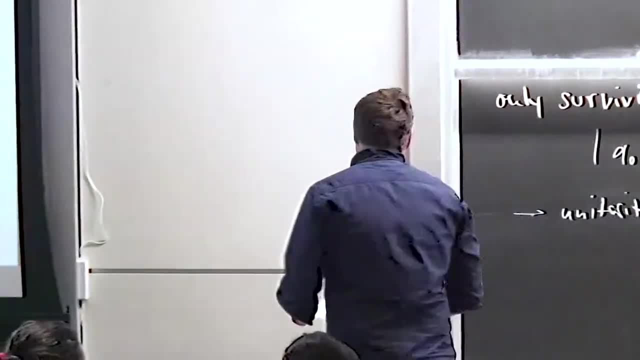 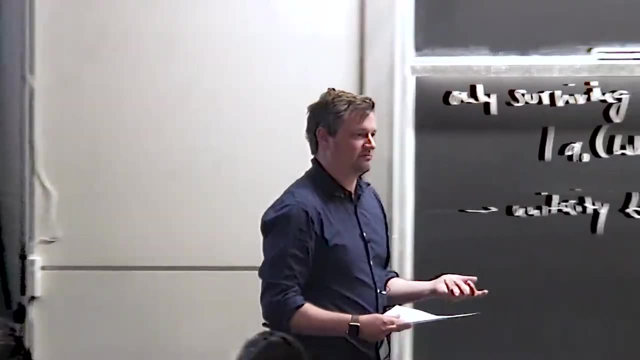 In a sense that you can predict where new stuff sits. So the LHC really was a no-loose experiment in that sense. But you also can see that this unitarity stuff is really a major motivation of beyond the standard model Higgs searches. 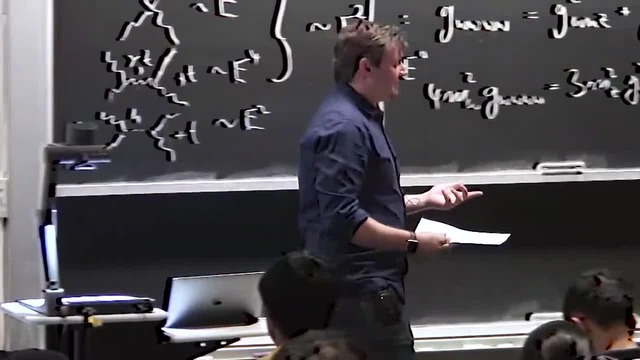 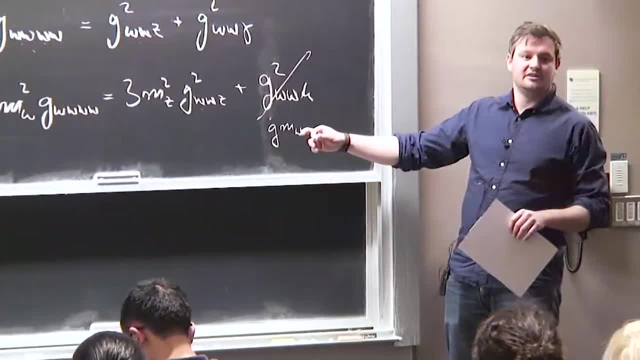 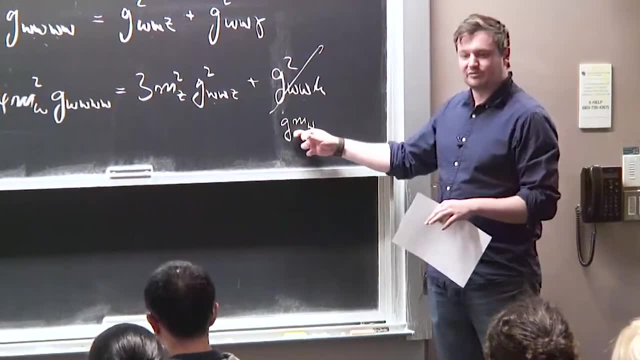 Higgs searches. So if we measure, say, a deviation of 10% here of the Higgs coupling to the Ws relative to the standard model, so if that deviates from this value, Then we are, you know, back to square one. 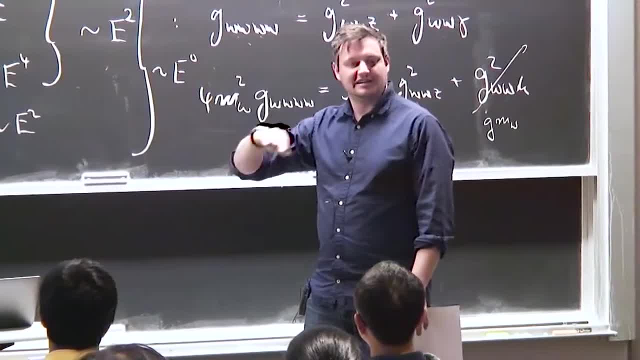 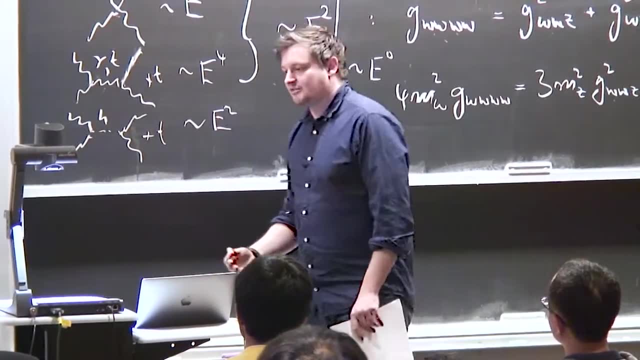 Which means that at high scales, we get unitarity violation, And they can only be circumvented if new degrees of freedom pop up that exactly compensate for this effect. Now, So you? This gives a very, very strong argument to look. 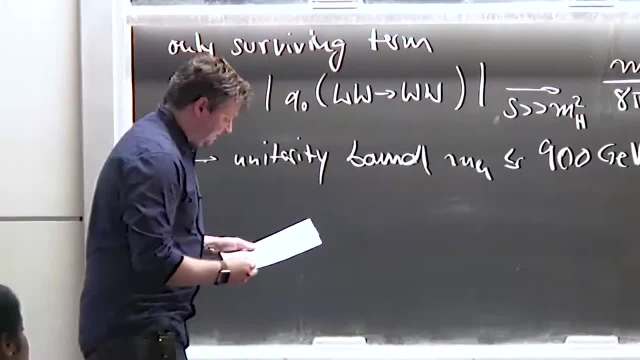 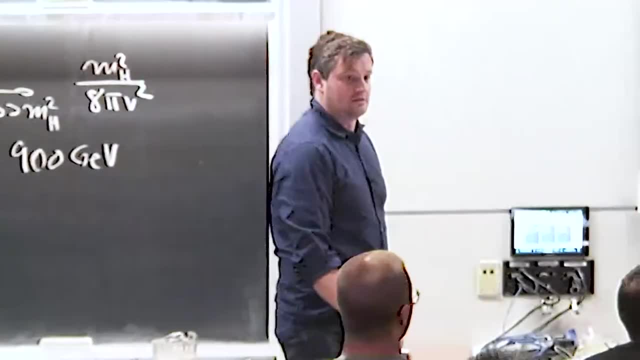 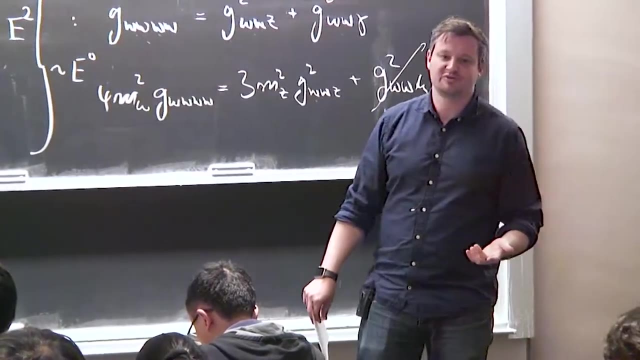 into very specific processes at the LHC, and we'll discuss this later on. Yeah, Do they have the same problem? The same problem: Yes and no, because five-dimensional theories are intrinsically non-renormalizable, so they always come with a cut-off. 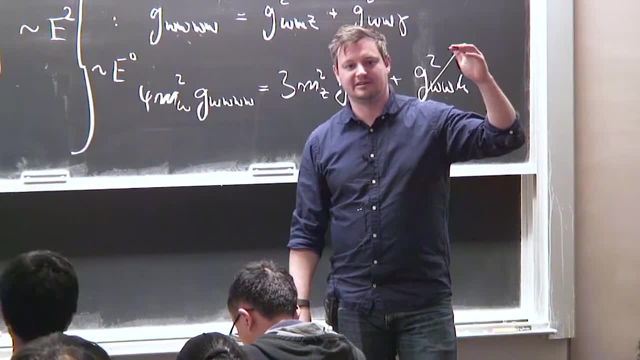 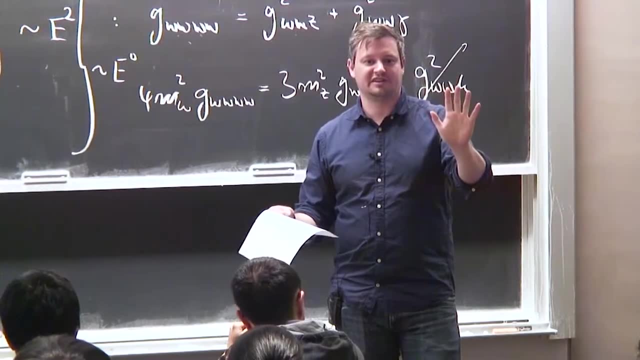 So you get this entire Kaluza-Klein tower of states and if you look at the heaviest one, then by definition they would get a unitarity violation, because you don't know really what lies beyond that cut-off. The cut-off is played by the UV brain. 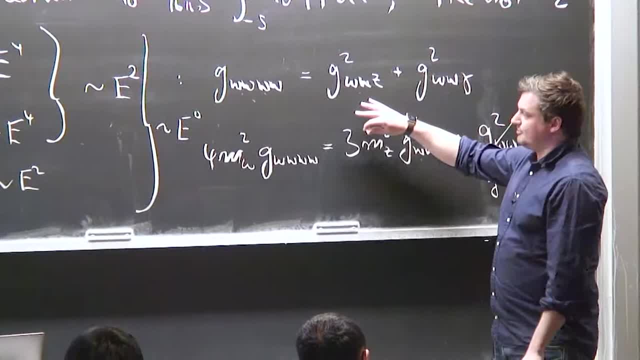 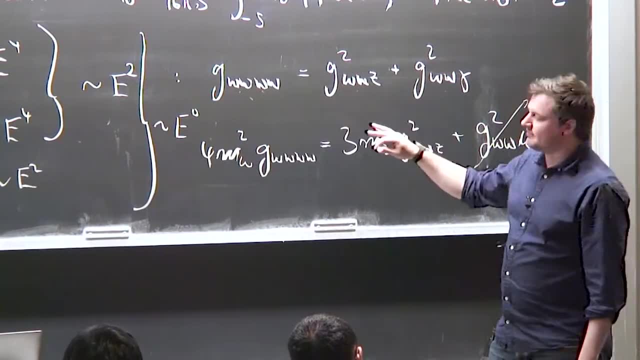 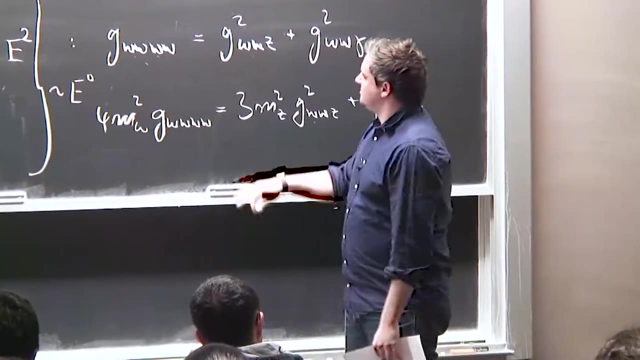 The source of these things- and there's actually a nice, if you're interested really in 5D theories, for instance, or ADD scenarios as well- the source of this is completeness relations of wave functions in the fifth dimension. So it's essentially a completeness relation. you know Fourier modes, if you wish. 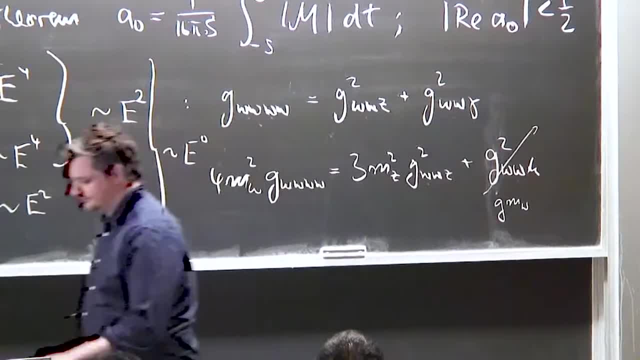 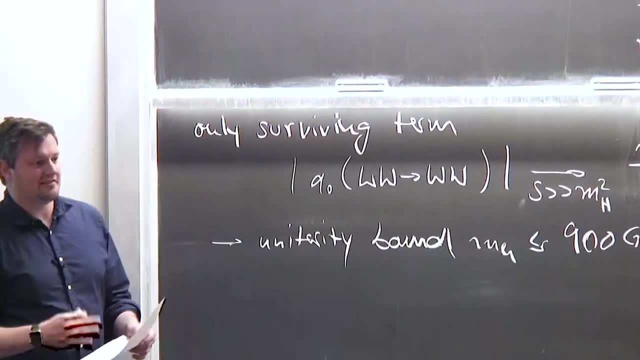 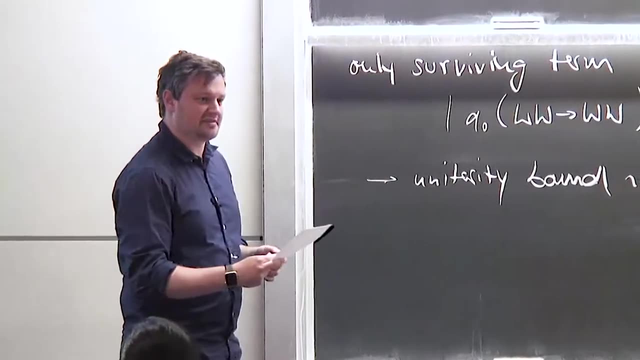 And this is how you prove this as well. So any modification of Higgs couplings, though, away from the standard model value, will tell us that something else has to be there, And this is why people are very, very concerned about getting the precision of these Higgs couplings nailed down. 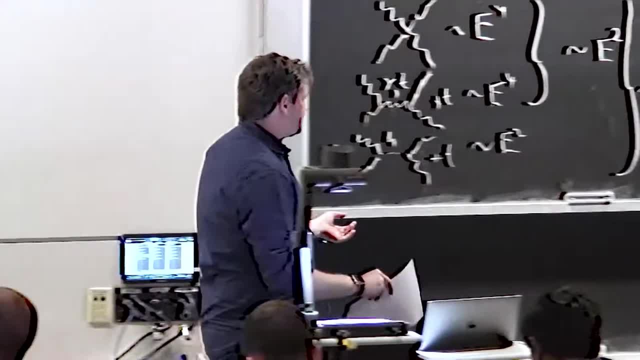 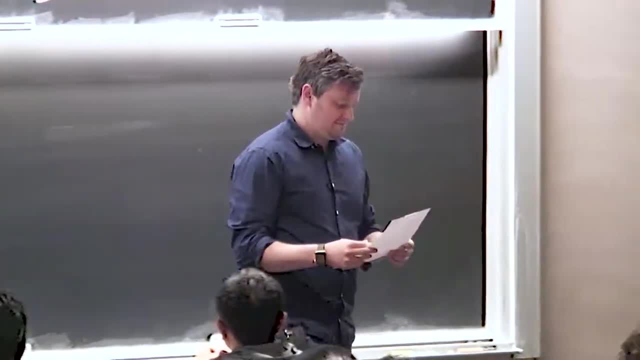 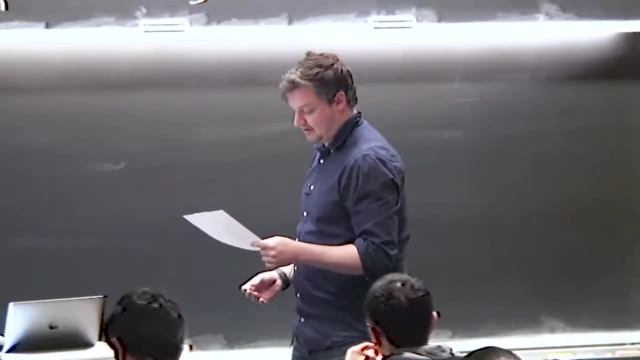 So let's have a look at one example where this actually takes place, And Jim already discussed this singlet mixing. This is a Higgs portal sort of scenario, and this is quite nice to have a look at this in this context as well. 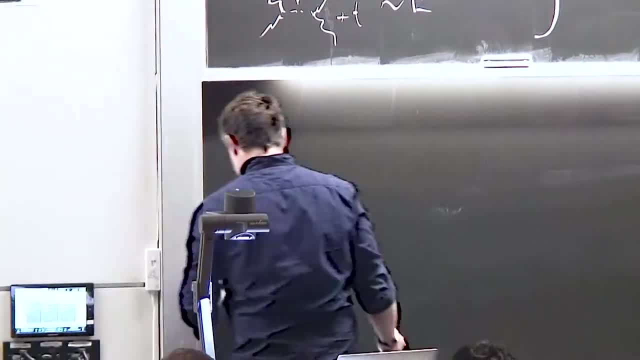 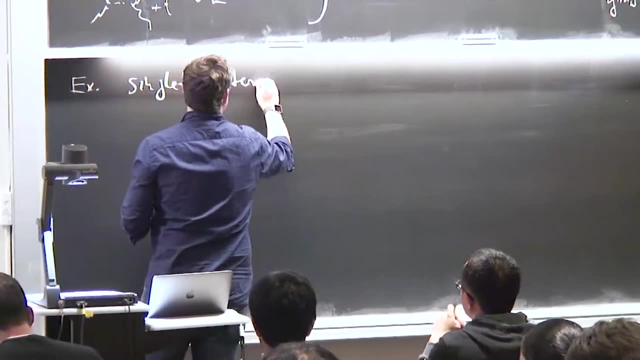 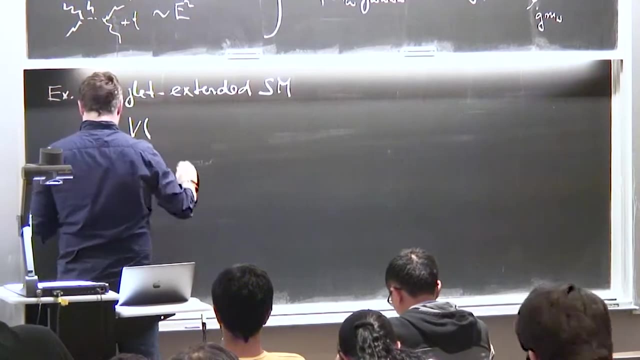 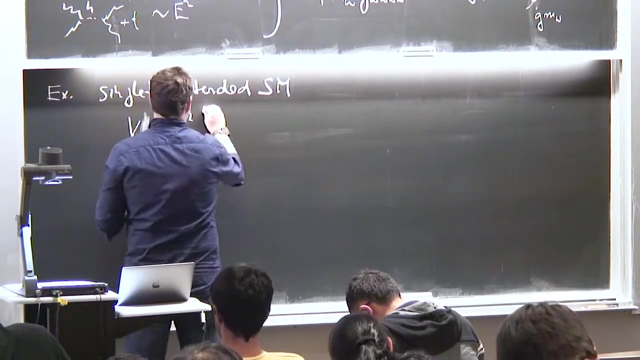 So, as an example, we have the singlet extended standard model And you can write down a potential that depends now not only on the Higgs sector but also on the Higgs potential. So if you want some hidden sectors, you can take a mu s squared, phi s squared for the visible stuff. 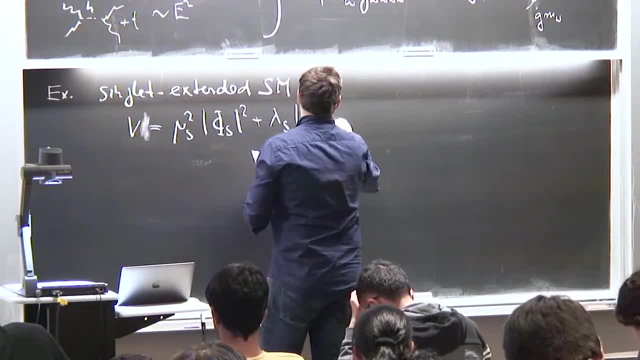 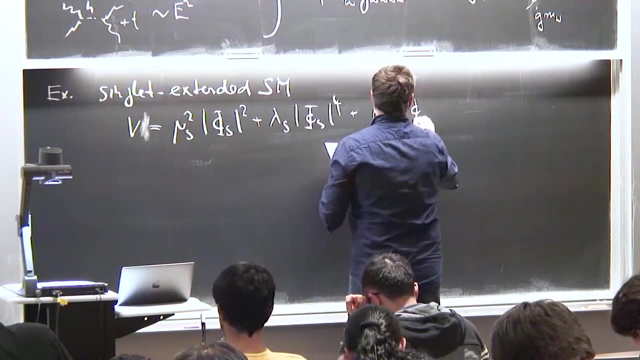 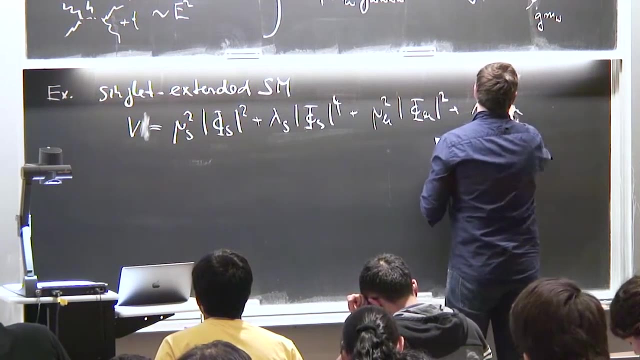 plus a lambda s phi s to the power of 4.. And you have the same thing mirrored in the hidden sector: mu squared phi h squared, plus a lambda phi h to the power of 4.. And because the squared of these guys are singlets. 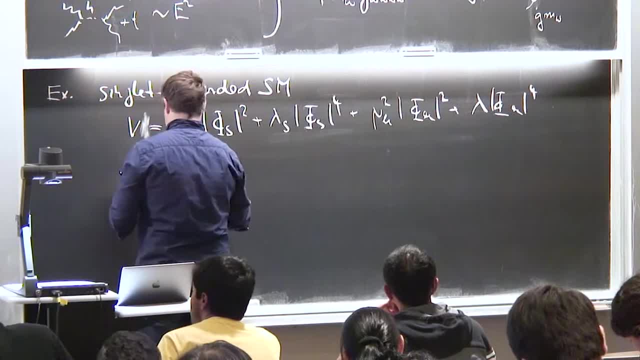 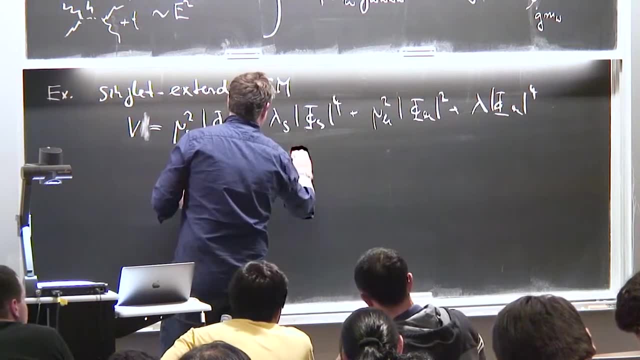 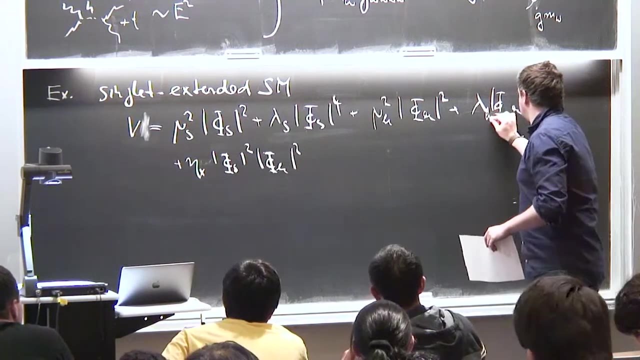 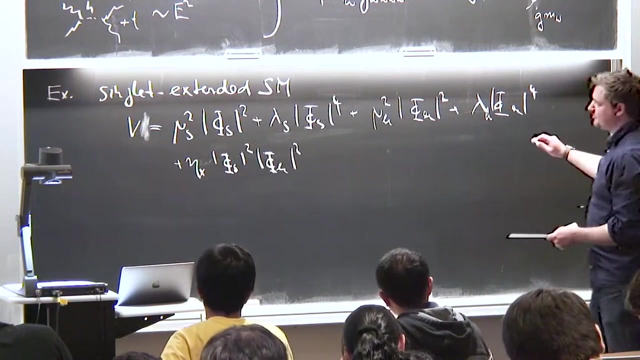 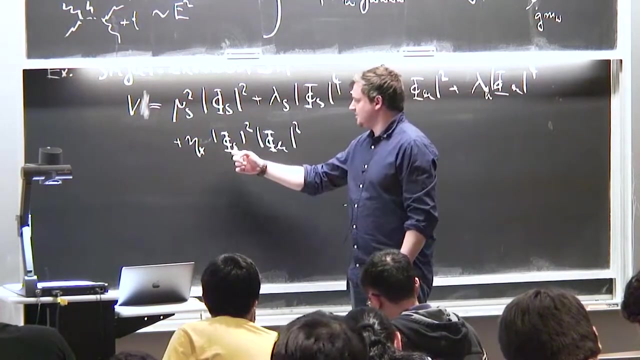 you can also mix them Plus an eta: x, phi s squared, phi h squared. So this is a perfectly renormalizable theory. Lambda h: OK. so you can find the minimum of this potential, but that's not too relevant. But what we see is both the visible sector or the hidden sector, both at the same time. 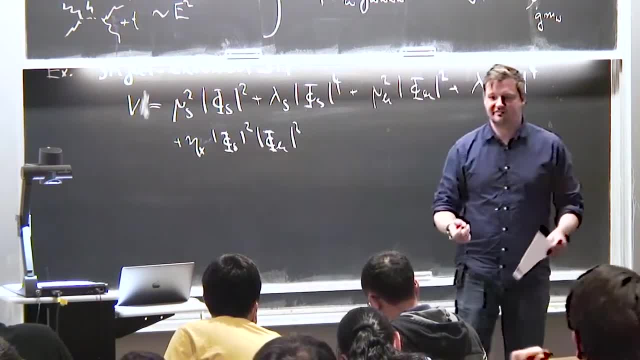 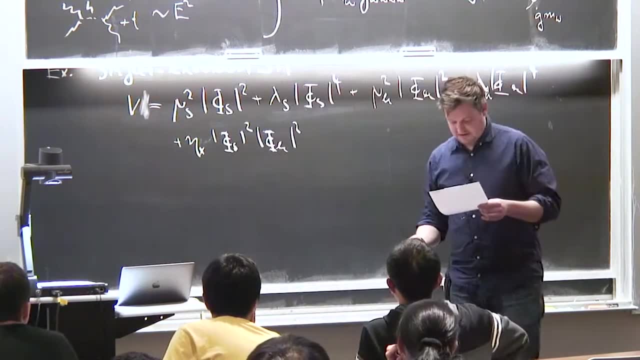 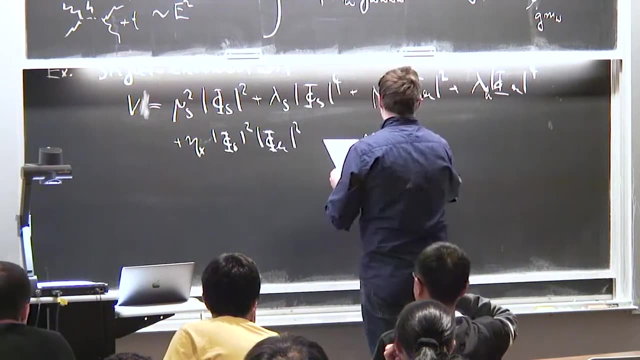 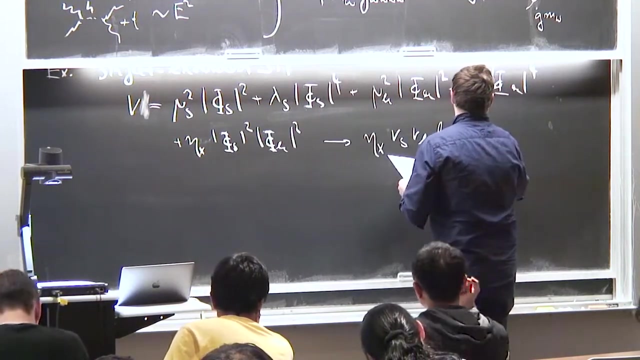 so both phi s and phi h obtain a vacuum expectation value, then this will lead to exactly this mixing between phi s and phi h. So you are. this leads to terms eta, x, v, s, v, h times, h s and h h, for like the scalar. 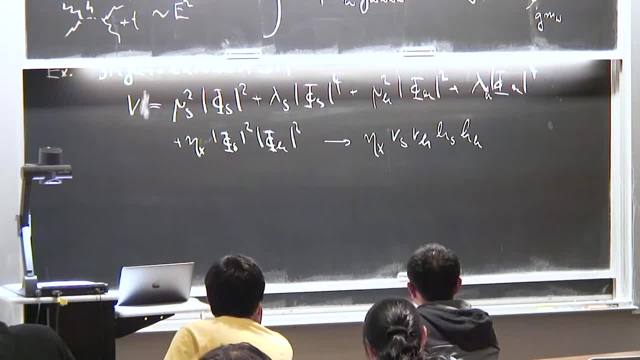 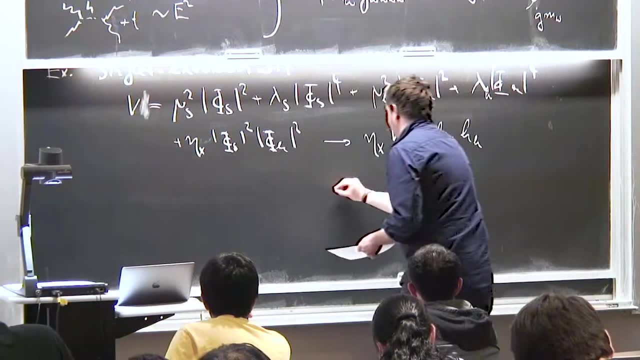 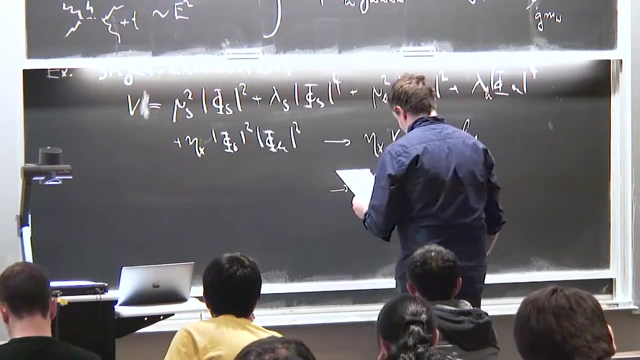 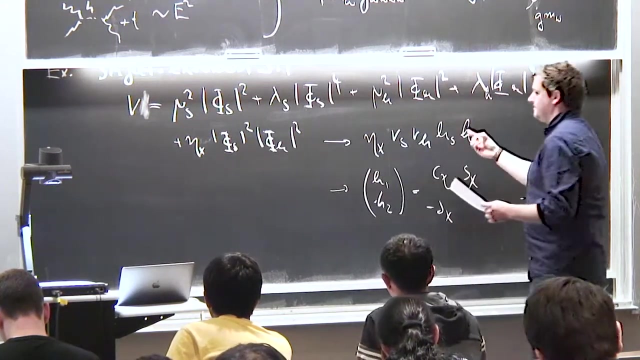 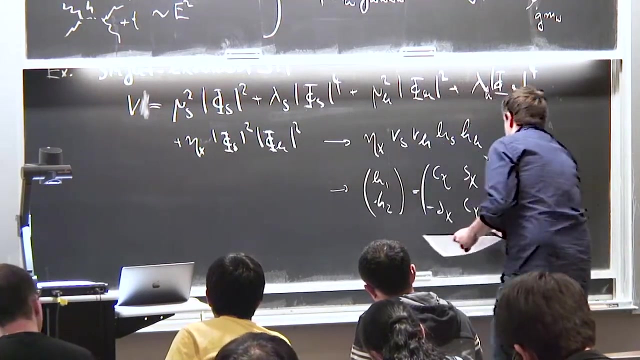 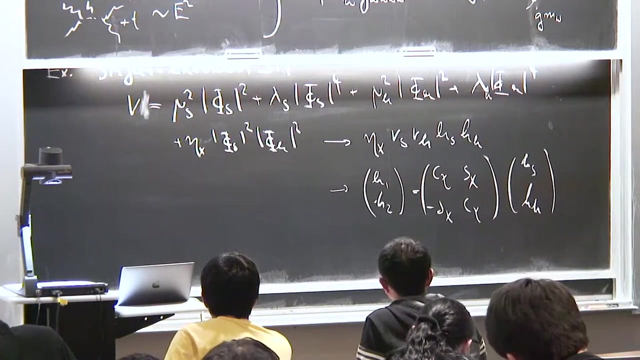 modes around these vacuum expectation values and of course this we have to diagonalize now. so this leads to a two states, h 1 and h 2, and they are related to the eigenstates here of the Lagrangian through again the two-dimensional rotation matrix and the angle I just call psi here. 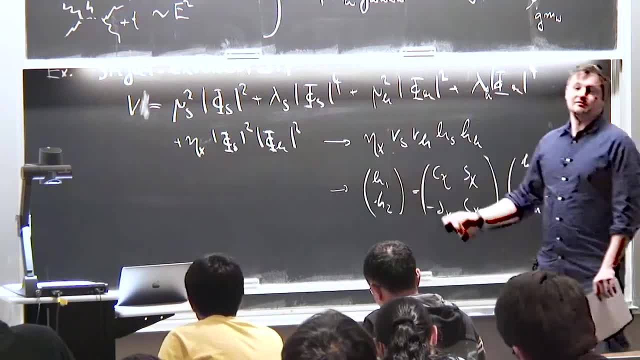 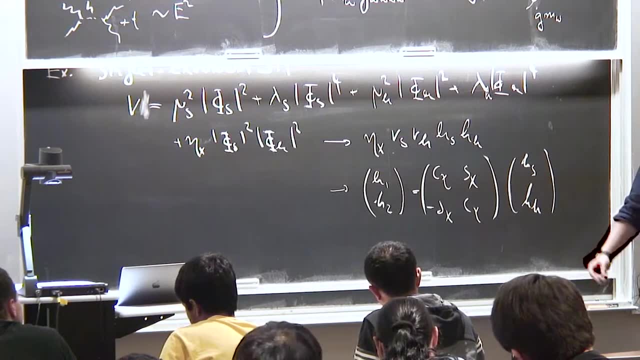 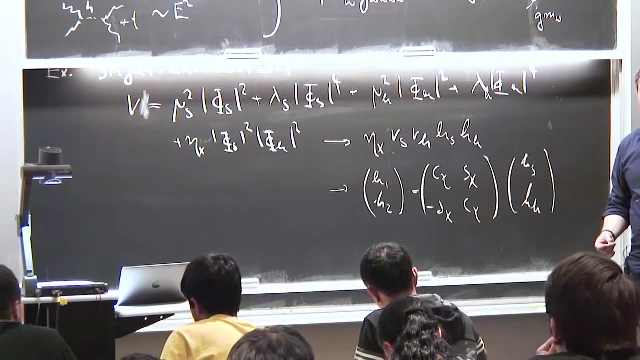 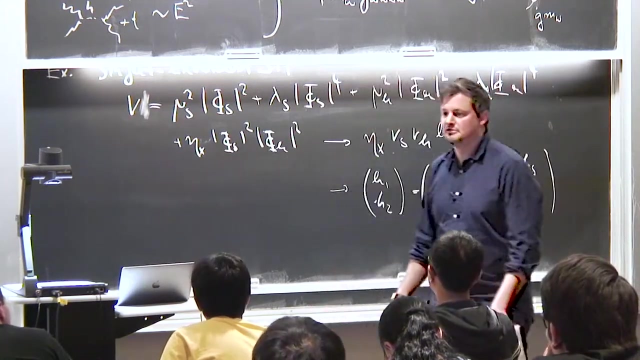 So then this mixing is gone, yeah, Yeah, yeah, I mean, this is just an example, right? You typically would apply some discrete symmetry to get rid of these terms. yeah, Doesn't matter for this. yeah, Yeah, let's take complex. 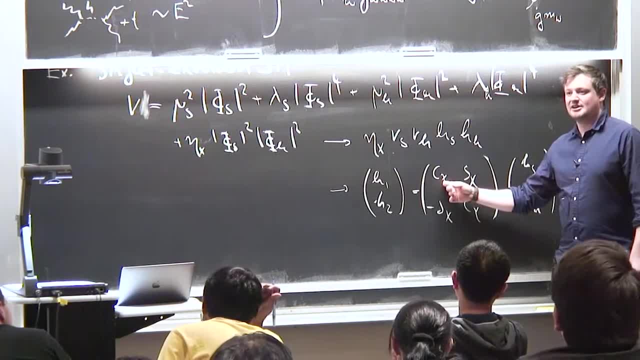 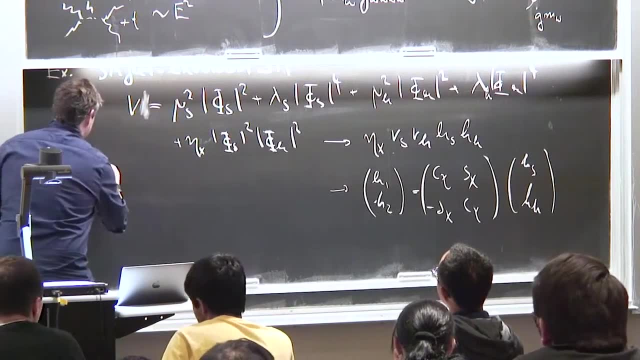 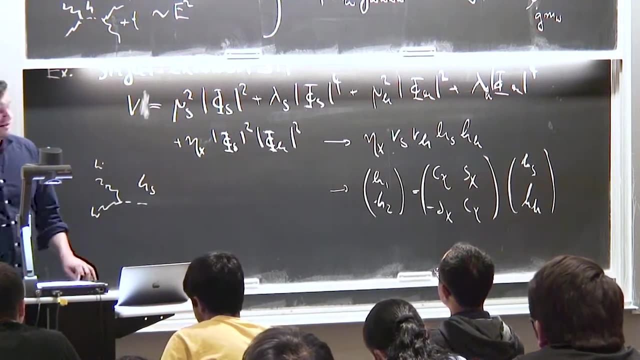 What matters for the argument is that this is non-zero. yeah, because what happens now is that, Yeah, This vertex w, w, h, s- and this is everything that would be in the standard model- gets rotated by this cosine square. yeah, 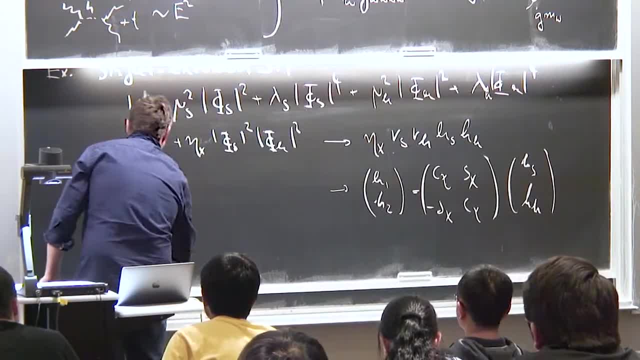 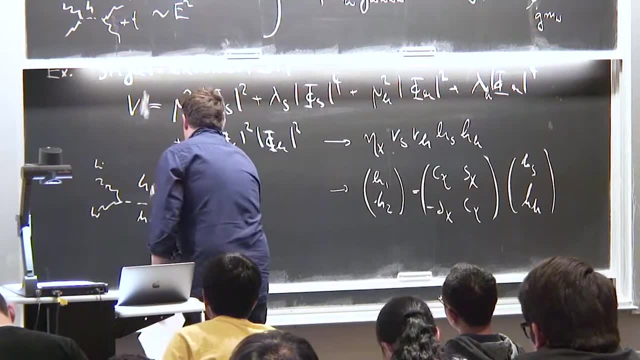 So you deal now with the h 1 and the h 2, and this couples proportional to the cosine of this mixing angle. But now it's already given here, right? So you just close it to longitudinal w's. You get exactly the same coupling here as you get here. 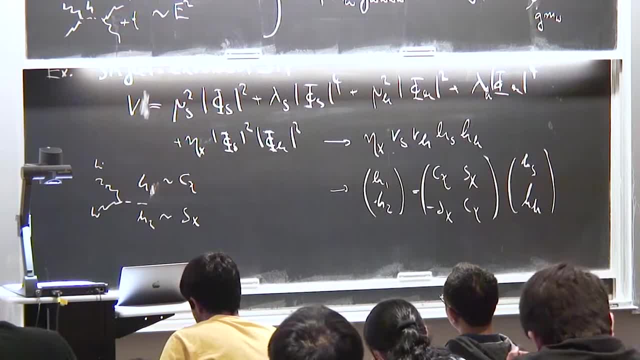 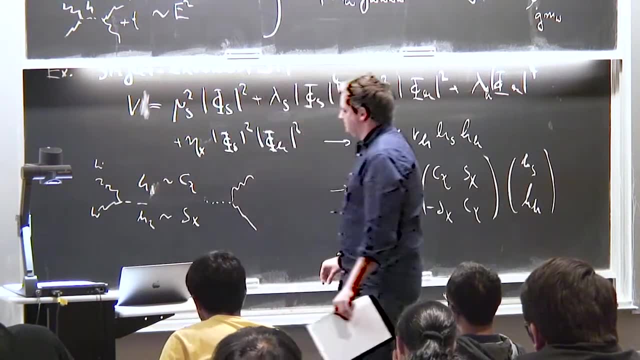 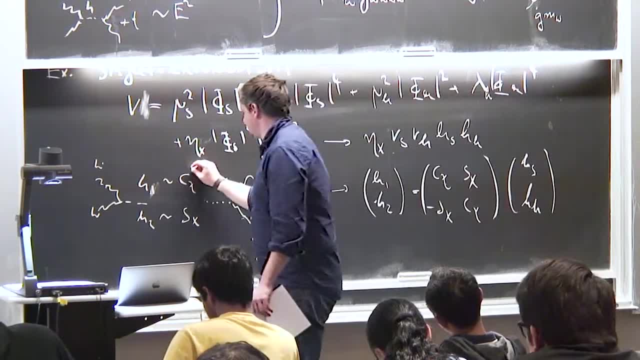 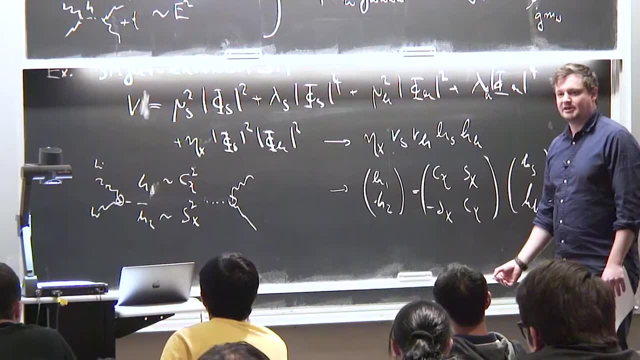 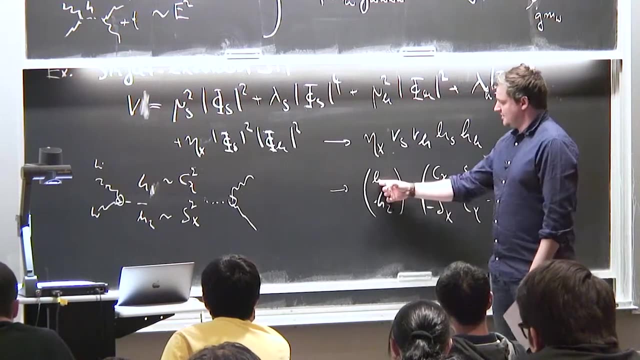 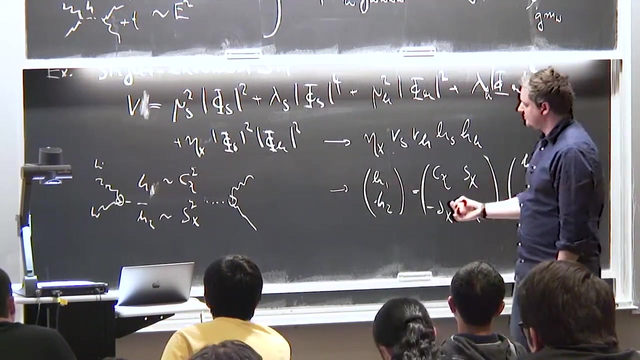 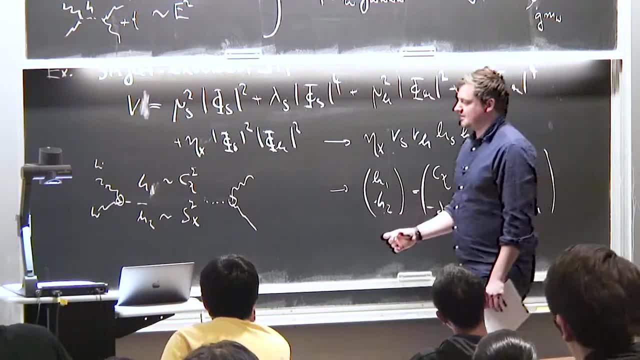 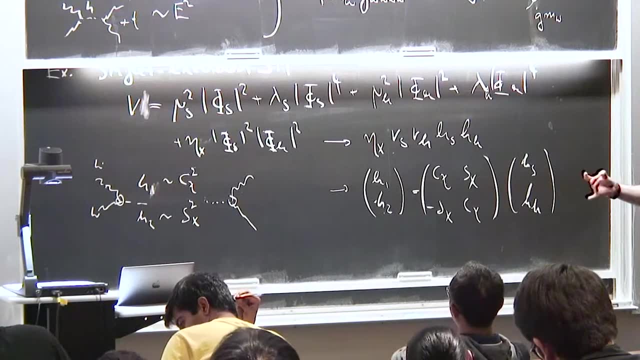 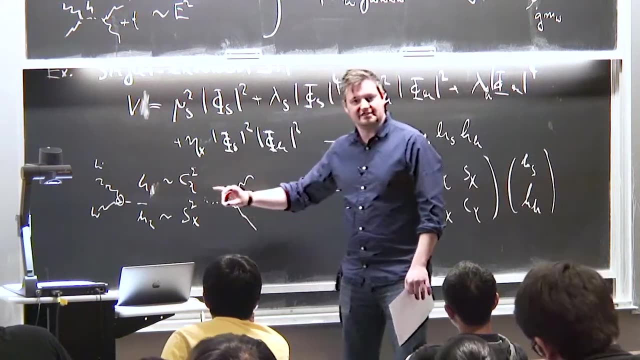 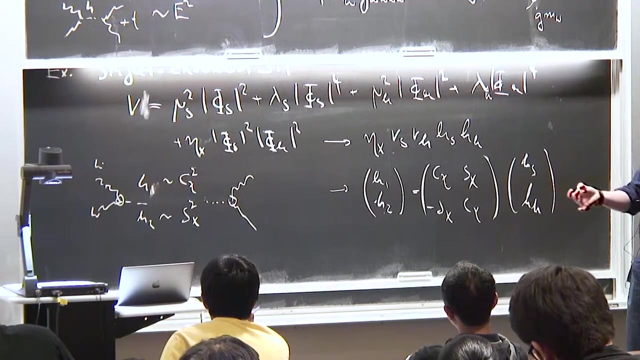 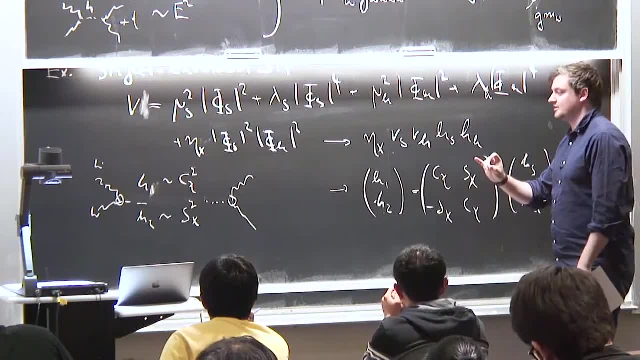 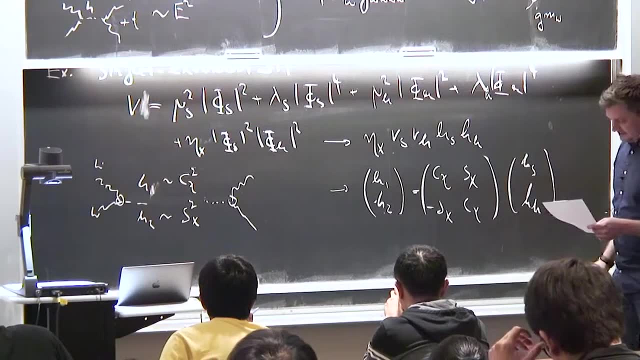 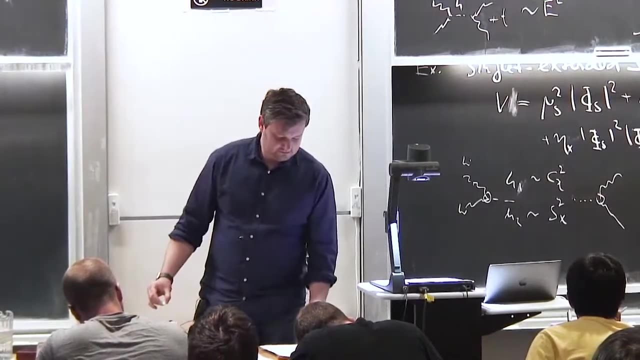 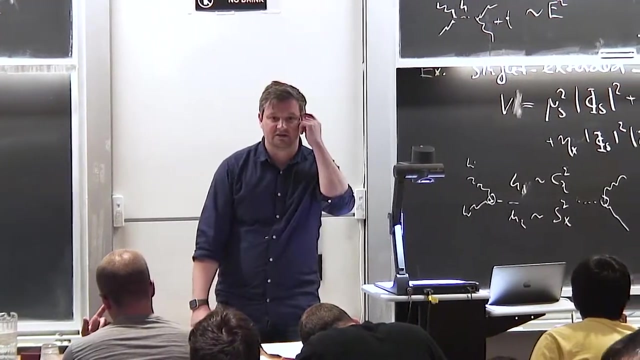 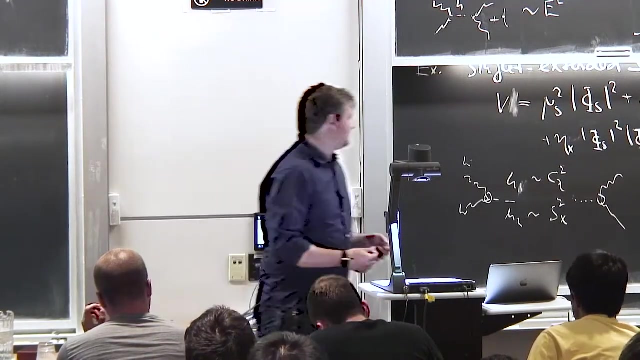 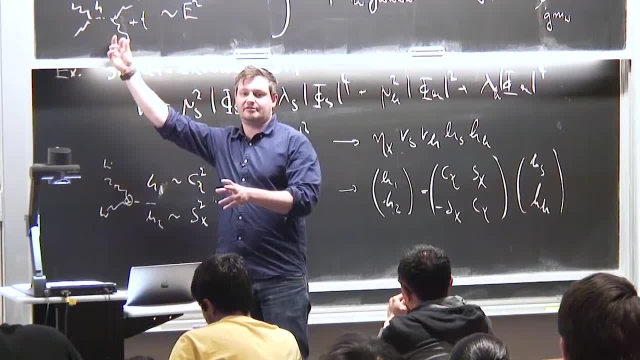 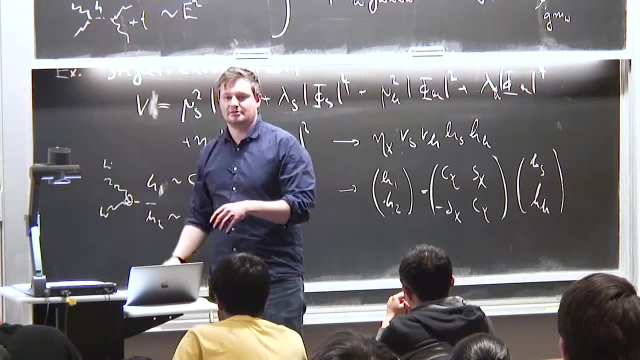 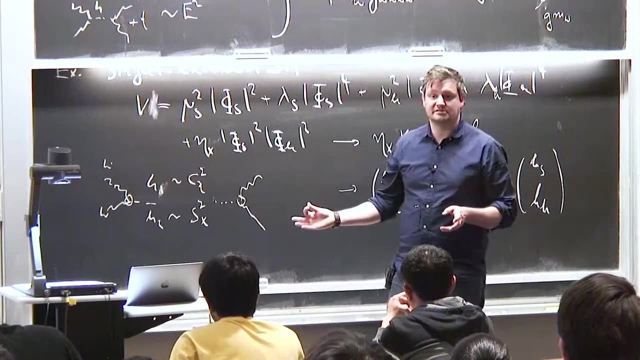 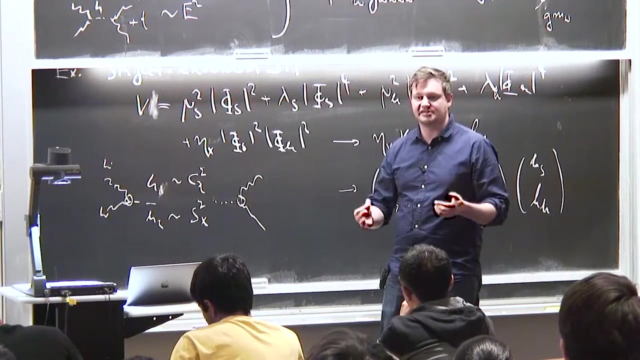 obtains a value. that is the standard model. if you're above both mass thresholds, At this point it doesn't really matter. When you start worrying about Higgs, coupling constraints and branching ratios, then of course this changes. But for this argument it doesn't really matter. but I agree So as a fully-fledged model. there are additional. 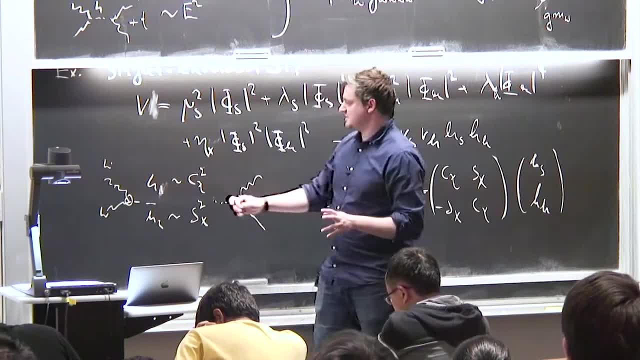 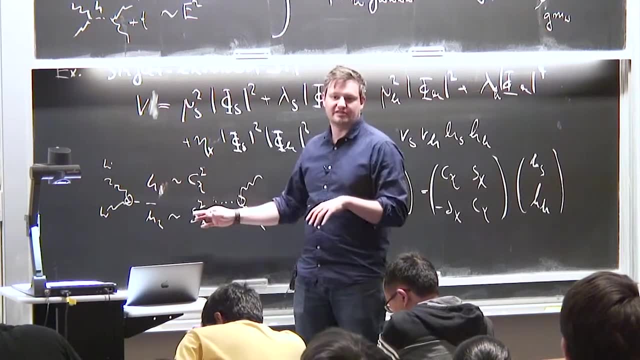 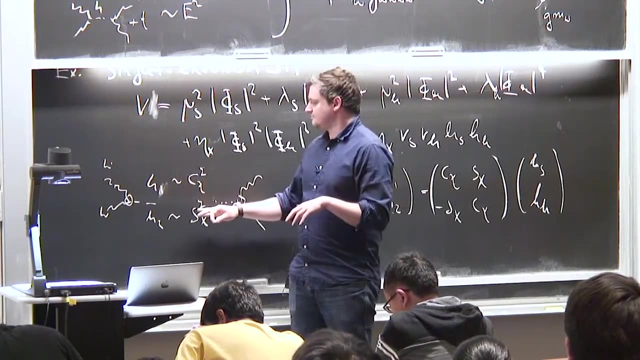 constraints that you have to worry about. but the point I'm trying to make here is that if you're above the mass thresholds you get back exactly the standard model contribution. So unitarity is restored. But unitarity is not really the most constraining bit here. If you assume now that H1 would be the light, 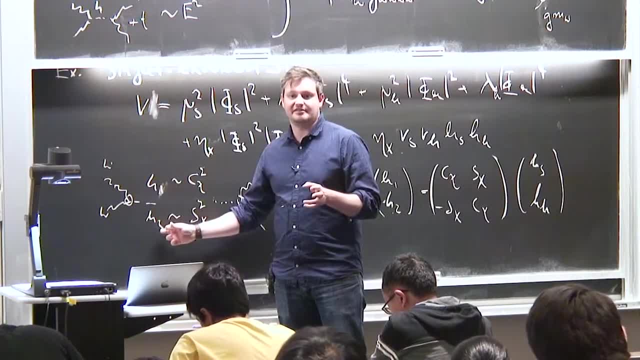 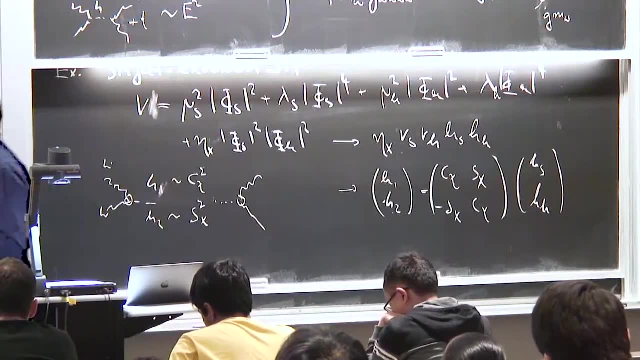 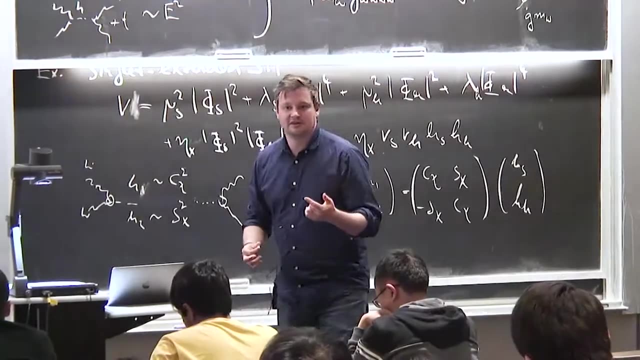 Higgs 125 GeV, and this would be heavier, say 500, 600, 700 GeV, then you get a unitarity constraint which is pretty much identical to this guy here. right, because it happens below 900 GeV. But if you then study electric reposition effects that are induced by exactly 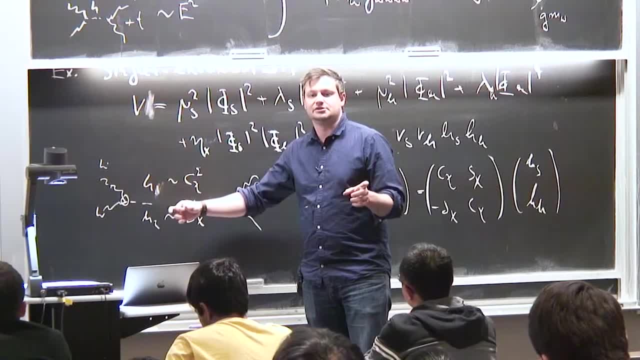 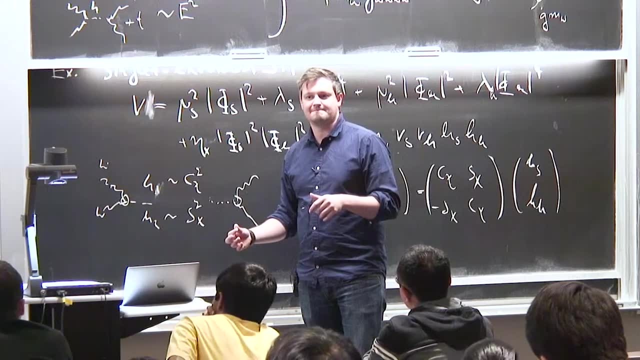 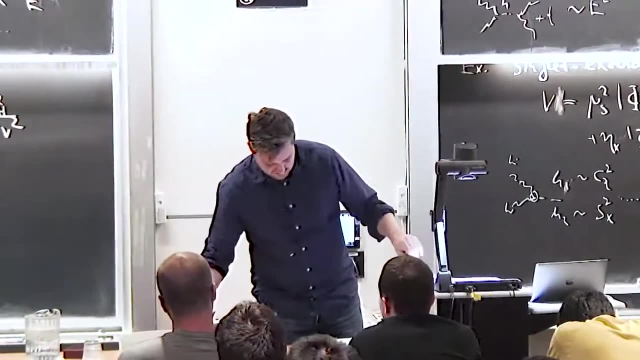 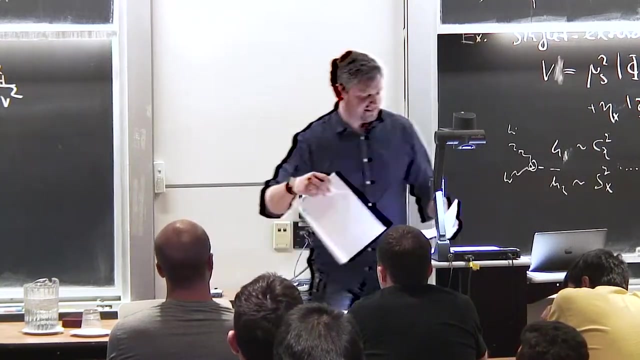 these coupling deviations, you find a much, much stricter bound, And this is what I want to do in the following. Any other questions? No, All right, So I'll upload these handwritten notes to the Twiggy, because I don't want to write down all these numbers now, But I want to talk a little bit. 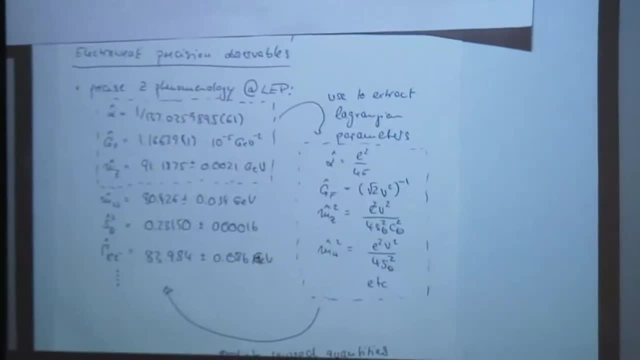 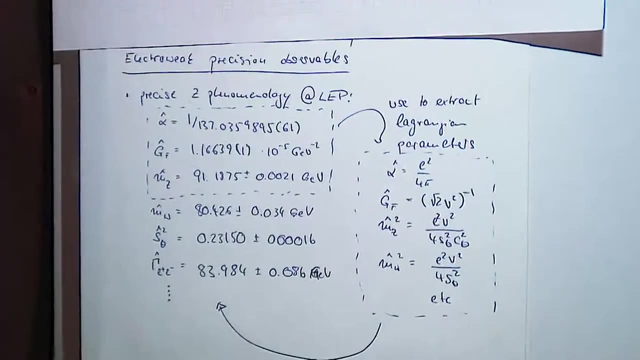 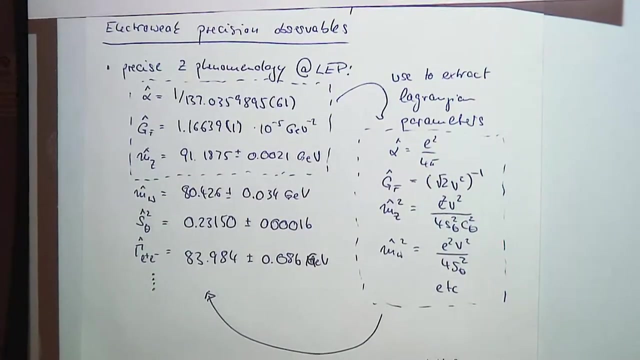 about electroweak position observables, because they are really like bread and butter physics for theoretical particle physicists. So what's the motivation behind all of this? We have now all these parameters that we can fix, So we know we can fix the VEF through the. 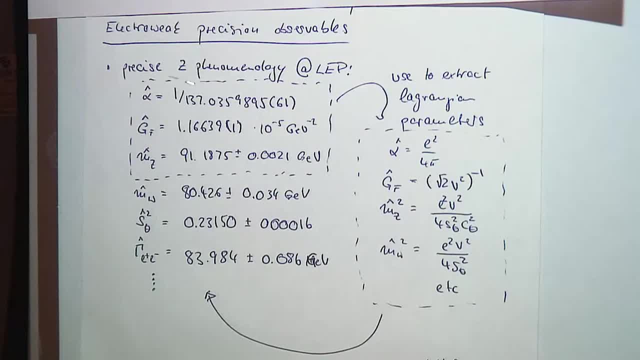 Fermi constant. We have alpha that we can, for instance. so the electroweak, the electromagnetic coupling, the fine structure constant we can fix. We can measure this from low energy, electron scattering. So we have a plethora of input. 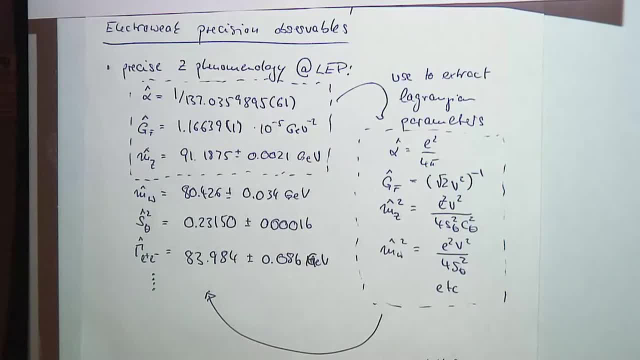 parameters. Even we have more measurements than we actually have input parameters to the electroweak sector. So now you can start doing fits and try to see if the correlation between different parameters shows you some tension. So if this picture is not consistent, 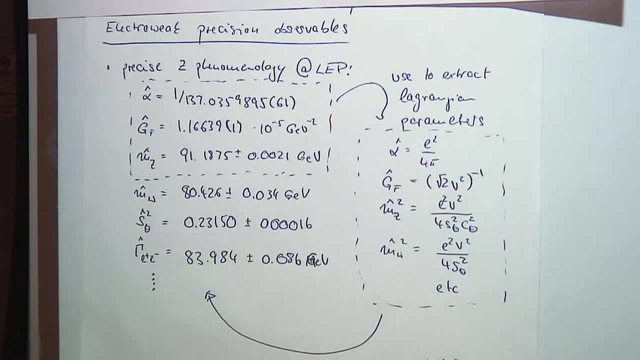 then you can take some of these observables and predict others, And if you have some sigma is off, then you should shout new physics. So this is the whole idea of this effective field theory business as well. So we do a little bit of an approximation into this through. 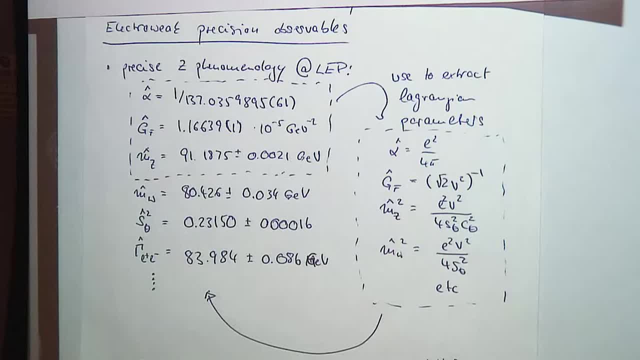 the Peskin-Takayuchi parameters. So let's do this in this particular case. So you take alpha, GF, MZ, squared and MW, for instance, and you use these pseudo-observables or observables to relate them to fundamental. 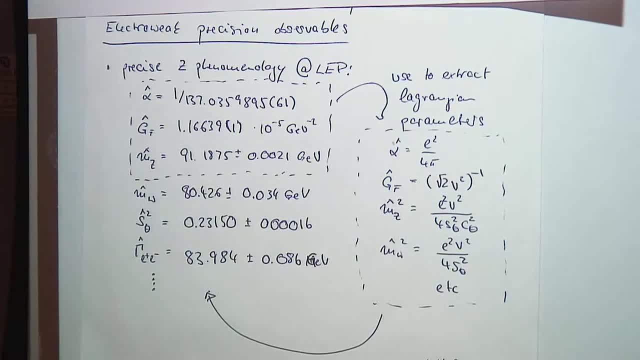 parameters. So you take alpha of your Lagrangian. So we know that this measured value here with the hat is related to the electric coupling by E squared divided by 4 pi. So you can fix E that way. You know, the Fermi constant is related to the vacuum expectation value. So with this 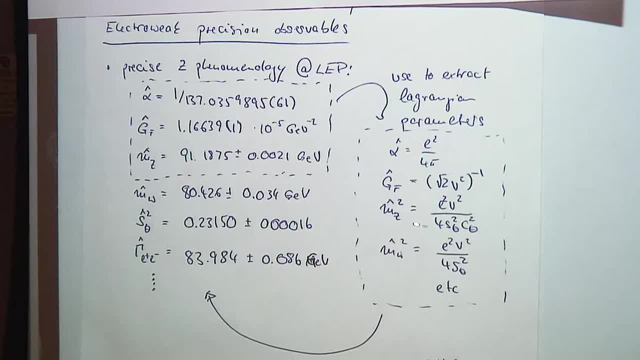 you can fix V. Now you go back to what was written before. MZ squared is just related to G squared plus G prime squared, square root of that times V squared. So now you have V and AND you are just going to add age. 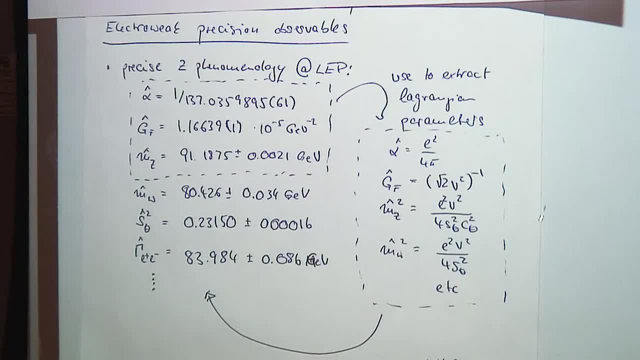 from here here to A little helps, right? Um, Oase first, and basically that is what it does, right? So youeri can go that chance that you put in Psi squared and of course a hat, and that can work, And of course you can say: home, you break that down, Then you give this mod. 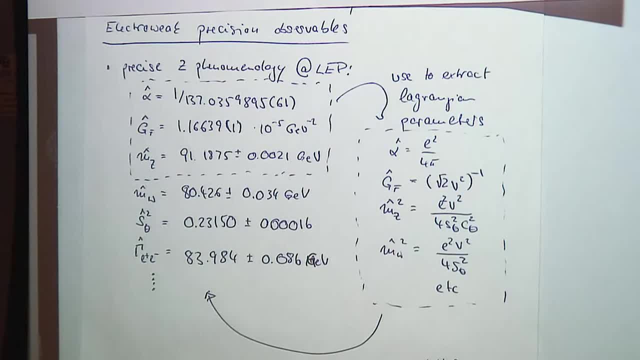 You say, predict the L plus, L minus, so the Z decay width into leptons. Or you do something different: You include that into your input parameter set and predict the W mass. And if you do this, and all of these things are super precisely measured, as you can see. 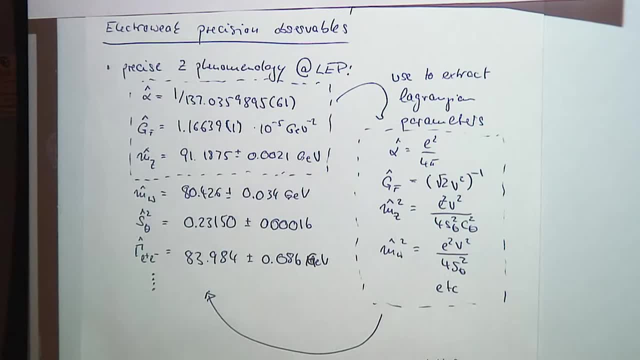 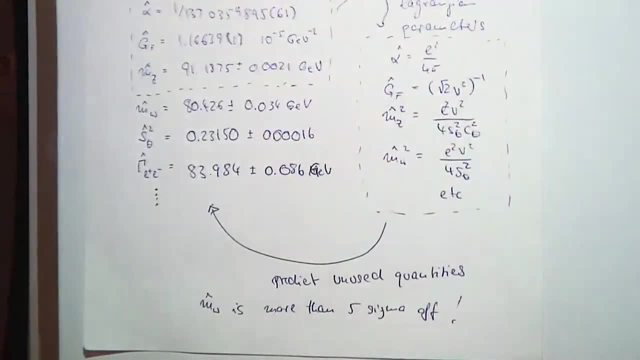 with my horrible handwriting. you can see that actually some of these parameters- you can calculate this or you just believe me- are actually off by 5 sigma, And much more than that. some of them are off by 10 or 12 sigma. 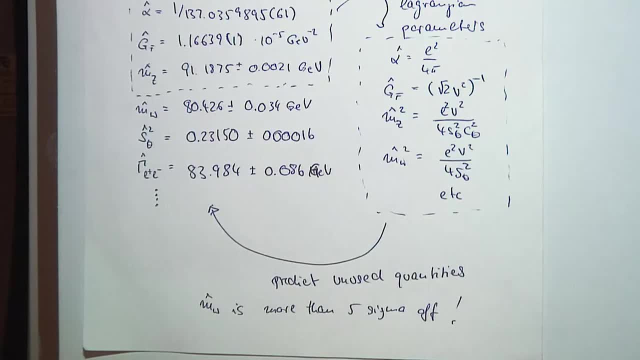 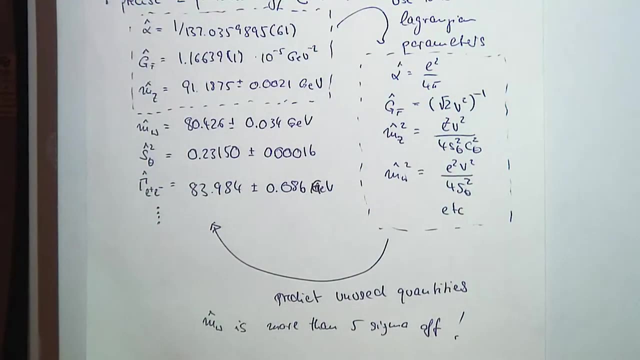 So this means actually, what I told you wasn't really worth the two hours that we spent. Of course, this is not the end of the standard model, but it tells you that if you increase the precision of your measurement, then radiative corrections become important. 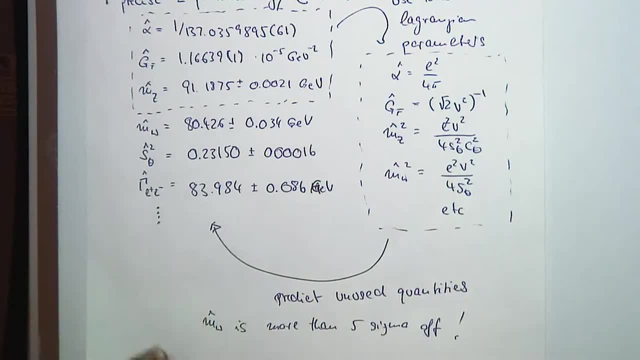 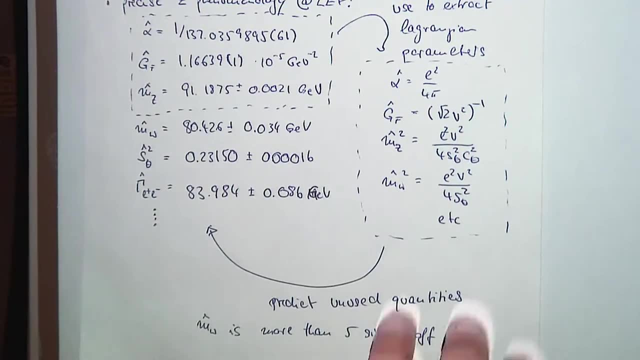 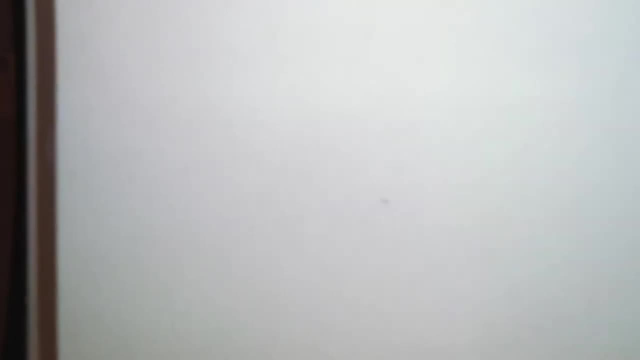 So leading order physics: once your stuff is precise enough, you can do that. So stuff meaning measurements requires you to work harder, harder in terms of perturbation theory. So how does this work? So I walk you very quickly through this, because it's sort of very matzy. 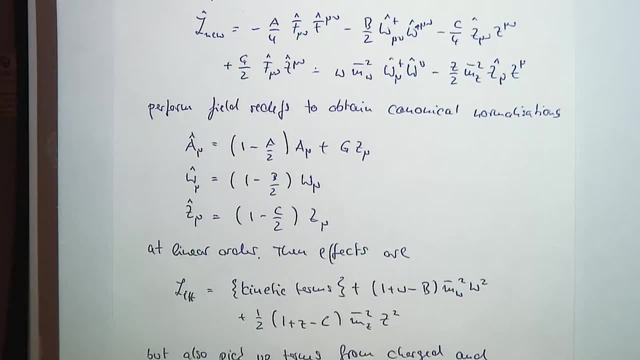 It's not super complicated algebra, but it's a lot of it. So the point here is that what you have, of course, if you look at E plus E minus, scattering, for instance, to Q- Q bar, that's really what was done at lab: E plus E minus. 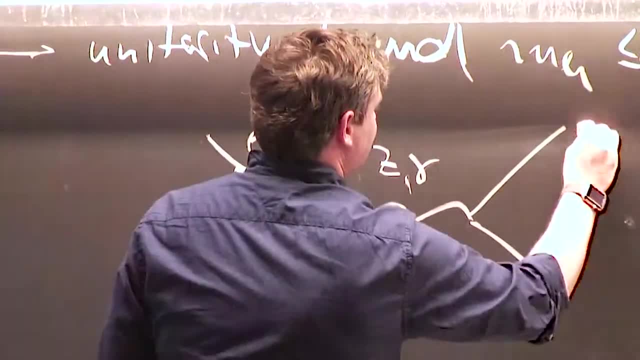 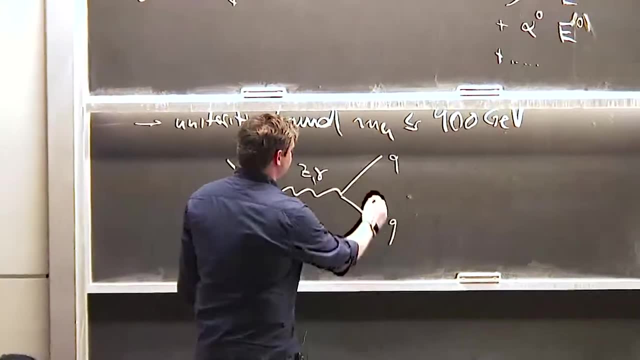 So you have Z or gamma and you observe this in two quarks. Then in higher orders, you can write also. you can write also. you can write also. you can write loads of corrections to it. You can, for example, write a loop here. or you can write a loop here: 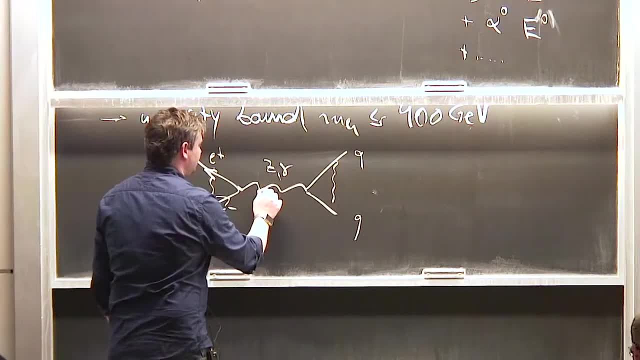 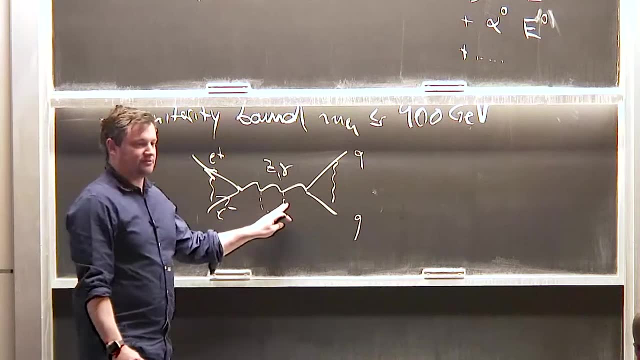 or you can also write loops here, for instance: right, So you can have a Higgs, for instance, like this: Okay, and some of these. you can think about this being really a new physics field that impacts this measurement in the low energy regime. 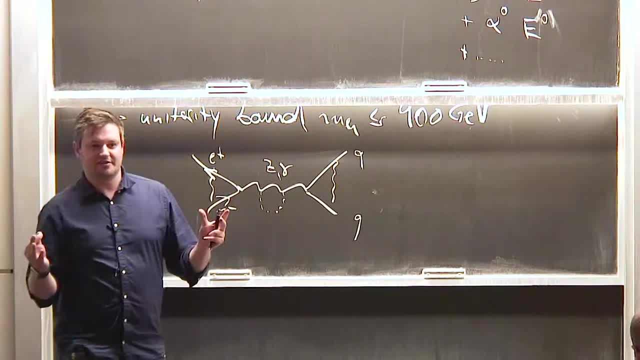 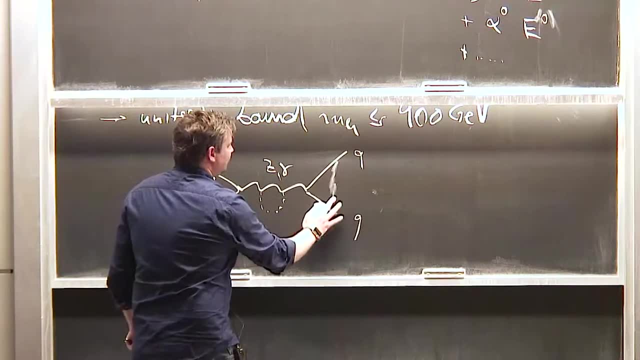 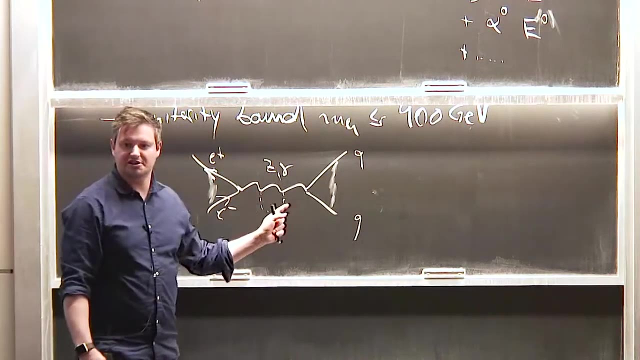 And if you assume that whatever this new physics is, it couples predominantly to to the gauge bosons, then new physics corrections of this sort of type. they will not be dominant, but it will be stuff that relates to corrections of the two-point functions of all gauge bosons. 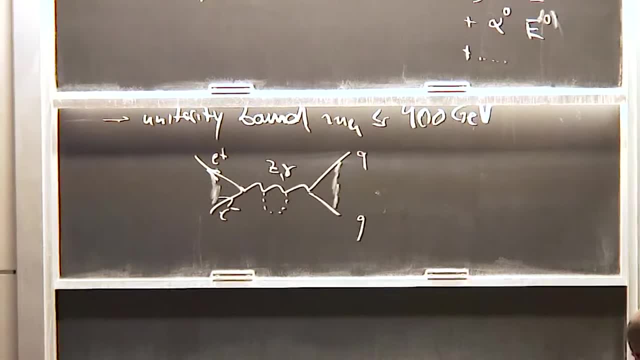 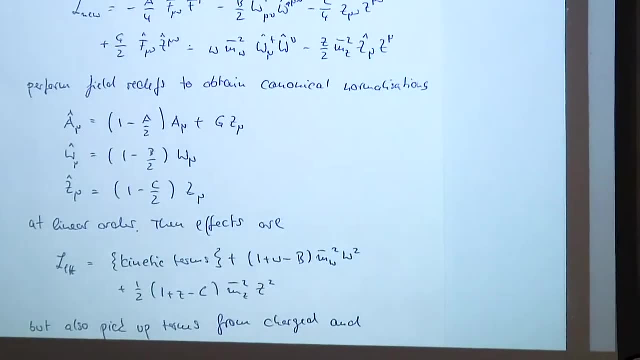 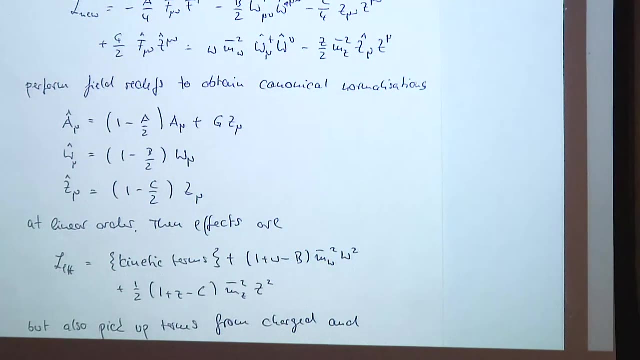 So if you assume now that this is the case, then you can write your new effective interaction below whatever the mass scale is of whatever runs in the loop here as the standard model plus some new interactions, and these new interactions will only modify the kinetic terms. 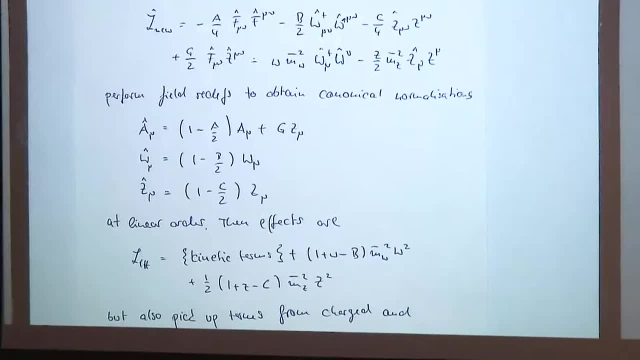 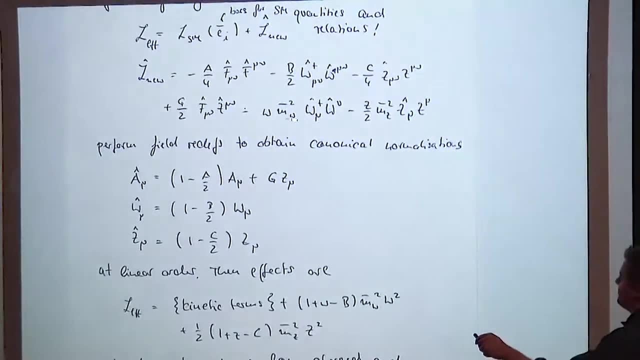 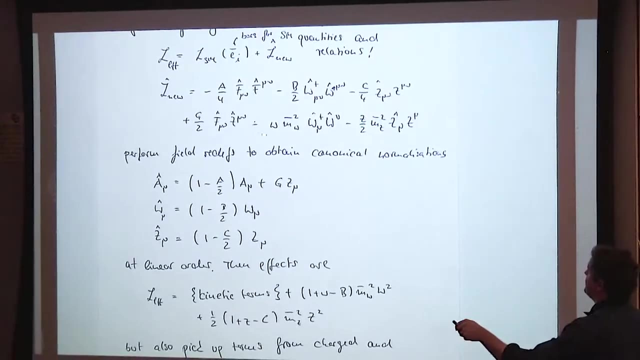 or the mass terms of the associated gauge fields. So these are related to exactly the two-point functions. So, integrating out these states, you end up with some number A that we would like to measure and number B, C, G, D and so on. 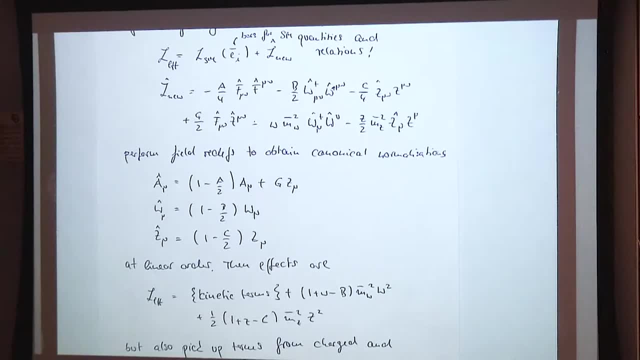 So you have A, B, W and Z, And because we like perturbation theory so much, what we have to do to apply it is shifting and renormalize these fields such that we deal with canonical normalizations, And this is where it gets a little bit tedious working through these things. 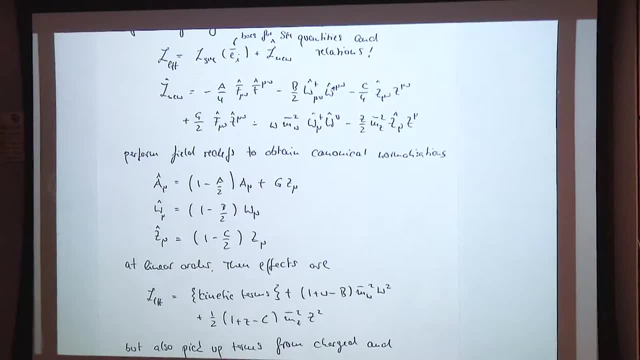 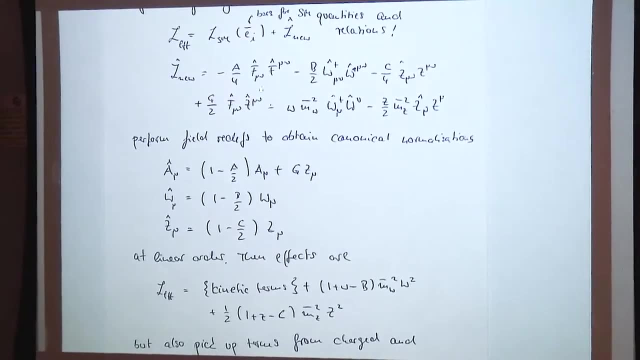 Like Mathematica, you can probably do this very quickly. So, in order to get rid of this, you rescale A just by the number of these. So, in order to get rid of this, you rescale A just by absorbing exactly this additional factor. 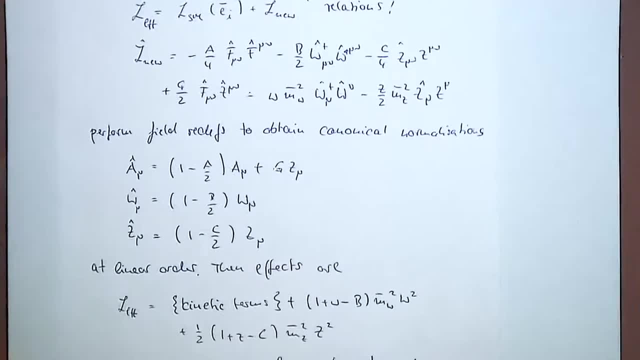 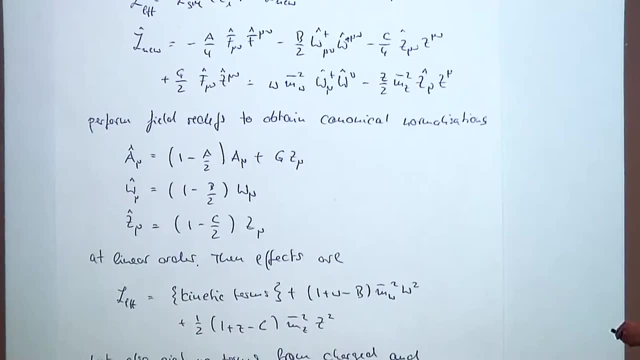 And there's additional margin here for photon Z mixing, which is given here. So this is parameter G. You do this with the W fields and you do this with the Z fields And you work at linear order because you assume that these parameters are reasonably small. 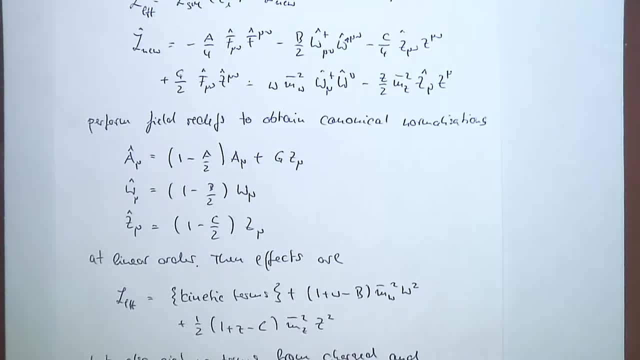 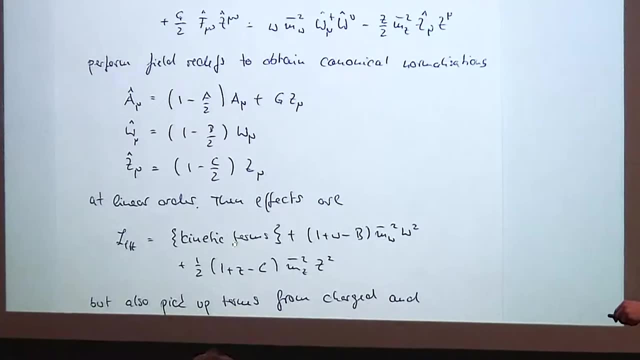 so new physics is heavy or weakly coupled, or probably both, And if you do that by construction you end up with kinetic terms. So you don't really need to sort of copy all of this away. I'll put this onto the Twiki. 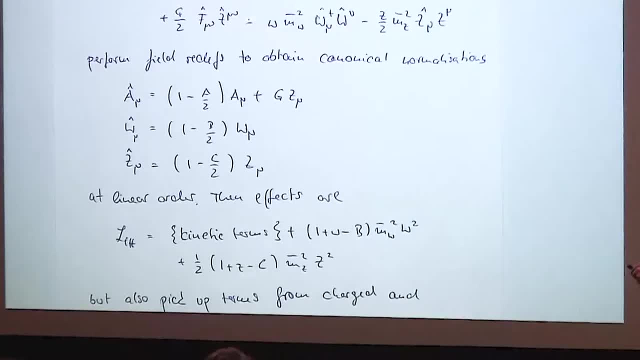 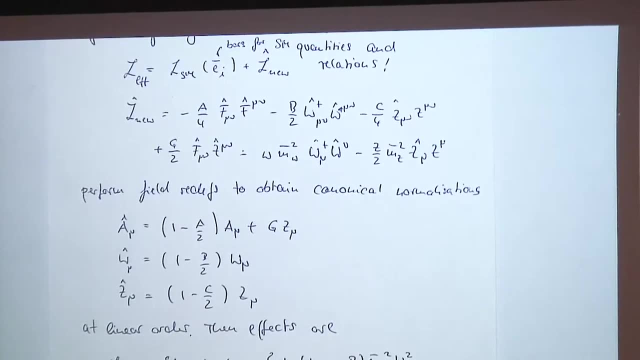 But now all of these coupling changes will of course affect here the modifications of the W mass, because this piece here will field whatever kind of field redefinition I've done So. now my Mw squared has this additional factor of B and my Z squared has this additional factor of minus C. 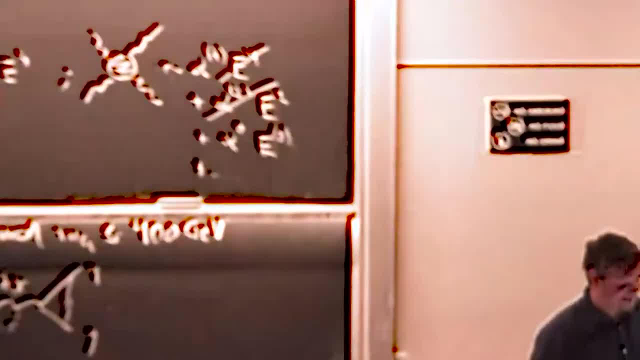 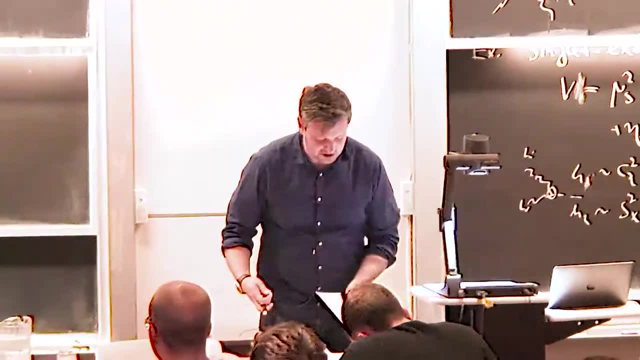 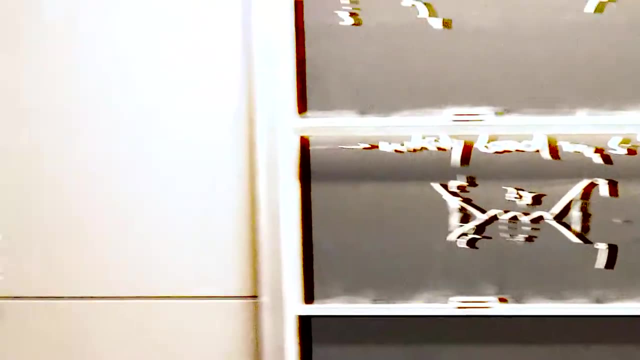 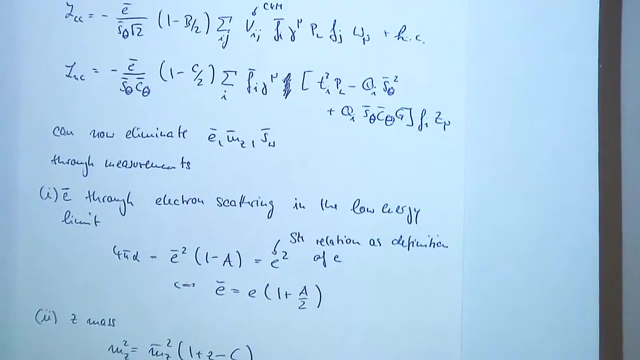 But even more so, the interactions of the Ws in the sets with fermions will be modified as well. And this is now you see why I do this here on the projector, because writing this on the blackboard is a pain. So, similarly, you will rescale the electromagnetic currents. 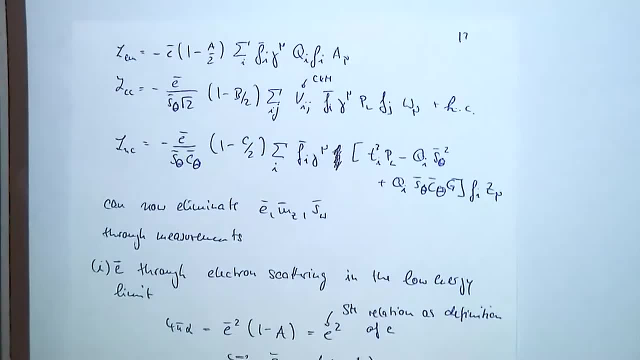 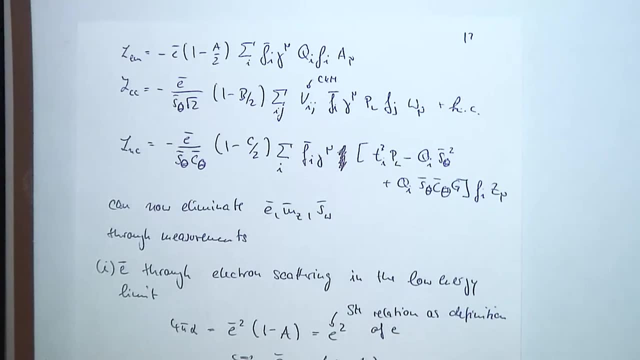 the charge currents and the neutral currents, And you will also modify it. You will modify them through exactly this additional G factor. And I should have said that the bar quantities are really standard model quantities, So I'm allowed to use standard model relations for quantities that have a bar over them. 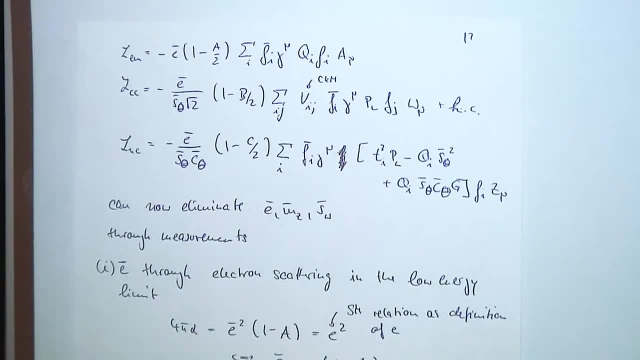 So now we actually have quite a horrible Lagrangian that we're dealing with. The only thing that's really nice to us are the gauge kinetic terms, and we don't really need to worry about that anymore. But- and I keep going on about it- 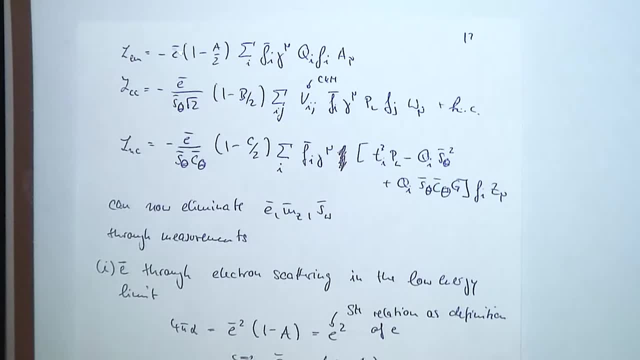 and I talk about this all the time- none of these parameters is really physical, but they are related to physical quantities through measurements. So now we can eliminate some of these guys through measurements. So for instance, we can take the electric coupling, the Z mass and the sine of the Weinberg angle. 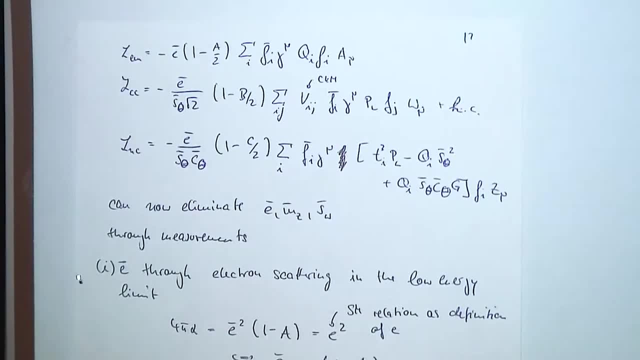 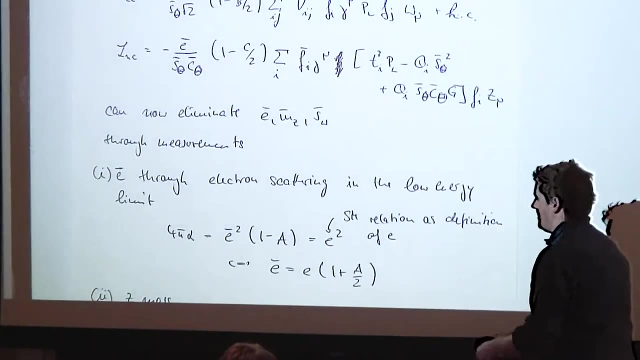 and work them out. So we can fix E through electron scattering at low energy And we know that this essentially gives you defined structure constant And you can take this as a definition of E and you match it to your new coupling that is shifted by this additional factor of A. 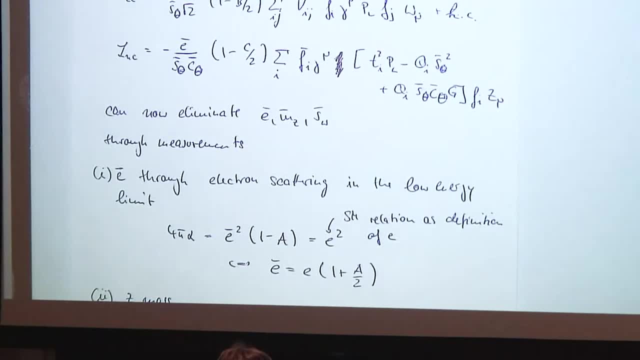 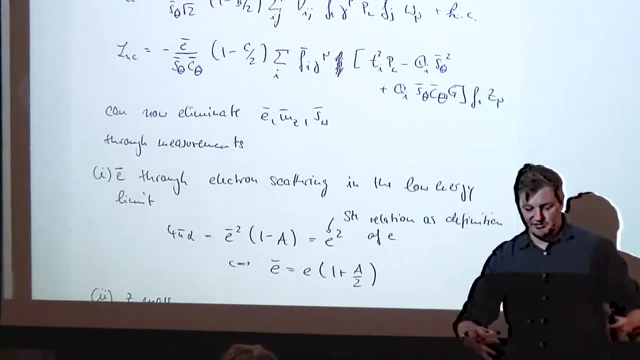 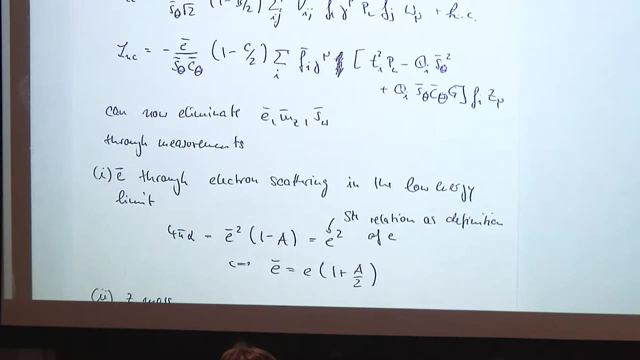 And there's a factor of 2 compared to here, because we're dealing with A squared and then linearized. So what this means here is that you do the measurements. so you measure like a cross section of electron scattering at a given energy, and typically you would do it at zero momentum transfer. 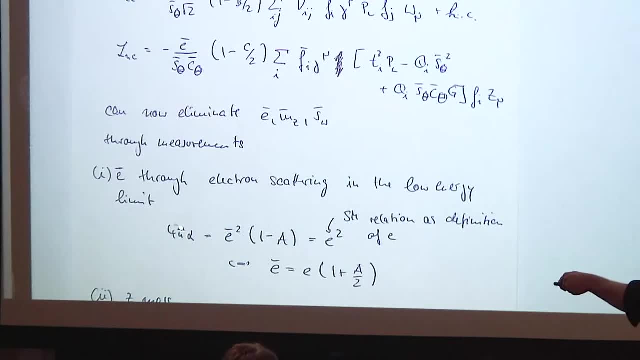 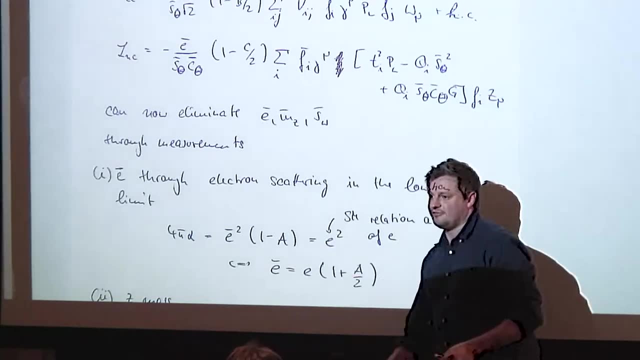 And this is really what this left hand side here summarizes, and you use just the standard mode of relation to define an E that you like. What this means is it's a placeholder for a physical cross section. So this is the idea of renormalization, over and over again. 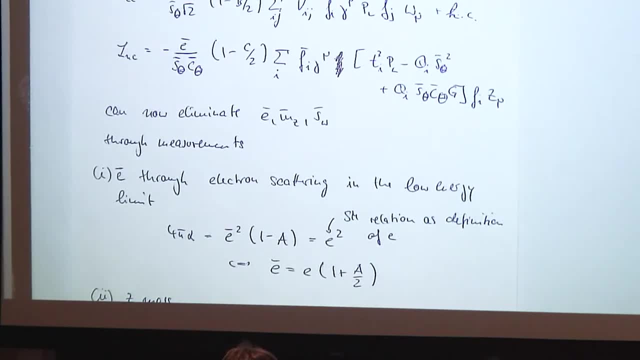 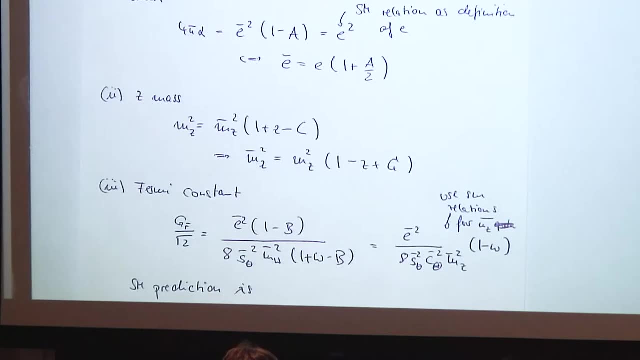 but here in a finite kind of way. So you do this with the Fermi constant as well, And this gets a bit more worse, if you wish. So you calculate the muon decay. use all the modifications of the Feynman rules that arise through these field rescalings. 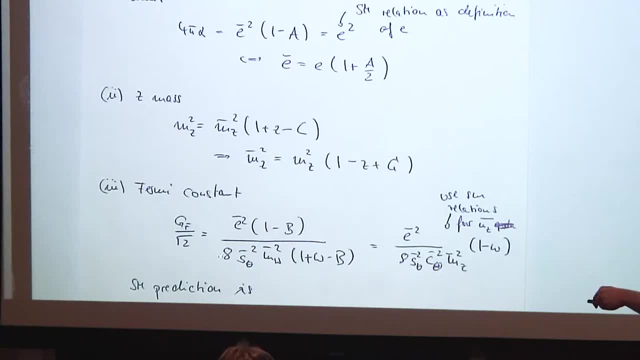 and if you do that, you end up with an equation that looks like this: And remember that these bar quantities are standard model quantities, so I can use the standard model relations to put these in. Okay, So the standard model prediction. for this we never really worked out. 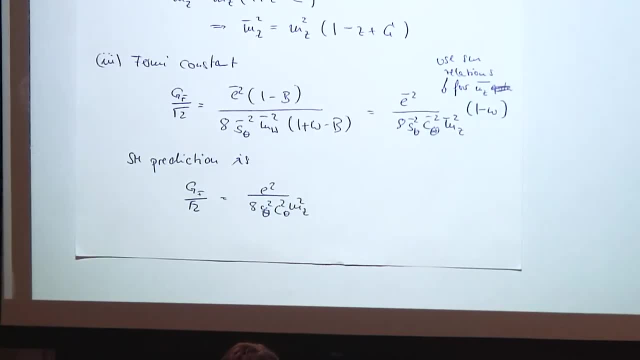 but it looks like this And I can use now, essentially, the measurement of muon decay, understood as a function of the Weinberg angle, to fix the Weinberg angle in this new modified theory. Okay, so what I want to do is I want to write. 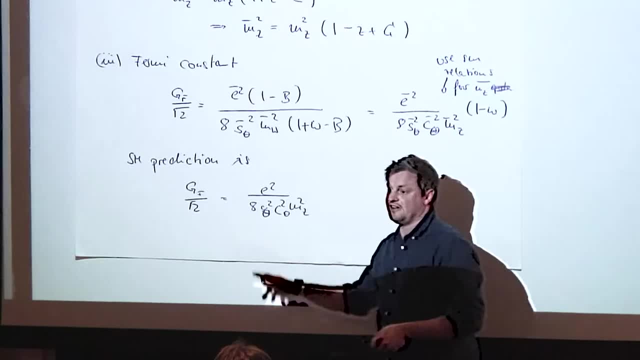 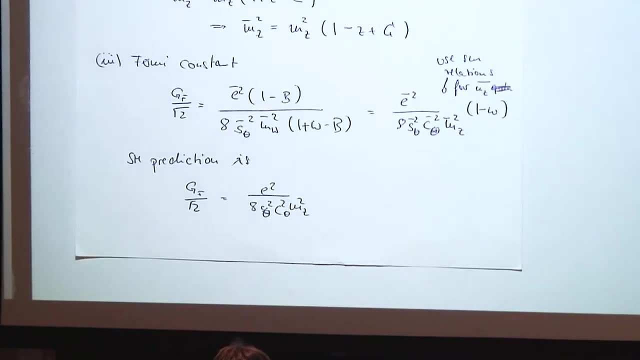 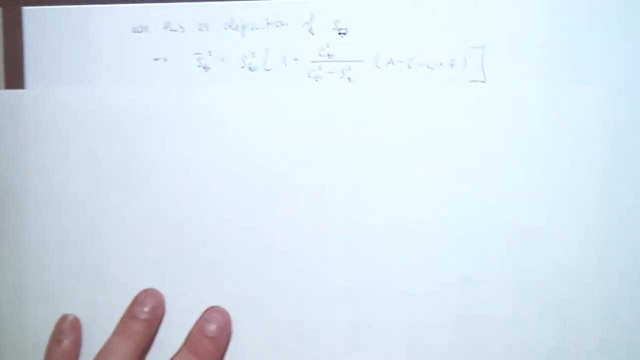 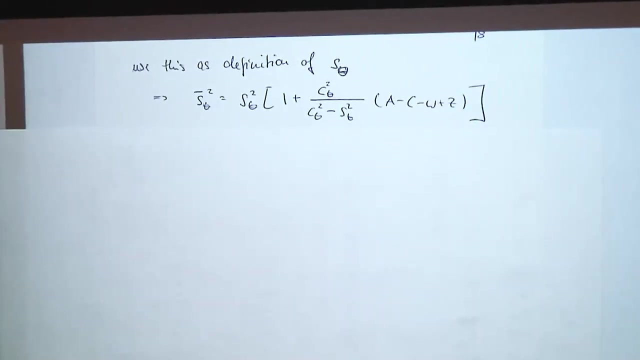 S theta bar as a function of S theta, And this can be done, And you have something like this. Alright, so quite horrible. So essentially what we are doing here, and don't worry about the algebra, it's really not too important. 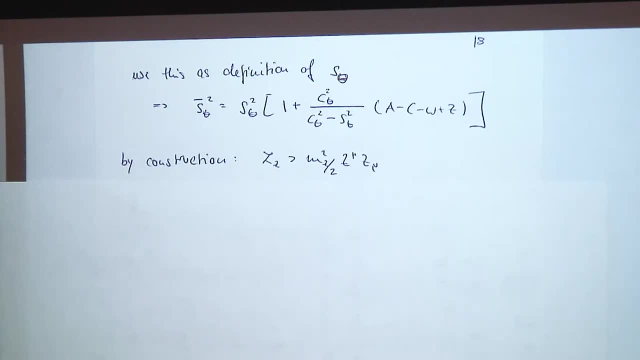 It's just trying to identify how these parameters and how these new physics sources get shifted around in the Lagrangian and what they later on really mean in physical quantities. So if we've done that, then by construction I mean because we use the Z mass as an input parameter. really, 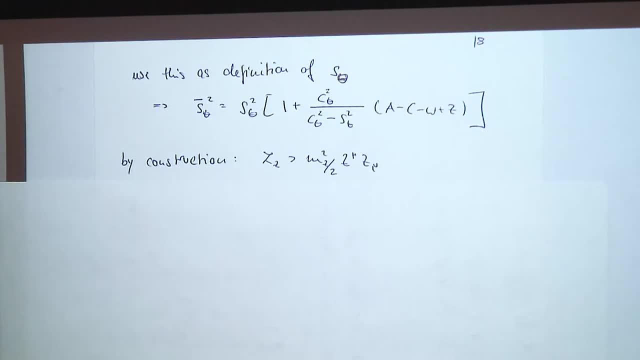 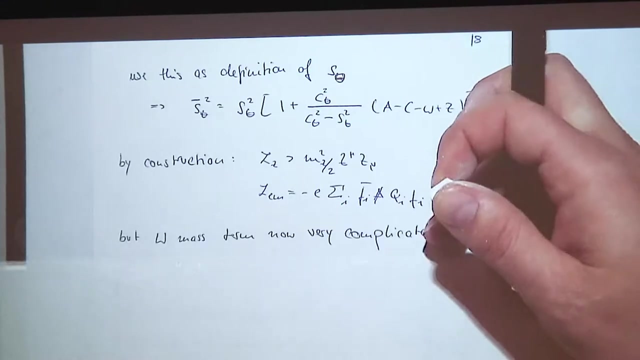 the Z mass will be exactly what it should be, will be MZ squared divided by 2, times Z squared. as a Lagrangian operator, The electromagnetic current will be exactly the same as you would expect in the standard model, So it's fixed through electron scattering at low energies. 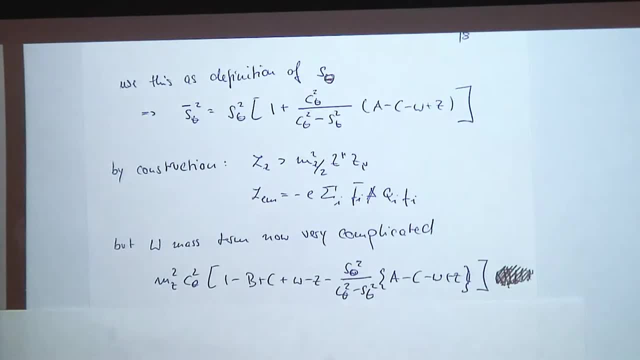 But the W mass is a bit more complicated. So essentially now you've shifted all these parameters, all these modifications, that we scaled our photon field, we scaled the Z field, the W field, the W mass, the Z mass. You've all absorbed them into a modified prediction. 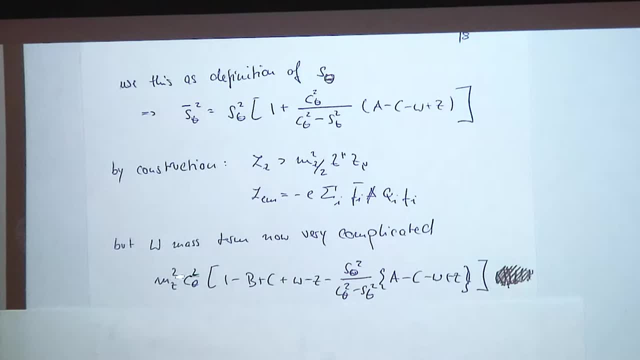 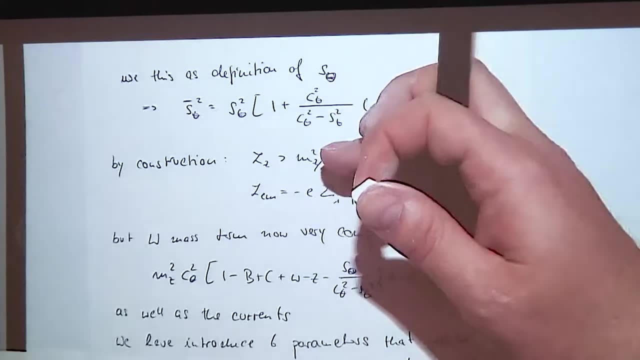 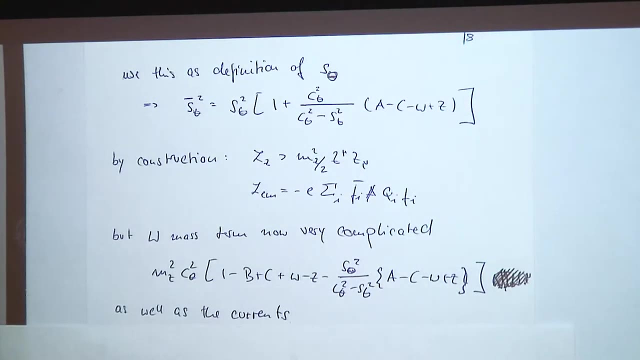 of the W mass. So W mass now looks like MZ squared plus all of this clutter. So the currents are of course the same. They get complicated as well for the W. But now you can go on and say: measure the W mass as a function of the Z mass. 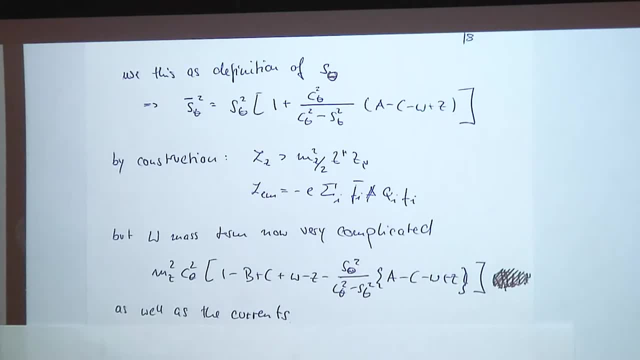 as a function of the Fermi constant and so on and so forth, and compare all of these things. So equations are not the end of it, but you can make it a qualitative statement. So we deal here with six parameters. We have the photon field strength. 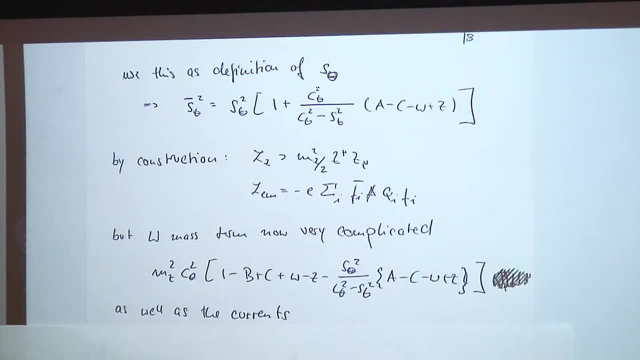 the Z field strength, the W field strength, the Z photon mixing and two masses. So we have six parameters, Three of those we can absorb into a redefinition of the associated gauge fields. So we are left with three combinations of these parameters which are really physically relevant. 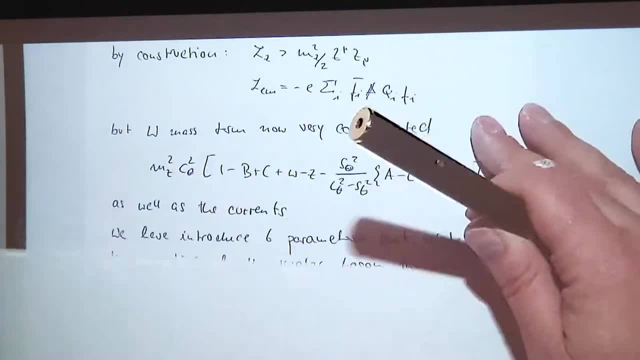 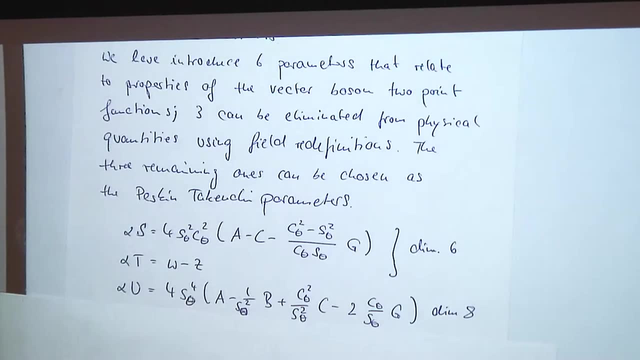 And these are exactly the Pesky and Takeuchi parameters. So, in terms of these ABCs and Gs, they are written like this: We have the famous S parameter and the T parameter, So there is no reason why you need to learn this by heart. 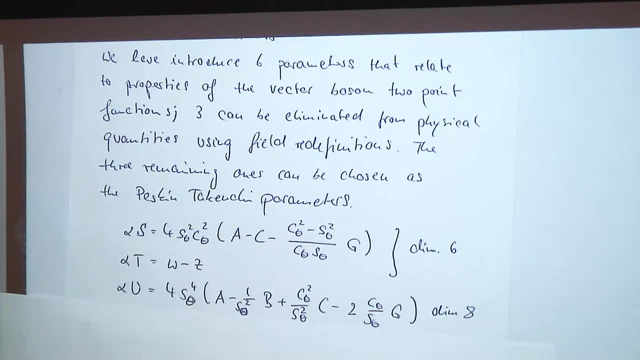 But what I want to say is that these are dimension six, so you would expect them to be leading deformations of the standard model, because there are no dimension five operators in the standard model as far as I'm concerned, And the T parameter in particular gets rather simple. 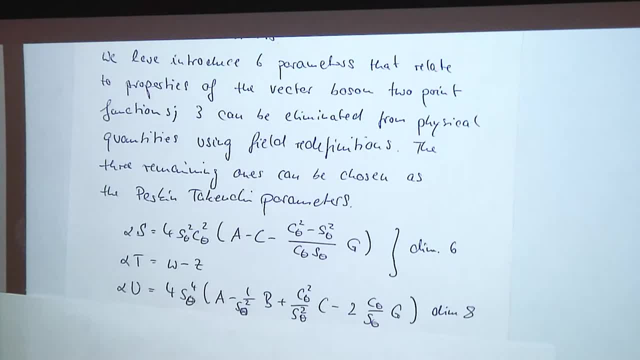 So it's just remember that the small z and the small w were just new contributions to the w and the z mass. So the T parameter, as I said earlier, really gives you a shift of the relation that we found through custodial isospin. 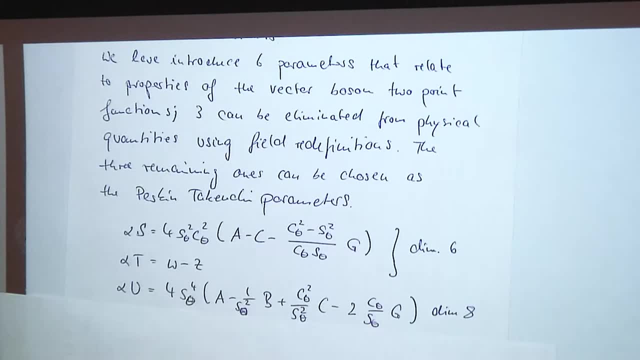 So that mw squared divided by mz squared, divided by cosine squared, theta is equal to one And the T parameter picks up on exactly modifications of this relation. And that comes about by comparing the large currents and the neutral current interactions with masses. So if you have these interactions measured, 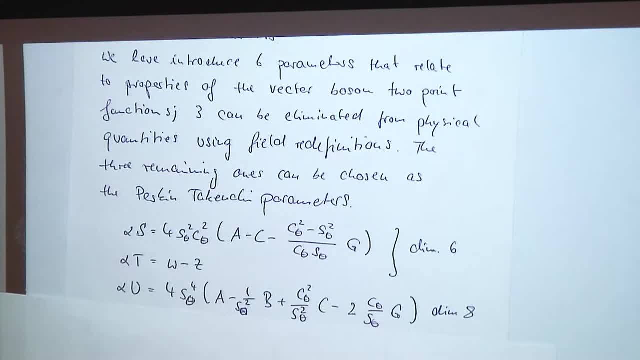 and you have the z mass, you have a prediction for the w mass, And if you can arrange them such that they are one, then we would exactly get back the leading order expression that we are after. So I said that these things are related. 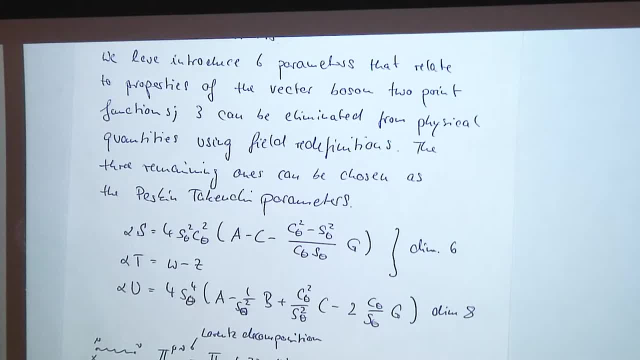 to gauge Poisson two-point functions. They have to be because essentially what we are dealing here with is a field strength renormalization and a mass renormalization. They are fully encoded in the two-point functions. So if you look at a propagator here, 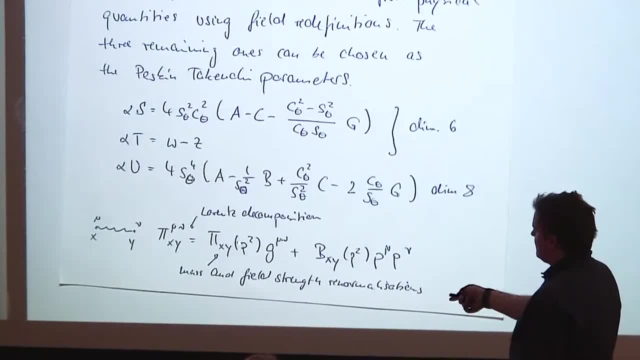 and you write the self energy and you do a normal Lorentz decomposition of it, then you get a g mu nu term, because there have to be two Lorentz indices. So you get a scalar function and you get a function that depends on p mu, p nu. 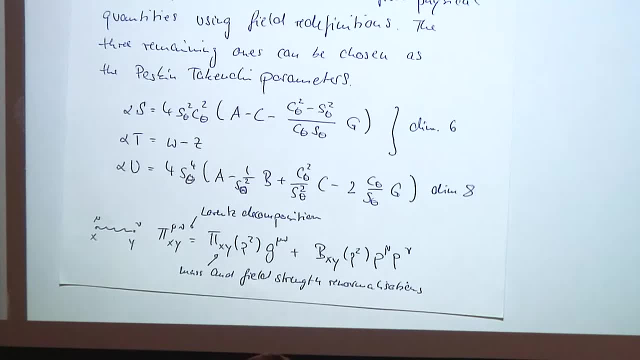 So we saw that these guys are typically related to gauge degrees of freedom. It's not really that important. so everything you need to calculate really is one loop diagrams to the z and the photon and the w and the z, photon mixing and you extract the prefact of g mu nu. 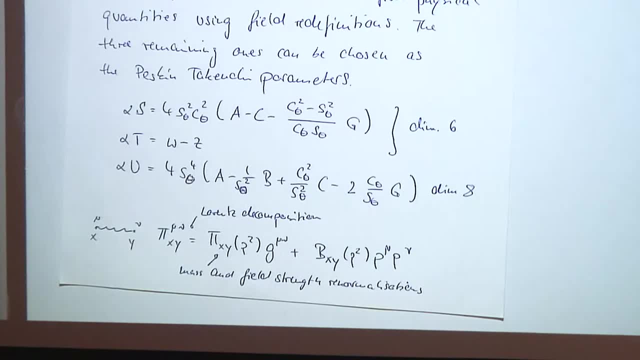 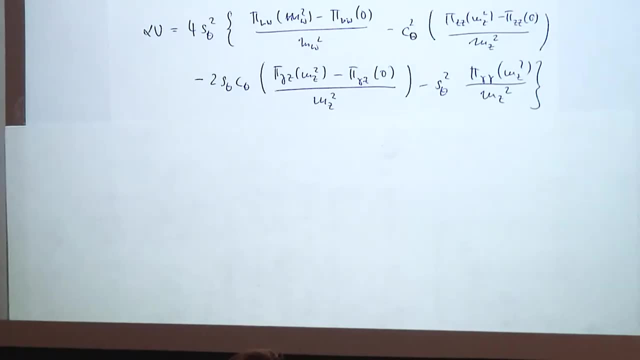 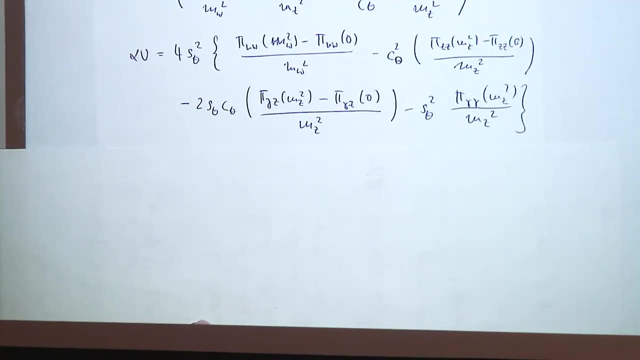 and you can calculate all of this very straightforwardly. Very straightforwardly in the sense that you have to put all of this stuff into an equation like that. But the good news is, you will code this up once and you can use it over and over again. 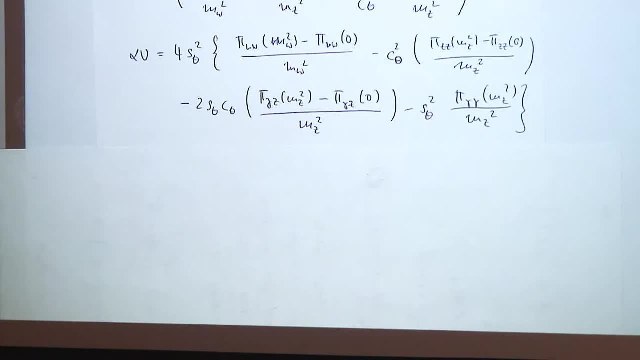 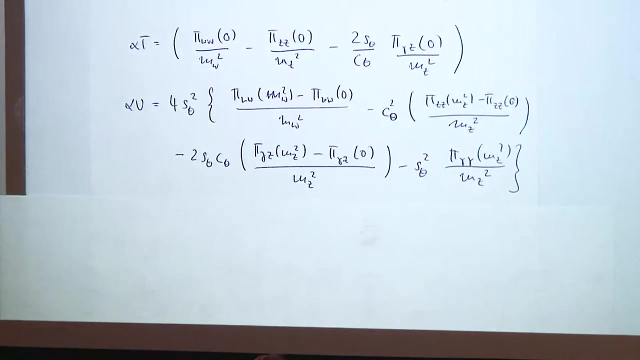 Now, of course there are ultraviolet singularities appearing here and there, but in the final result, because these things are related ultimately to experimental observables, they will cancel. So if you're not so inclined to do German physics, loops and renormalization and all of that, 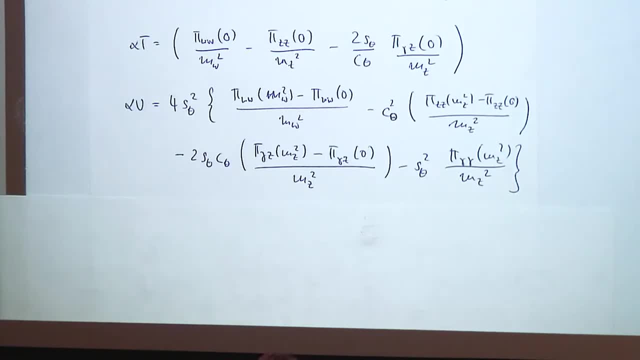 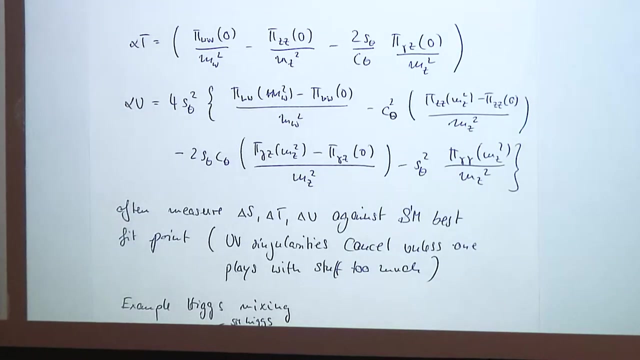 and you don't dig ultraviolet divergences, then this is an easy way around, because if there are any ultraviolet divergences left over, you've done a mistake. So it looks complicated, but it's fairly straightforward And typically when we do this, 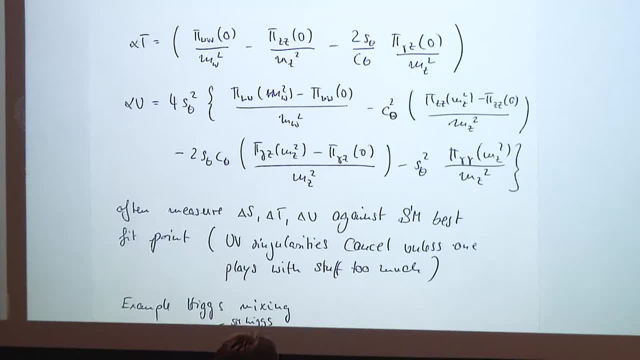 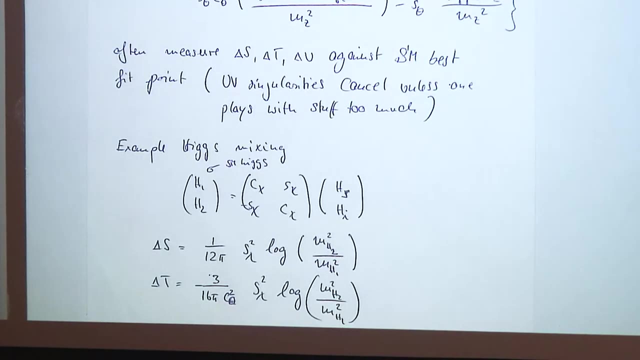 we relate it to the standard model itself and measure delta s and delta t and delta u against the standard model best fit point. So for example, in our singlet mixing scenario, just to give you the result, you get a contribution to the s parameter. 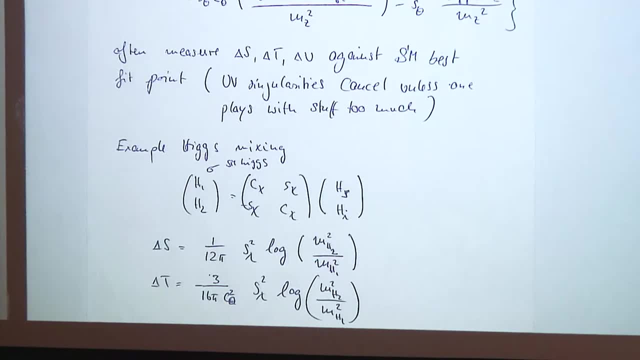 that looks like this and you get a contribution to the t parameter that looks like this. So it scales logarithmically with m h squared and in both observable delta s and delta t. So also when the mixing goes to zero, you see that you recover the standard model. 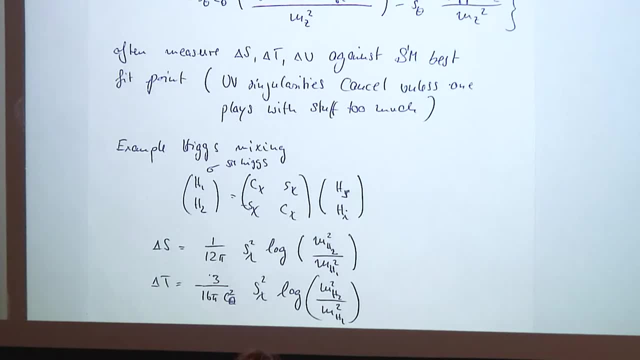 So s psi goes to zero, The top quark on the other hand. so I don't show you relations for that, but the top quark would enter here quadratically. So actually it's the difference between the top and the bottom quark mass. 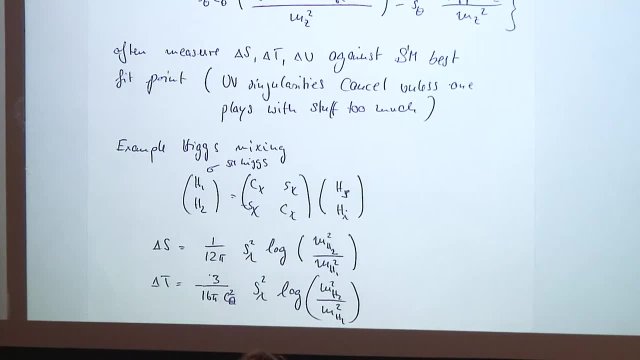 because that's also the source of chirality, which s ultimately measures and a violation of Castori law. So that's what we did with isospin, because we used phi, charge conjugate and phi to generate up and down quark masses. So we really make a difference here for the SU and 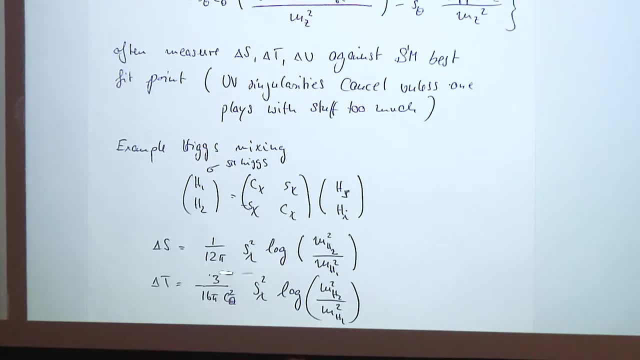 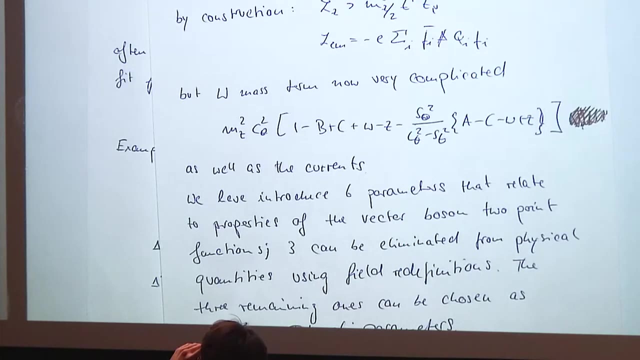 hypercharge breaks it as well. so you would get a contribution in the standard model here, that is g prime, proportional and logarithmically with the Higgs mass and then linear in the mass difference of m t squared minus m b squared. So that was quite heavy. 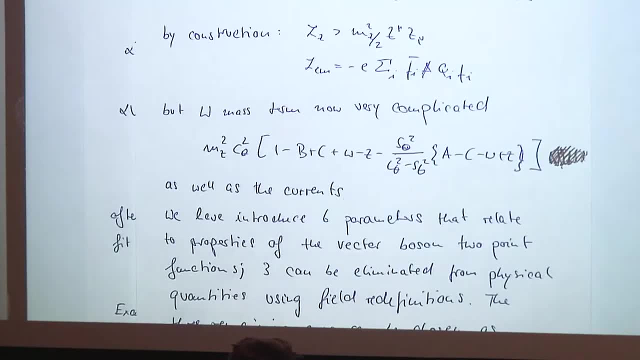 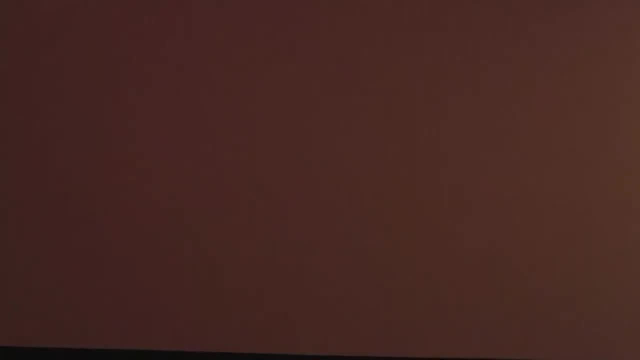 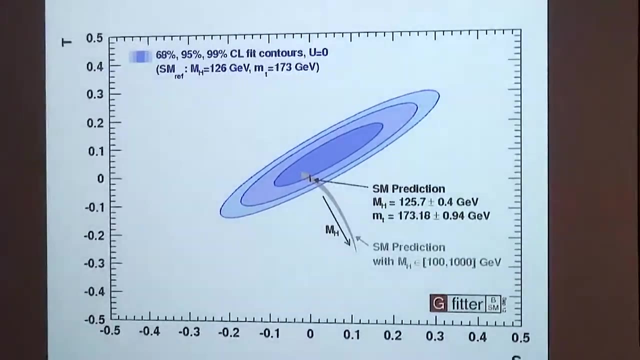 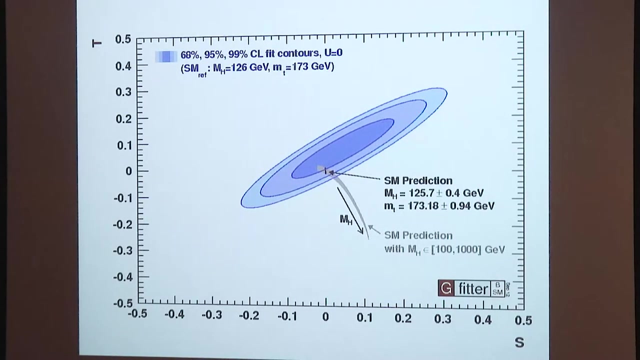 So let's have a look at if I can operate this, at how constrained these parameters really are. So I think that's input one. There you have it. So this is a German collaboration. g fitter: They do all the fancy electroweak physics stuff. 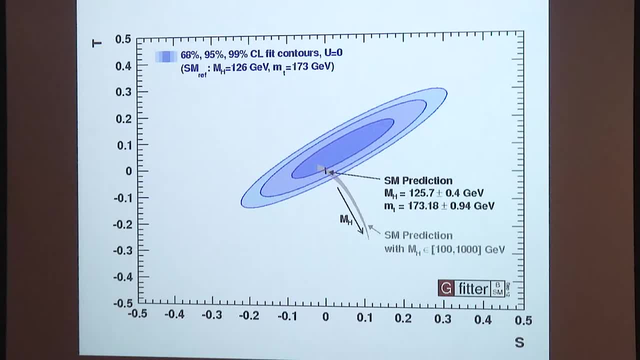 So they do complete electroweak fits using all sorts of stuff, you know, including corrections like this. But they also are nice enough to break that down to our beloved S and T parameters. So you can see that this is the ellipse, that is the left 68,, 95,, 99 percent confidence level. 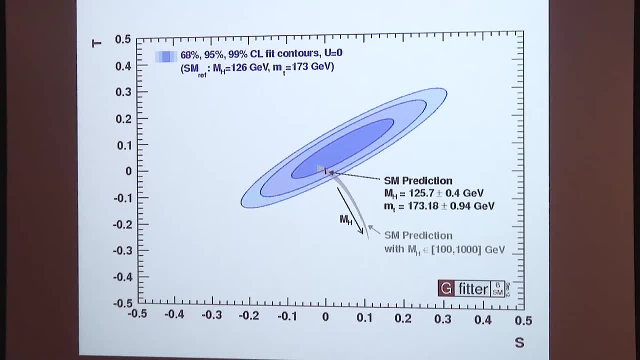 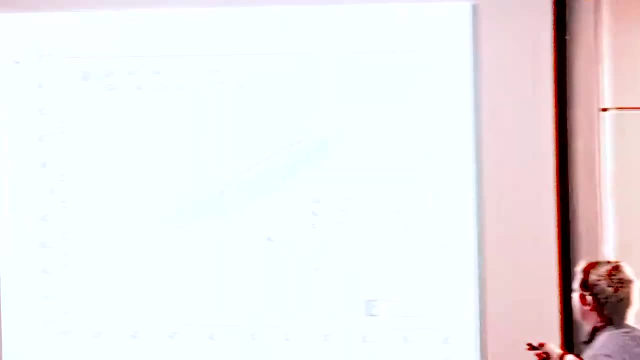 So the higher the confidence level, the more sure you are that you really covered the physically true point, And you can. we had this bound of 900 GeV right And you can see that this is really weird compared to what's happening here. 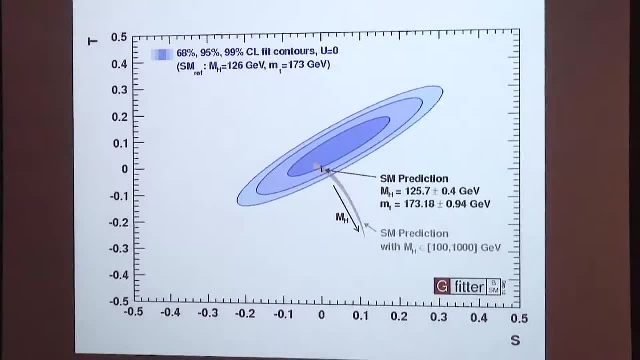 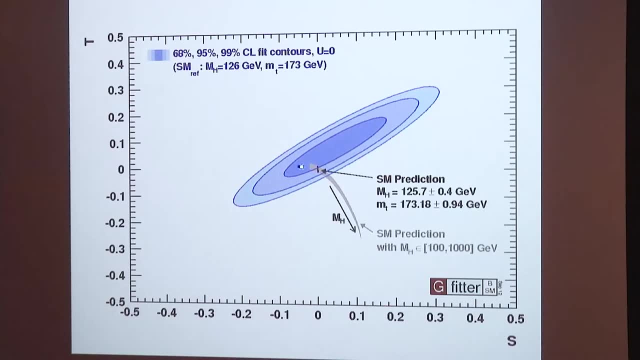 So this is from September 2012.. So this is shortly well, this is aligned with the Higgs discovery. So you can see that if the best fit point sits here and you slightly, slightly, slightly, increase the Higgs mass, you're outside 99 percent confidence level. 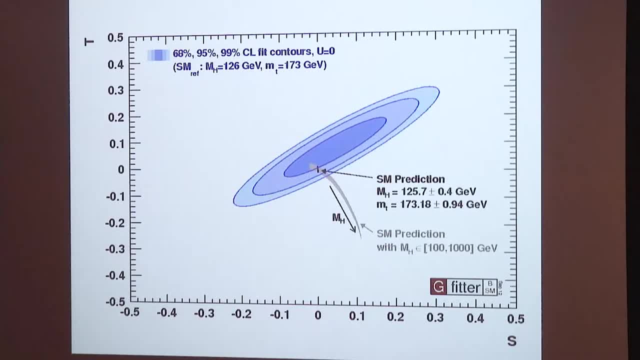 So this plot alone, after the top mass was discovered and its mass value was consolidated- because, as I said, this is a dominant contribution to S and T- this was really one of the most constraining plots that you could think of to constrain the Higgs in the context of the Standard Model. 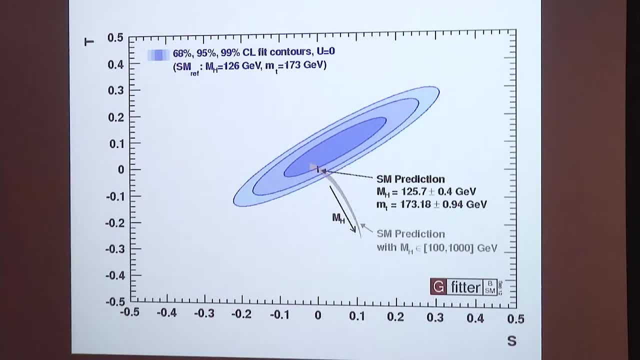 So 130 GeV Higgs was already ruled out in a way. But you know, people love this plot. These days maybe not so much anymore, but back in my days people absolutely loved it. Yeah, So usually these groups. 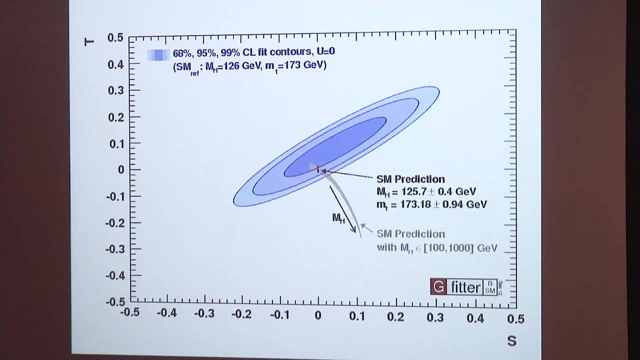 first of all, the U-contribution in our singlet model would be 0. But it's so in this fit it's set to 0 by hand. They also have stuff where they let U flow, But the naive power counting argument. 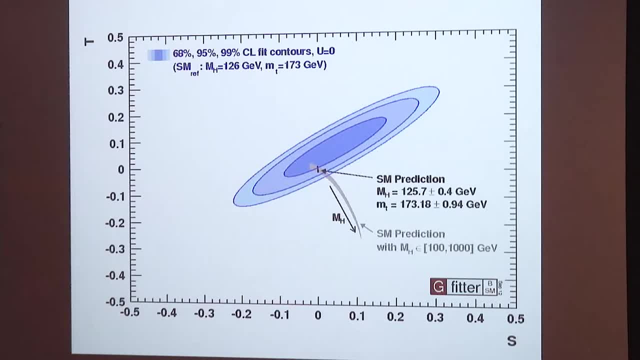 between S and T and U, you would expect S and T to dominate in terms of contributions. so this is a motivation to break it down into a nice palatable format for us theorists. So if you move out with the mix, you violate it very, very quickly. so our 900 GV unitarity. 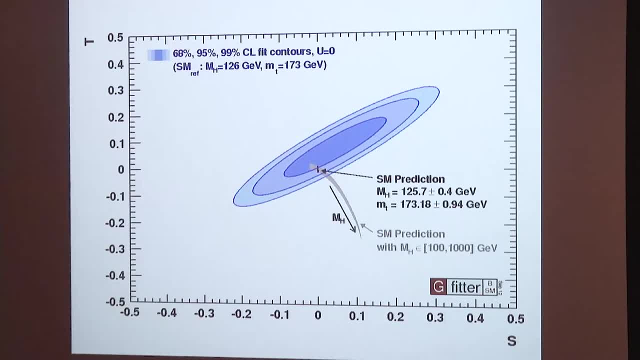 bound would sit here. so you see, this is completely disfavored by electric precision data. People like Tillman in the days they realized that, okay, you can actually get a positive contribution to S from the Higgs mass and a negative contribution to T, but if you throw. 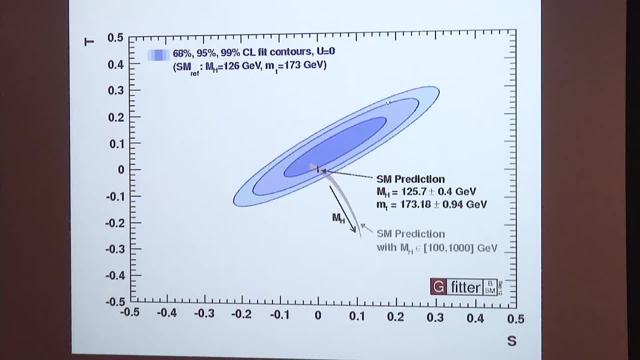 in additional fermions. if you're lucky enough, you can shoot yourself back into the ellipse up here, and this was the whole idea of introducing a fourth generation of standard model like fermions. Tillman can tell you all the details of how the PDG got it wrong, and so on and so forth. 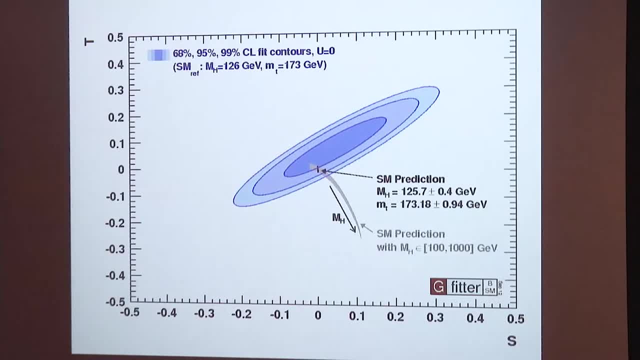 but now it's ruled out. there is no fourth generation because we now know that the Higgs production cross section does not allow for the presence of a heavy top quark on top of that. that would enhance the cross section quite dramatically and we've seen a cross. 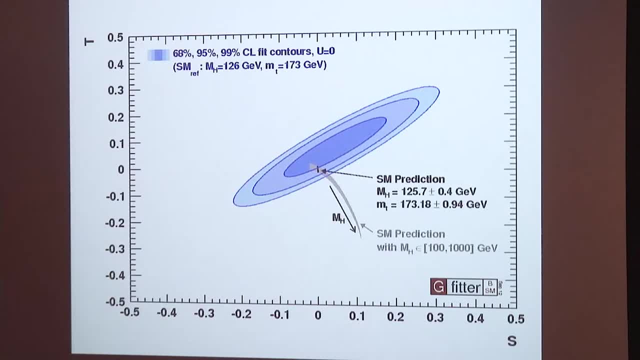 section. that is consistent with the standard model, so no need to worry about a fourth generation here. So are there any questions related to this? It's slightly smaller, but I think this already includes the Higgs mass, so the 125.7 plus minus 0.4, that has gone down a little. 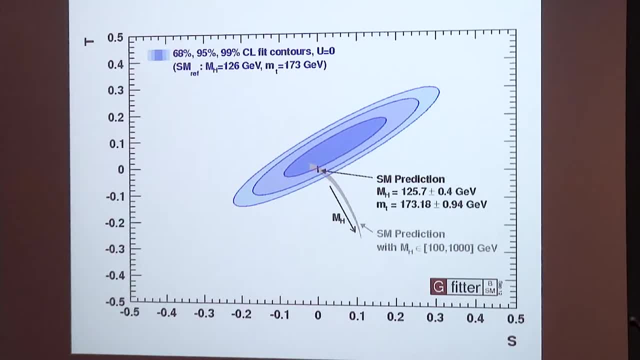 So this becomes more constraining, but not much has really changed. This is already super constraining. so I mean, if you write down a model has anything to do with electric symmetry breaking and you calculate S and T, you typically end up here or here, or here or here. so it's really, is it a kick in the bum? 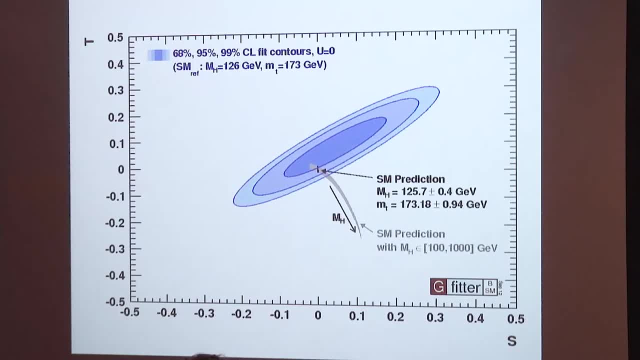 So, and this is also why you know you shouldn't mistake it for like just calculate S, T and U, and if you have a function where S and T is the absolute power we use, okay, So use this for those purposes. Pretend we have the higgs. 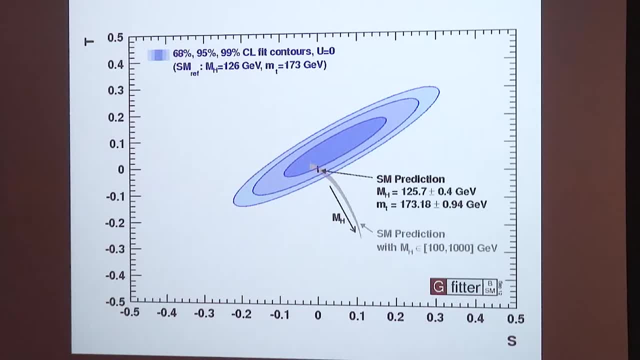 you and if you lie in the ellipse then you know you're fine. this is like it's the first step and it's an approximation to the full electroweak corrections. that includes the whole lot here. so you would call these oblique corrections because they appear universally in processes that involve electroweak bosons and the 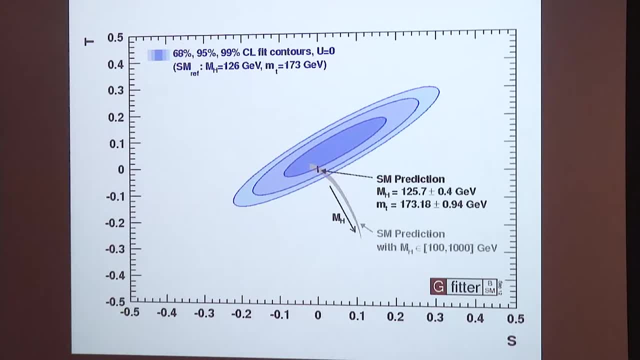 stuff that impacts, say, forward-backward asymmetries of peak quarks. at LEP we call them non oblique because they are really specific to to one particular particle and that's quite hard to work. it's hard to work that out, but typically we don't do this as phenomenologists. okay, so you look for S&T, make a scan. 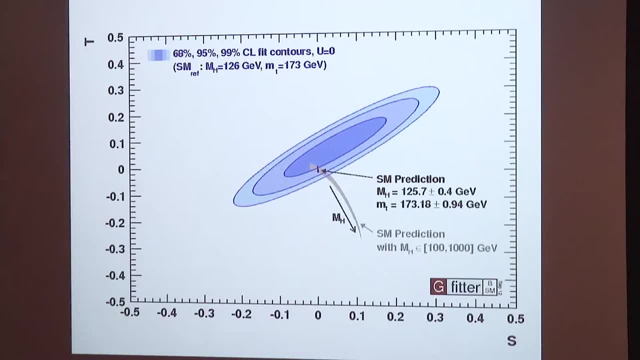 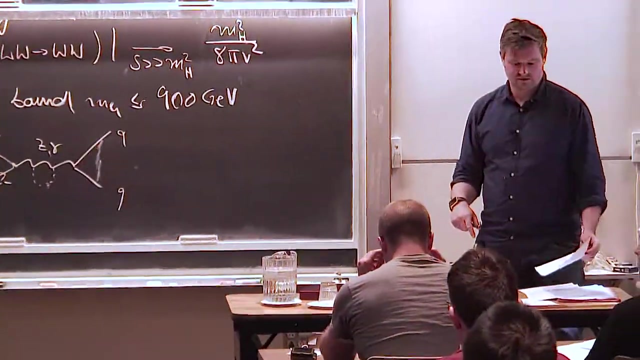 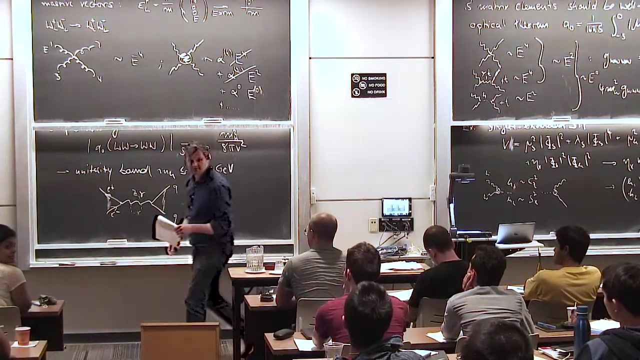 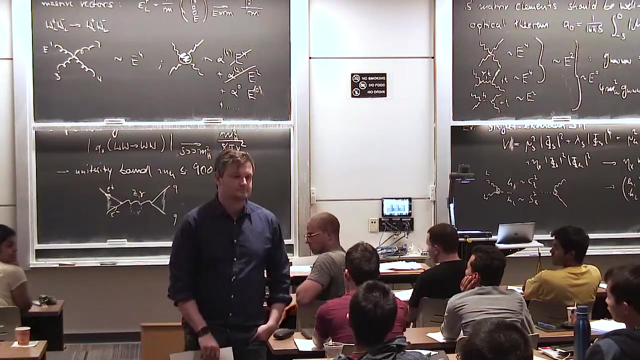 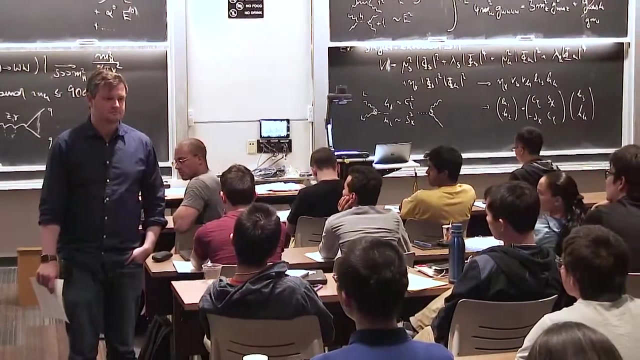 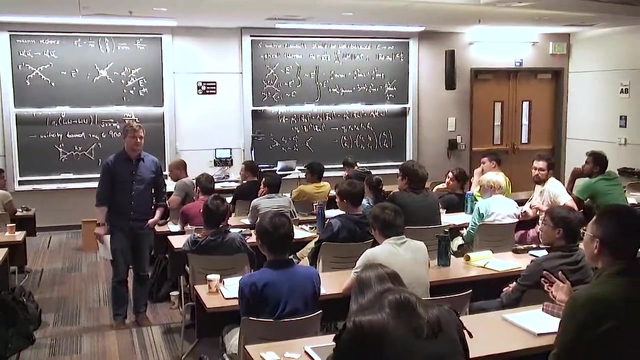 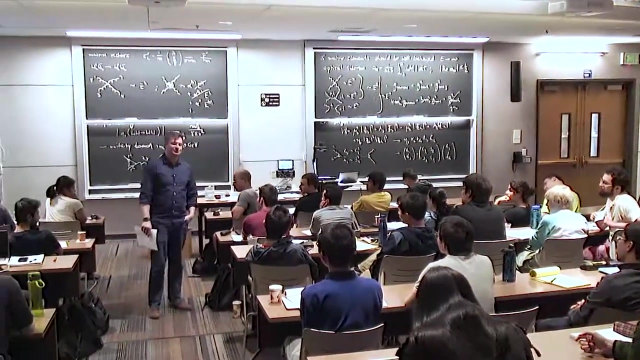 identify the points that fall into the 99% confidence level, contour and then you write the paper okay and leave the hard stuff to people who have more time and more patience. yeah, any other questions? no, yeah, yeah, I don't quite know how to answer this, apart from you have to do the. 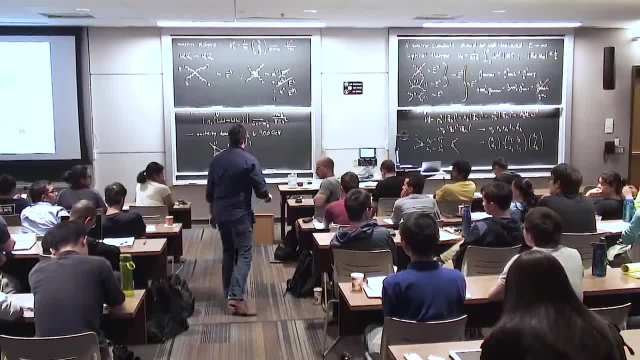 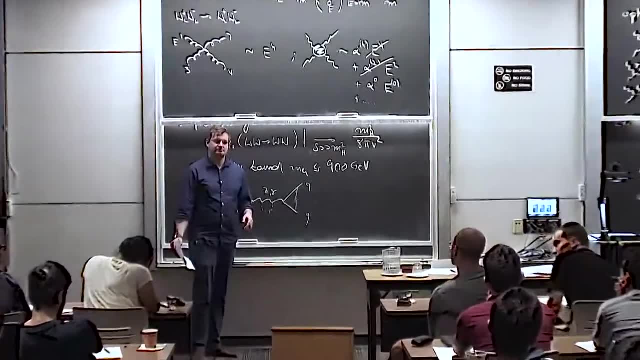 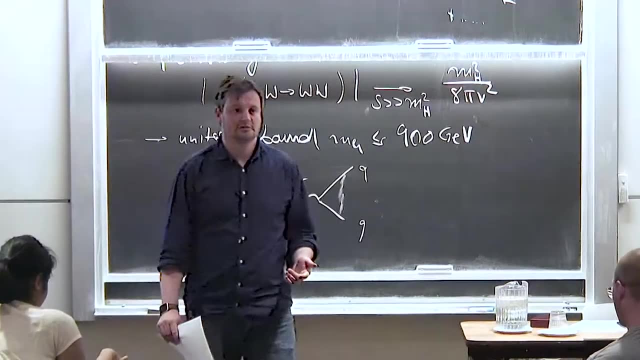 calculation, but the that, the Feynman diagrams that enter here. I don't quite know how to answer this, apart from you have to do the calculation, but the, the Feynman diagrams that enter here. yes, that's right, yeah, yeah, yeah, yeah, yeah, yeah, yeah. so the S&T parameter logarithmically. 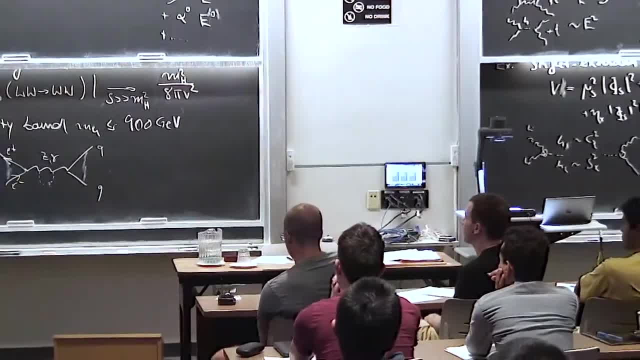 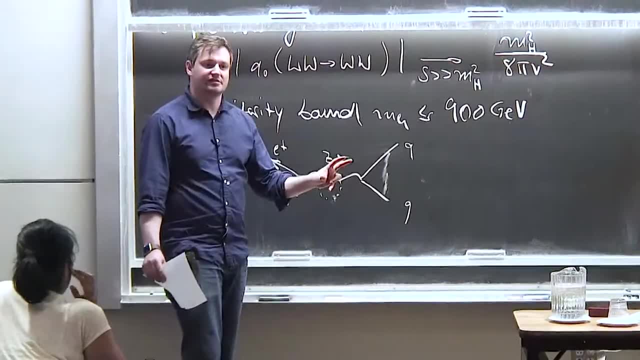 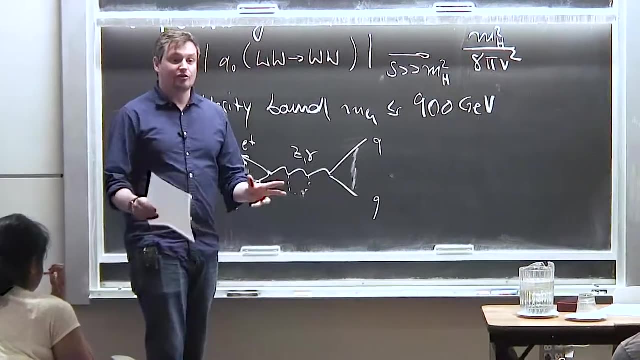 sensitive to it, to the Higgs mass. these diagrams here wave function corrections. they're always related to B functions in the Pasarina-Weltmann type of approach and these are logarithmically dependent, dependent on the masses. So if you look at the two-point function and the Feynman diagram, 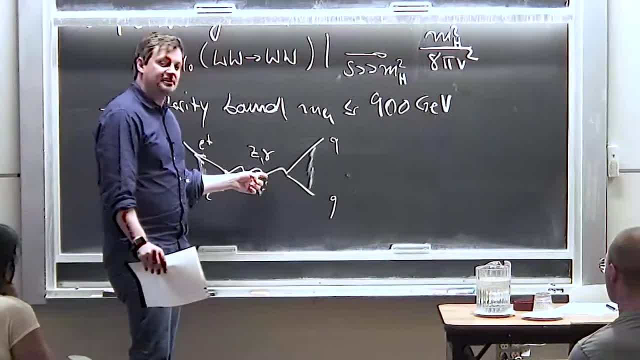 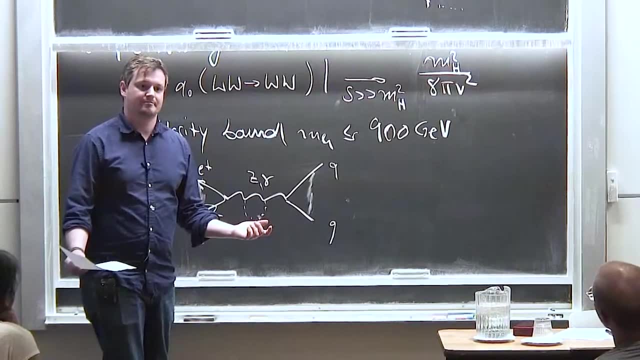 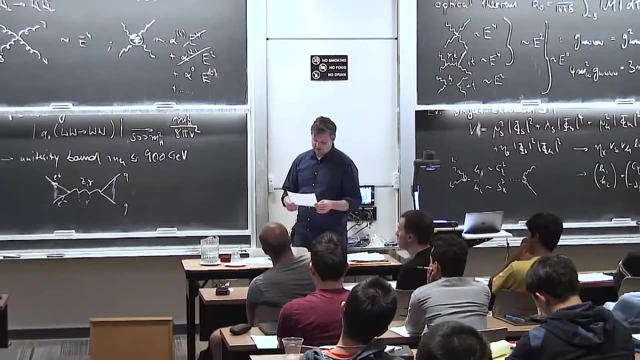 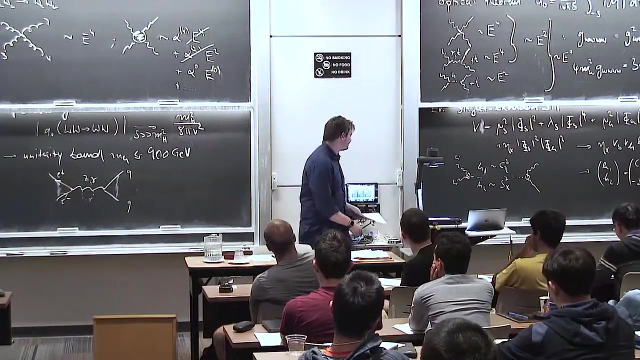 you translate this into an algebraic expression, you'll see that this will be logarithmically dependent, And this is a statement that we're living in four dimensions. really, Okay, how much time? Fifteen more minutes, Oh, tough, tough here the afternoons. 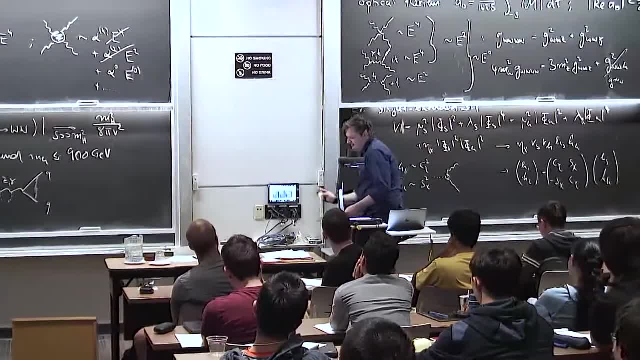 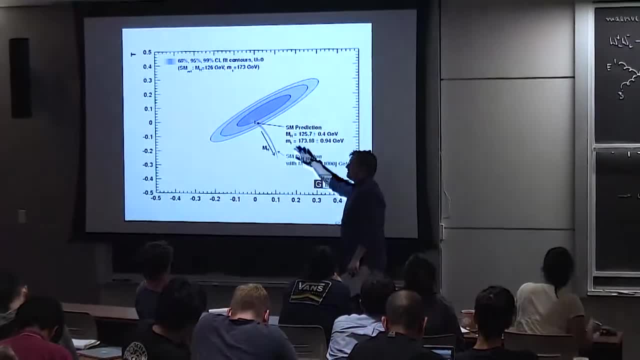 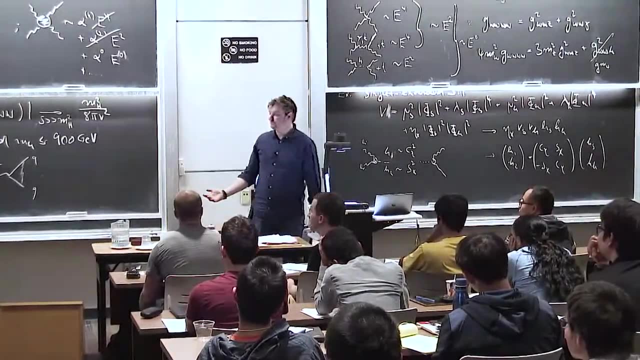 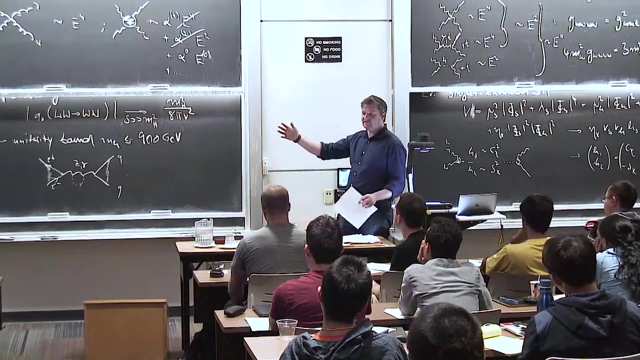 Let's do something nice at the end, okay? So now we know that 125 GV is actually quite nice, But are there any other constraints that might come around when we actually have 125 GV? So you know, this plot tells you that 125 GV Higgs in the light of everything that you can expect. 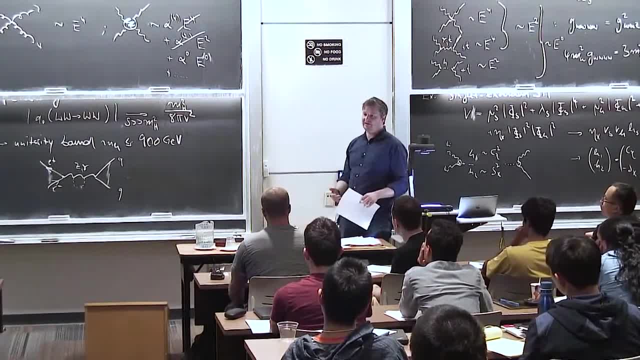 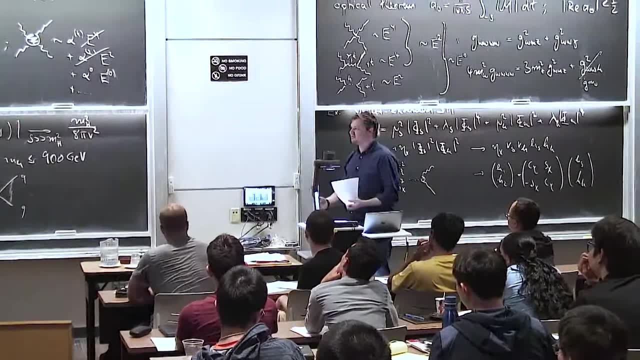 from lab measurements and so on and so forth is pretty much bang on. So we don't seem to have a problem with the Standard Model as such. you know, apart from the obvious shortcomings, you know no dark matter, et cetera, et cetera. 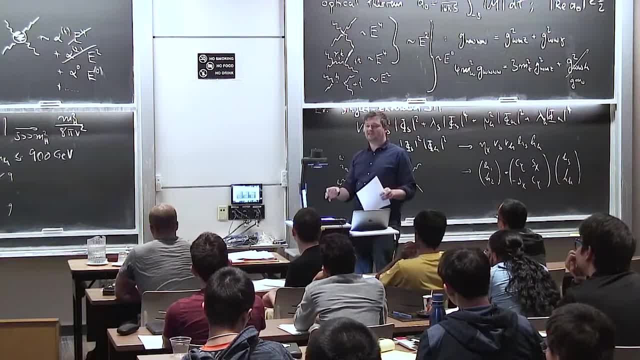 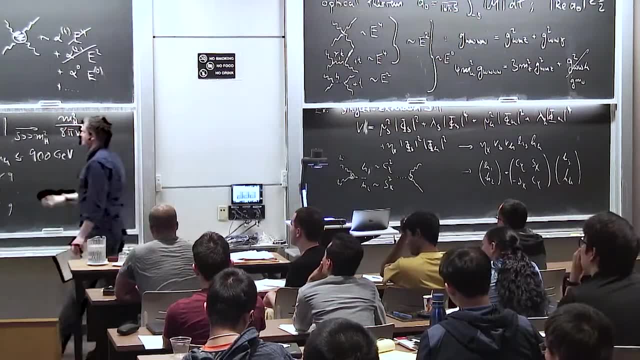 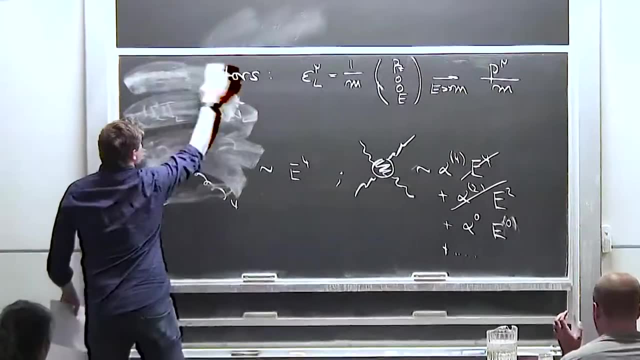 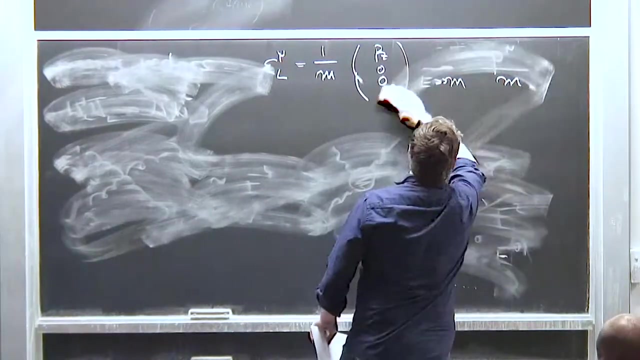 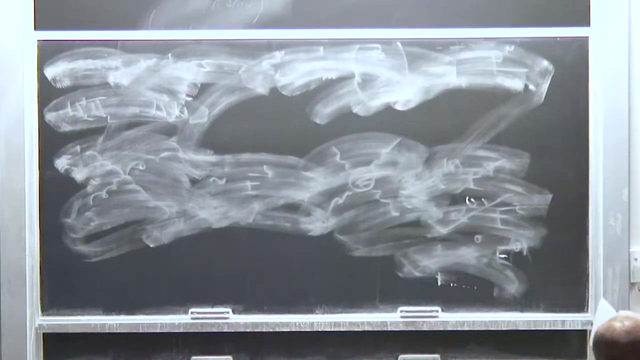 But are there any conceptual shortcomings of the Standard Model itself? Because that looks like everything seems to be nice in place. So let's have a look at some other constraints that relate to the evolution of the electric sector to high energies. Right, so none of these parameters in the Lagrangian are really physical? 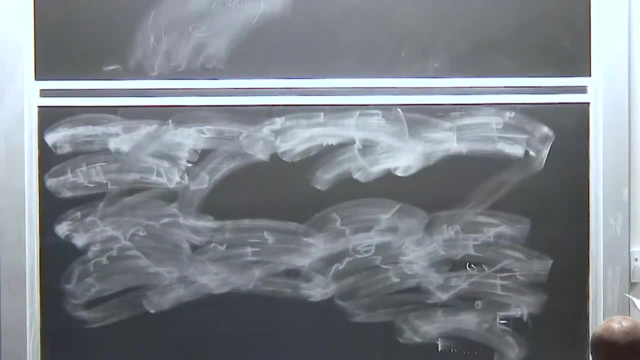 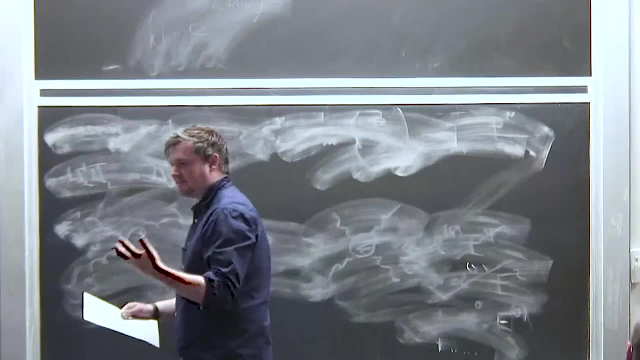 but the whole process of renormalization allows you to fix their value through a measurement at one scale and then infer their value at a higher scale just through RGE flow, and you can calculate this from perturbation theory. So if you do this, for 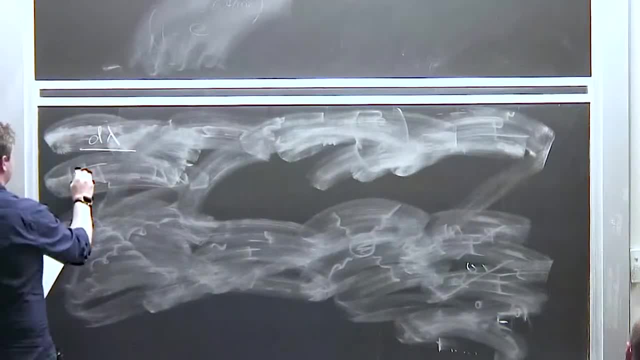 the self-coupling. if you do a d log Q squared, where Q squared is a renormalization scale that you can translate into a physical external momentum scale at fixed renormalization scale through the Kellen-Szymanski equations, then in the Standard Model it looks like this: 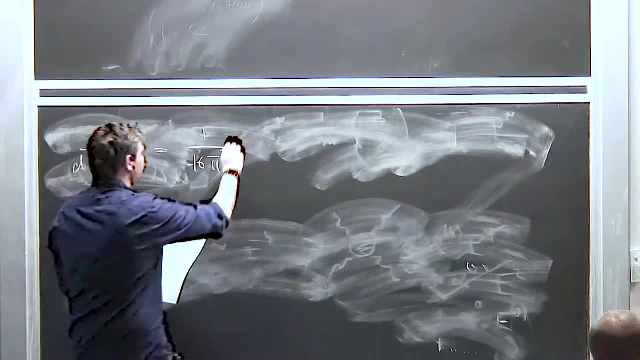 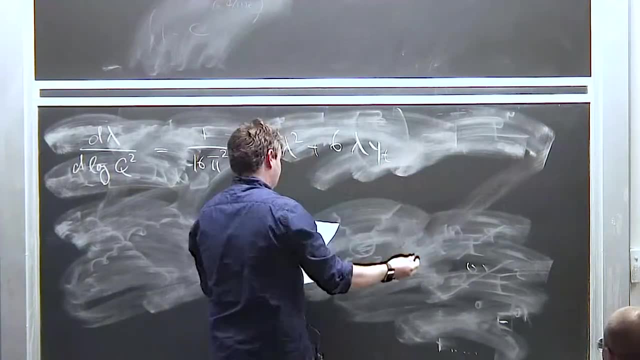 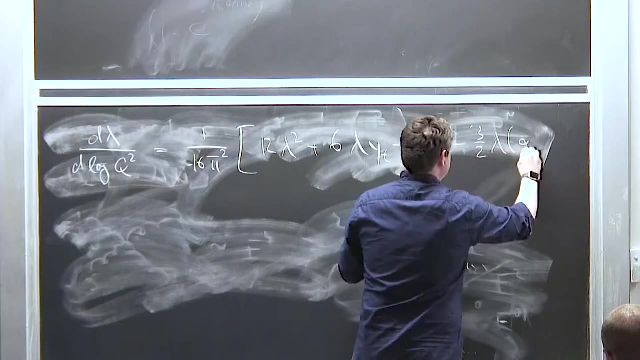 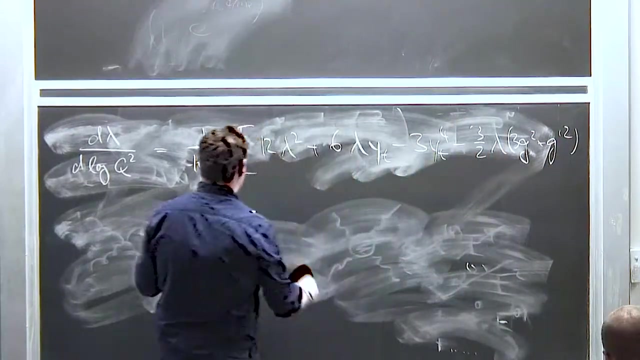 at leading order, so at one loop It's a 12 lambda squared plus a 6 lambda y top minus a 3 y top to the power of 4 minus 3 half lambda 3 g squared plus a g prime squared plus a 3 divided by 16. 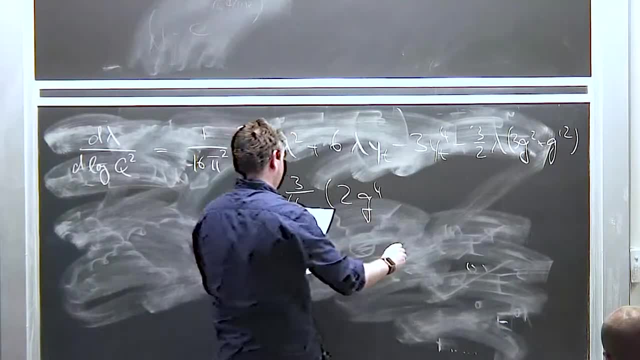 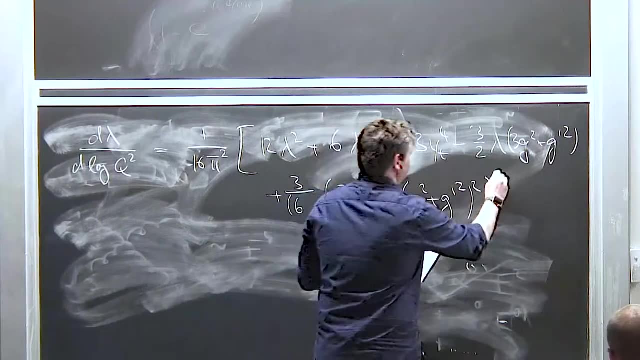 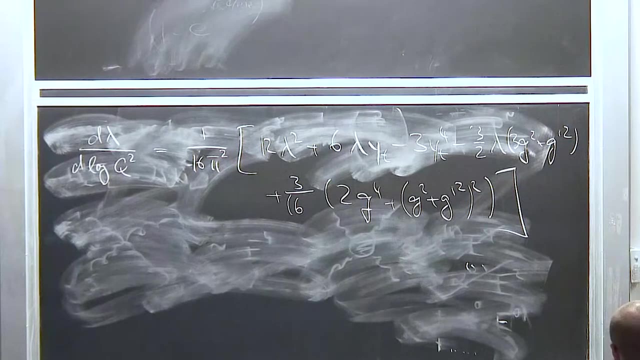 2 g to the power of 4, plus a g squared plus a g prime squared squared and big brackets. So in order for the Standard Model Higgs sector to be well defined, up to arbitrary energies, really we want a stable, it has to have a stable vacuum configuration. 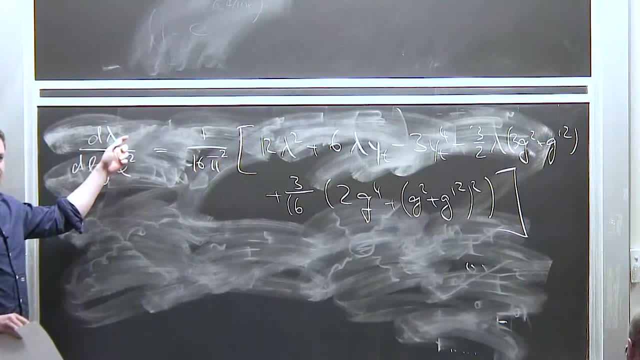 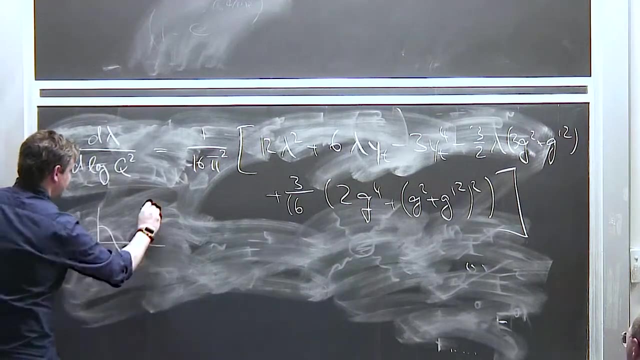 So remember that this scale defied to the power of 4 term and we have to have that positive, Otherwise we just fall into a potential. well, So if the potential that we calculated looked like this, so we really needed lambda bigger than 0 to be trapped here. 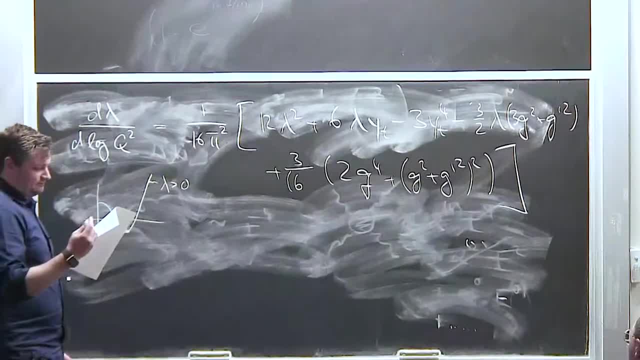 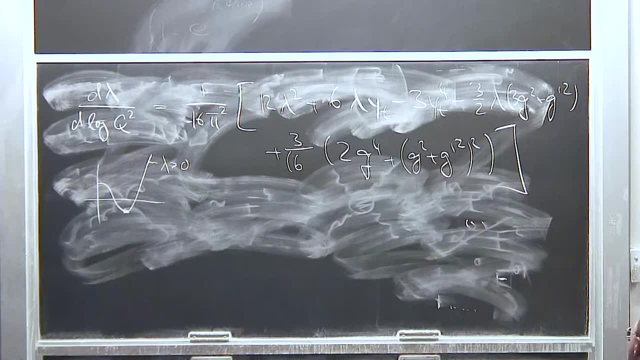 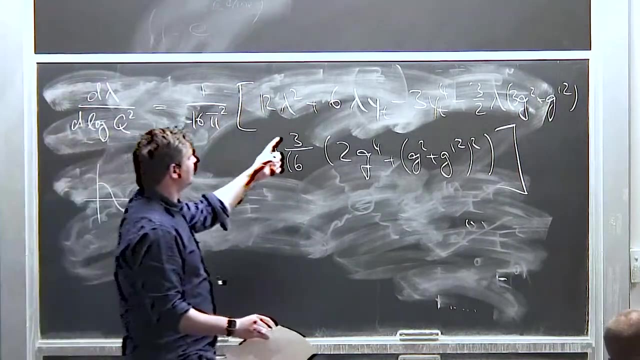 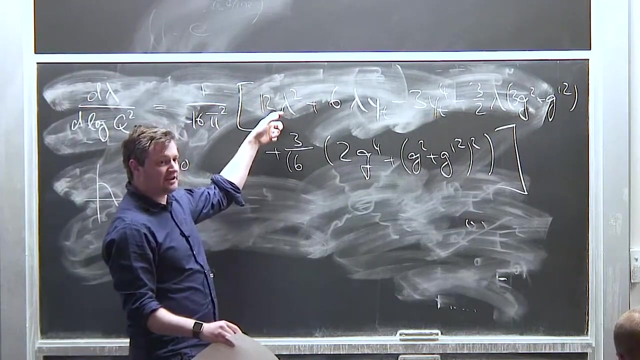 So now let's look at this RGE equation here for different scenarios. So in the first one is that we look at the case where lambda is actually large. When lambda is larger than all the other parameters that sit in here, then this term will dominate the RGE flow at large lambda values. 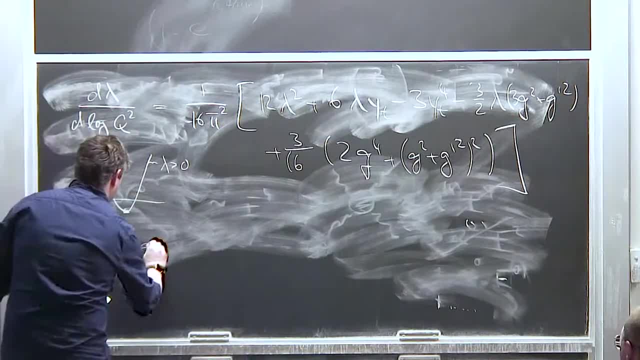 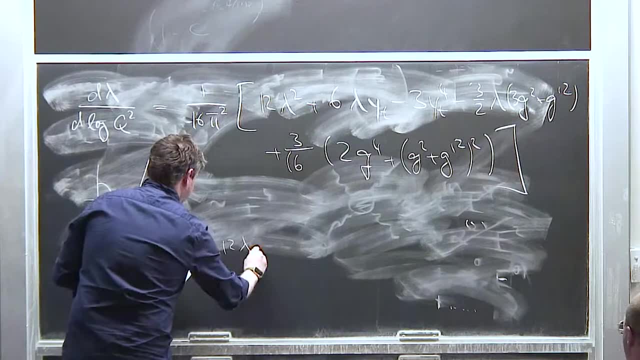 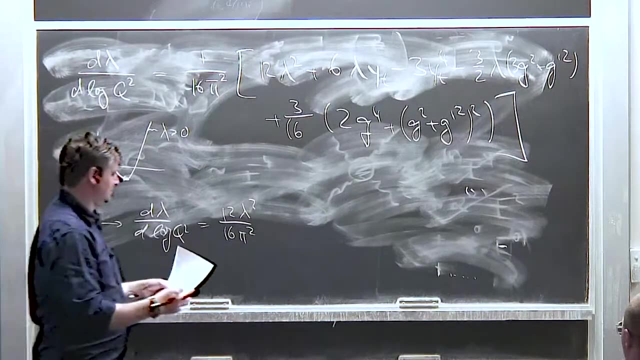 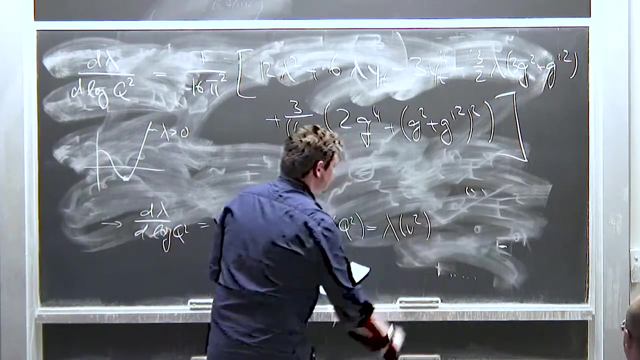 If you do that, you get d lambda by d log squared. q is a 12 lambda squared divided by 16 pi squared. So you can solve this and you get a lambda of q squared It's equal to lambda of v squared. So we fix it at the electric scale. 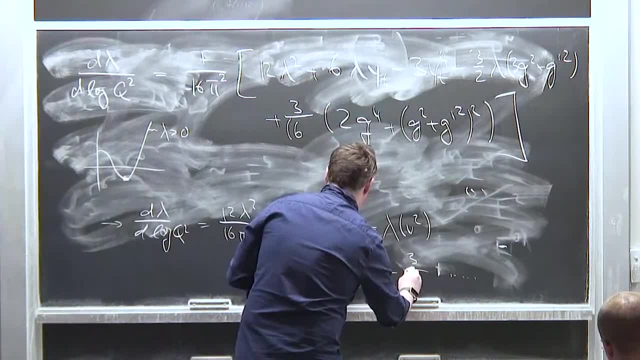 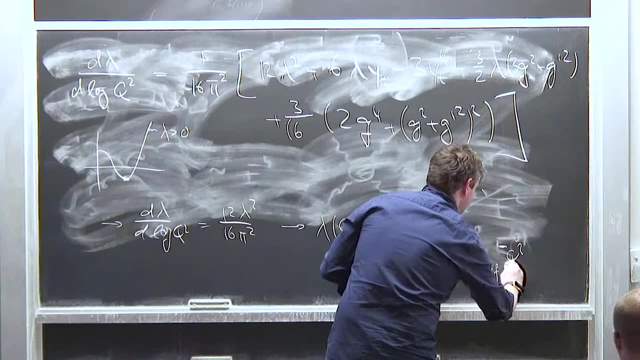 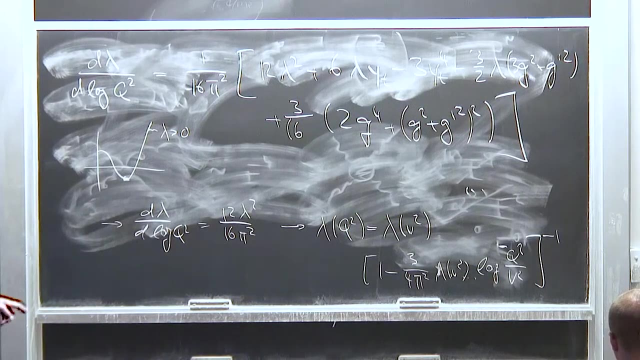 and you multiply a 1 minus 3 divided by 4 pi squared lambda at v squared times the log of q squared divided by v squared minus 1.. Okay, So you can see. You can see that if you evolve this now to high enough scales above the initial condition, 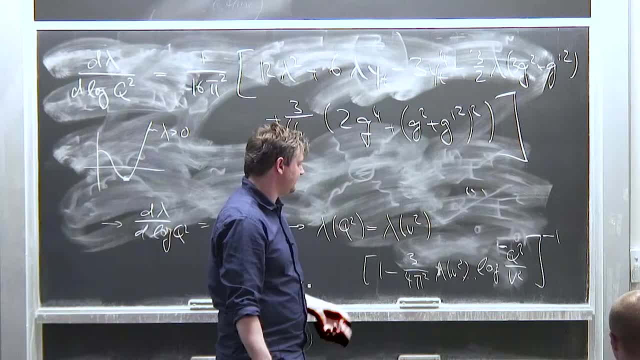 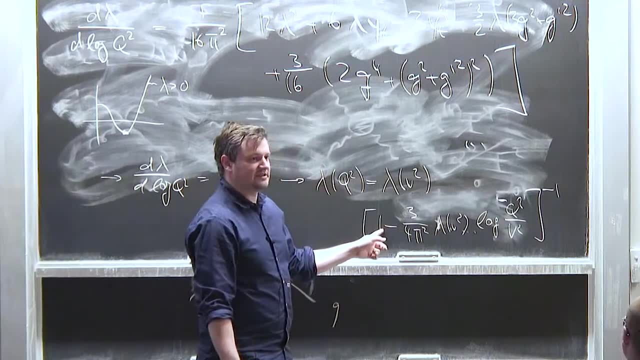 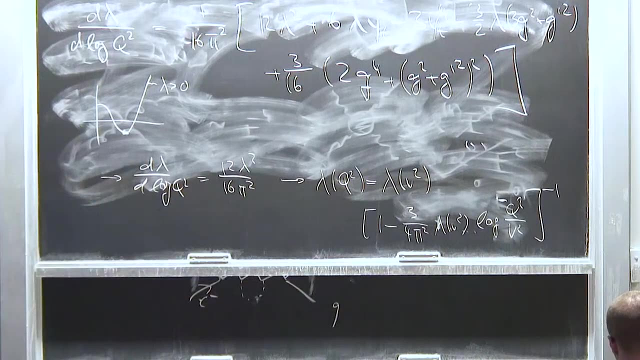 that we feed into the system at the electroweak depth. this becomes a positive number, And if that number becomes big enough, then you can get this equal to 1 here. So you hit the Landau pole, which you want to avoid, because then something else is to happen. that is not the standard model. 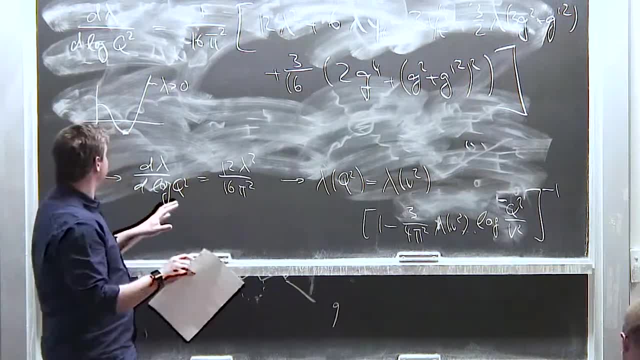 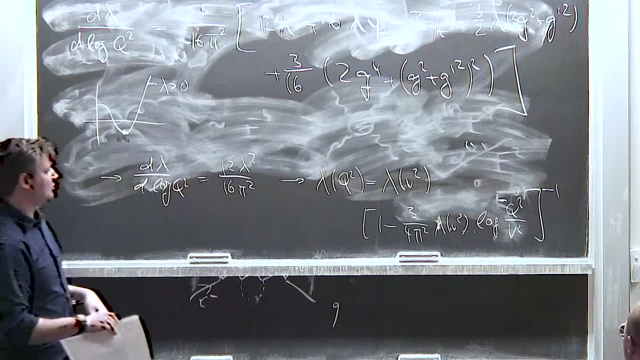 And if you want to have the standard model as we know it in terms of this picture, to survive to arbitrarily high energies or the Planck scale, you have to require that this Landau pole does not appear before. Okay, And because we saw that the Higgs mass is related to lambda. 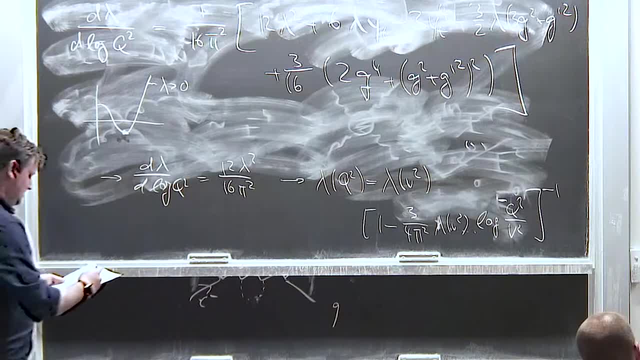 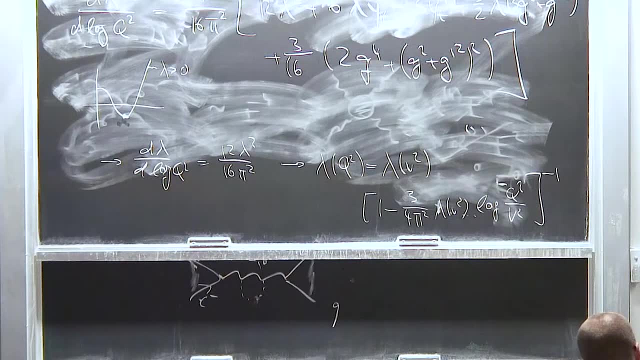 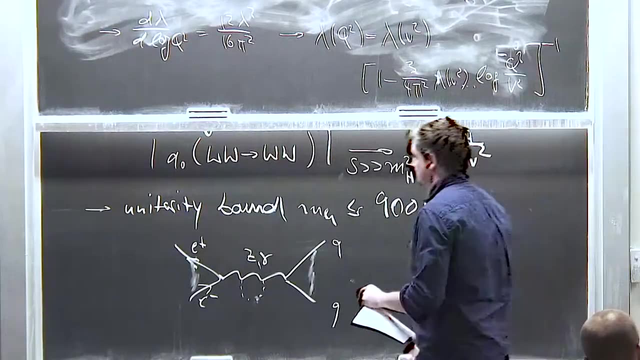 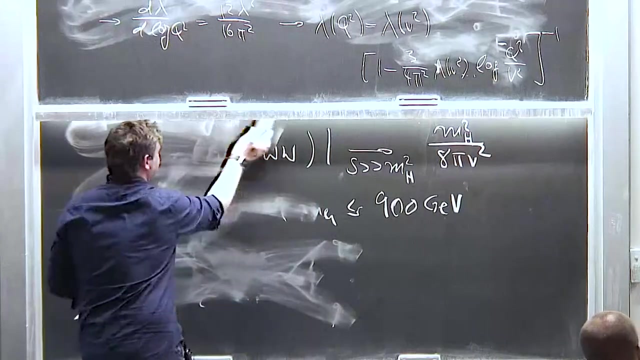 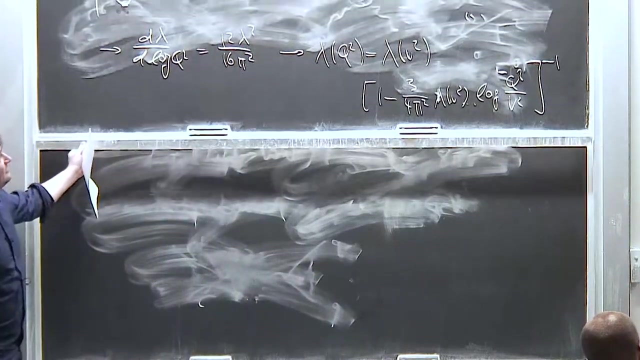 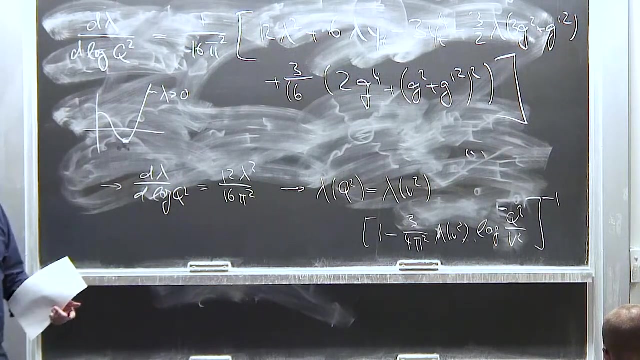 this sets a constraint on the Higgs mass itself, Yeah So, and it sets up a limit on m h, Also important. we know that it's the top Yukawa coupling, because that's of order 1.. The top mass in units of wef divided by square root of 2 is roughly 1.. 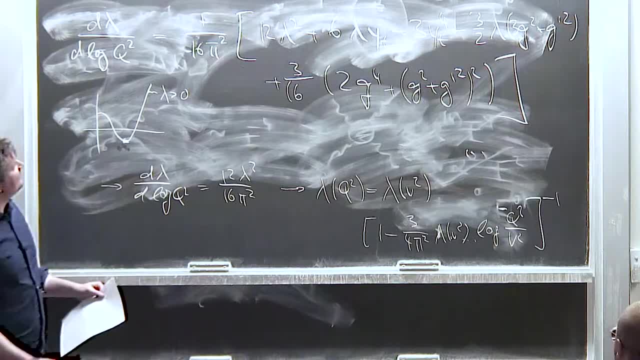 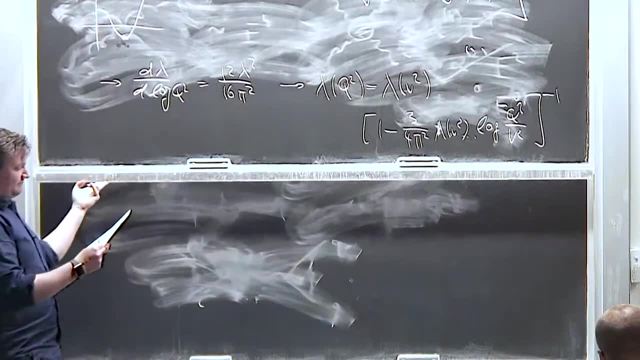 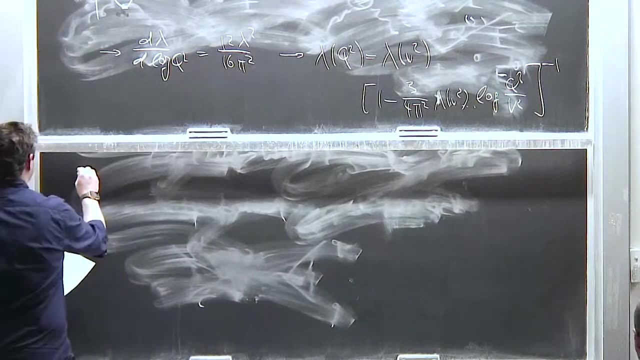 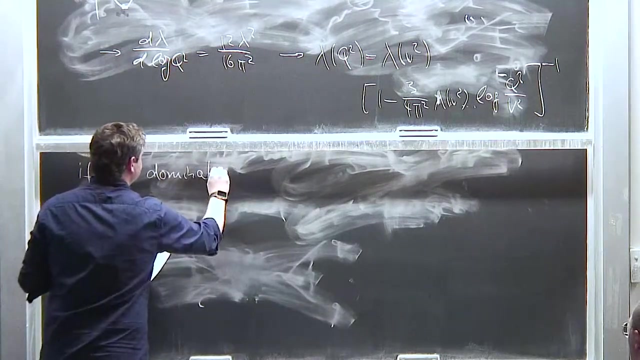 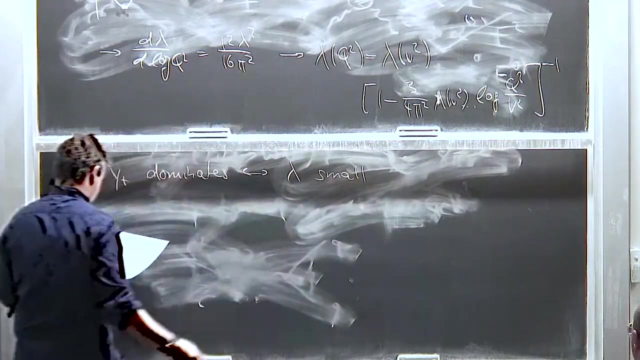 Okay, So this is quite a big parameter as well. So, and it has a negative sign because of Fermi statistics. So for small lambdas now. so if y t dominates, so this is in regions where lambda is small, you get a. 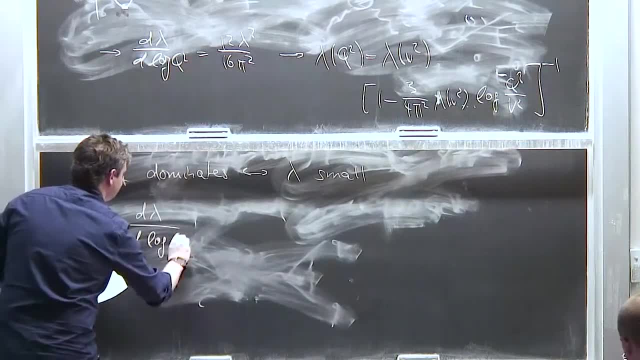 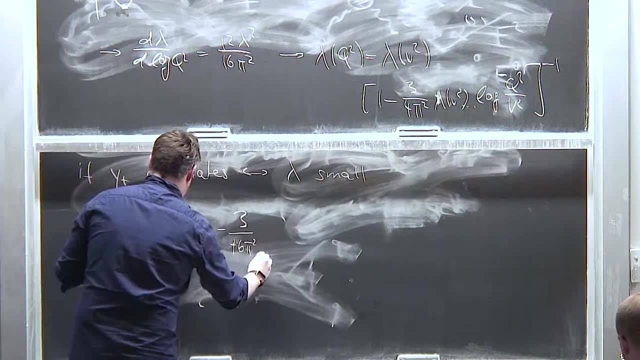 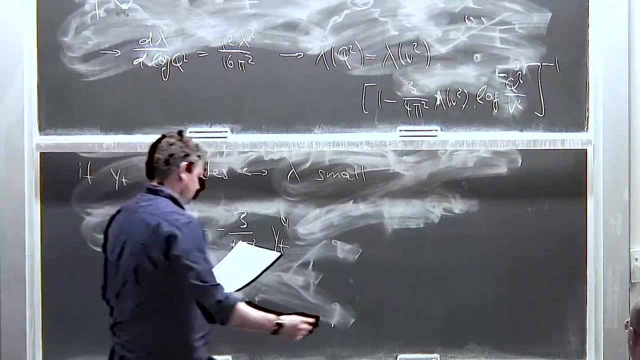 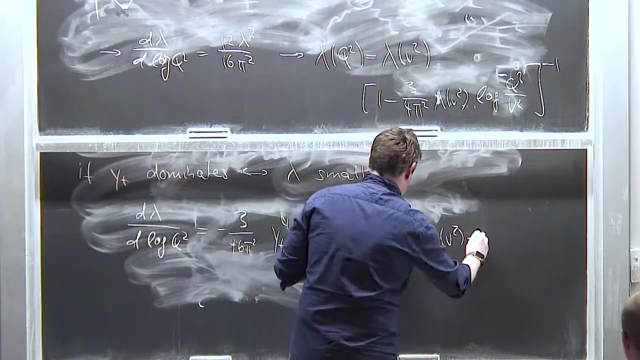 running of lambda d log, q squared, equals to minus 3 divided by 16 pi squared, times y top to the power of 4.. And this is an approximate solution that you get lambda of v squared minus 3 y top divided by 16 pi squared. 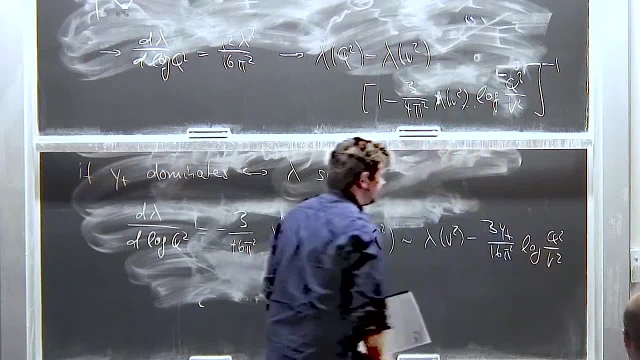 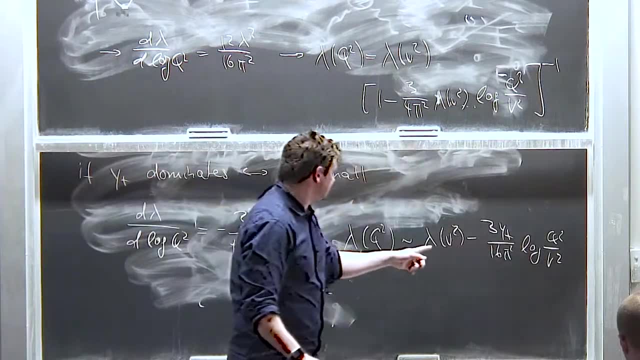 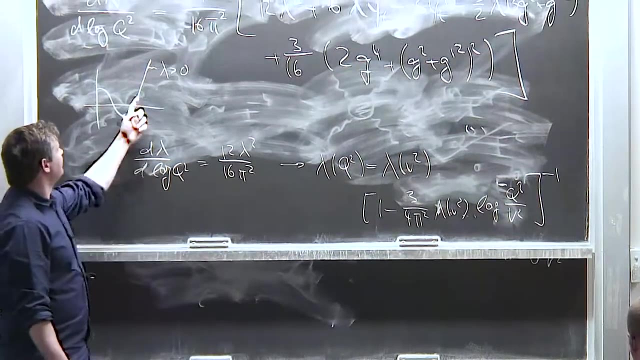 log: q squared divided by v squared. And again you can see that if you go to high enough energies you can actually change the sign in lambda. Okay, And then at high enough energies this would just fall over and you would not live in a stable vacuum configuration anymore. 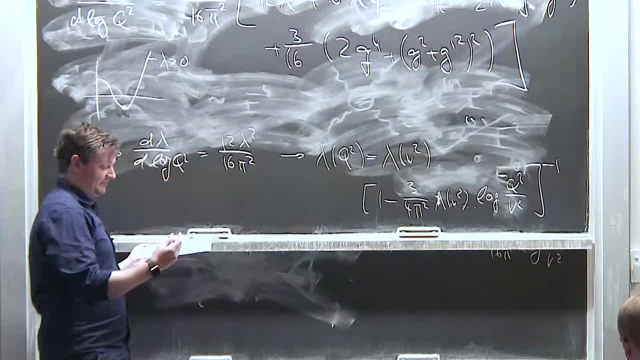 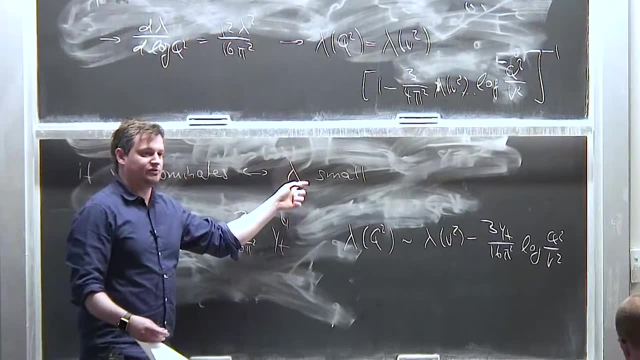 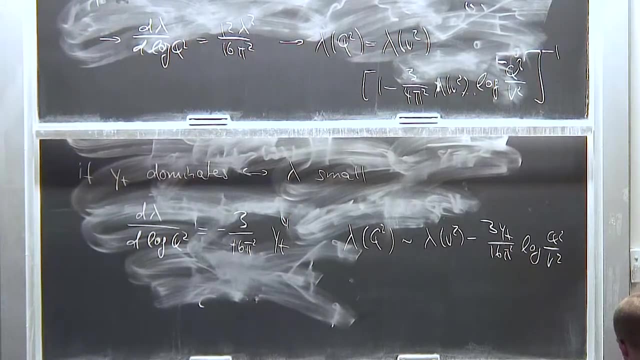 Okay. So these that sets a lower limit on m h. a lower limit on m h because lambda has to be small, ie the Higgs mass has to be small. So these guys are called the vacuum stability bound and the triviality bound. 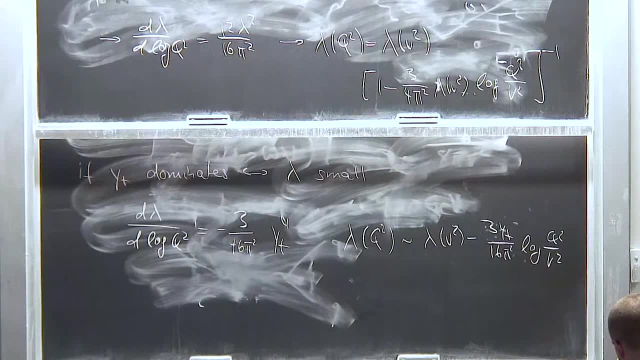 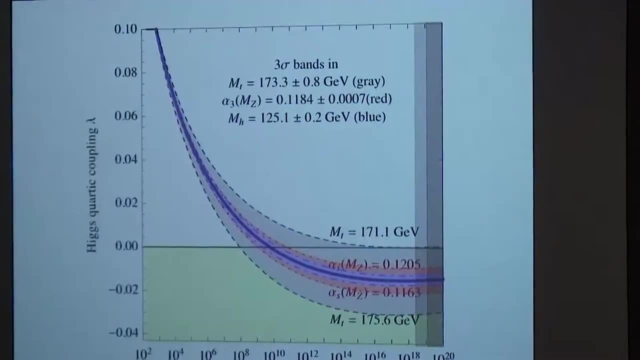 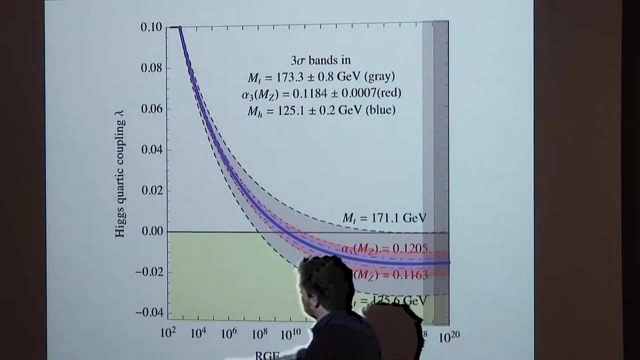 And people have looked into this in quite some detail. So this is actually going one order higher in perturbation theory. So it's really next to next to leading order, quite cutting edge. And this is the exported coupling and you evaluate it over a whole range of scales. 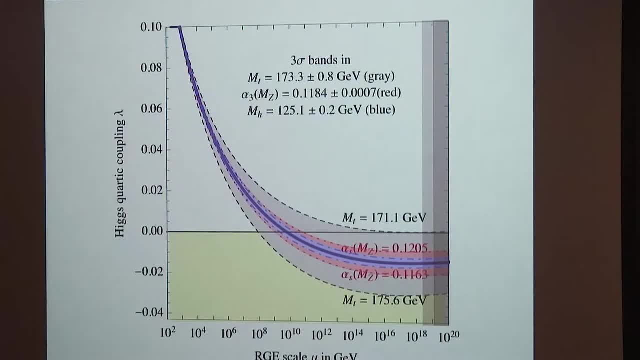 and you fix all input parameters at the weak scale to be like the stuff that we see, And indeed we see that for large enough values you actually dip into the negative regime of the potential. So this starts to bend over And we are not really. 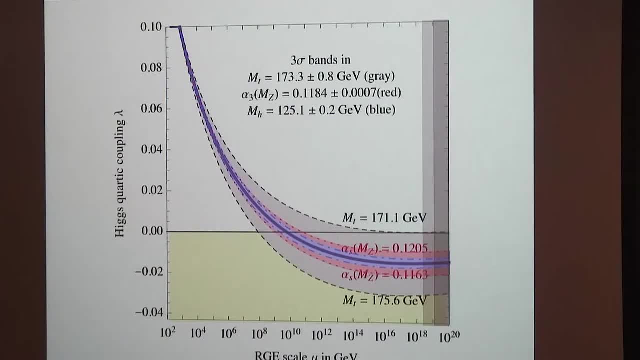 in the true vacuum anymore. Okay, And you can see also that. so the width of this band relates to uncertainties in the input parameters, m, top and alpha strong at z mass, and so on and so forth. So if you now translate this into into a plot that tells you whether we should 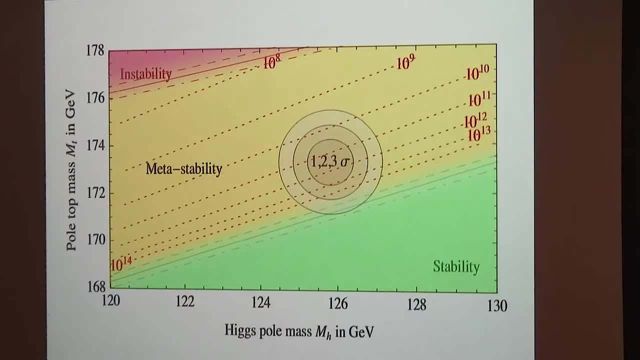 be having this conversation or not, meaning that we actually should be tunneling into a new vacuum. that would have quite violent implications. And you can see that actually the parameters are such that we live in a region that is characterized by meter stability. 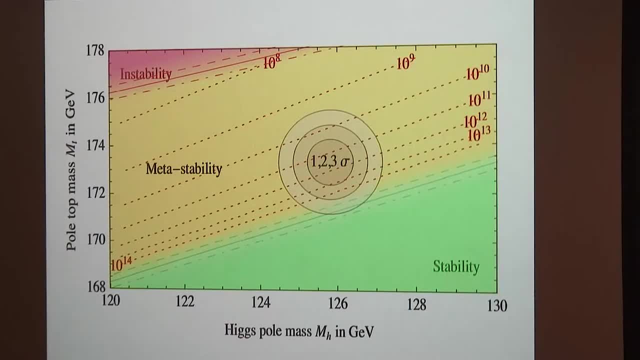 So where things can decay, but you know it's not super, super likely, Okay. so much longer decay lifetime expectations than the lifetime of the universe, Okay. so essentially, this calculation you can do with a WKB approximation, And so we are away. 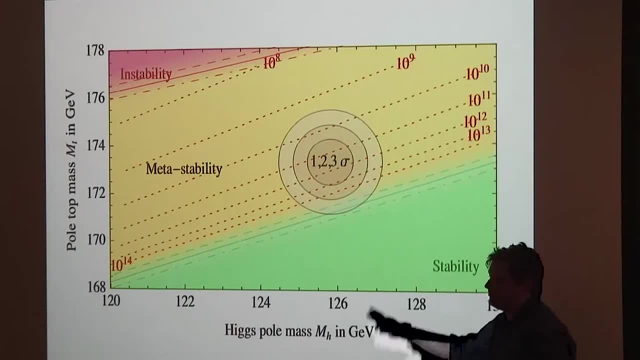 at the three sigma level from the stability region, But obviously otherwise you wouldn't be talking to me. We are not living in an instability region. Yeah, They are. they just refer to how far you extrapolate this. So it would be like the q squared max on. 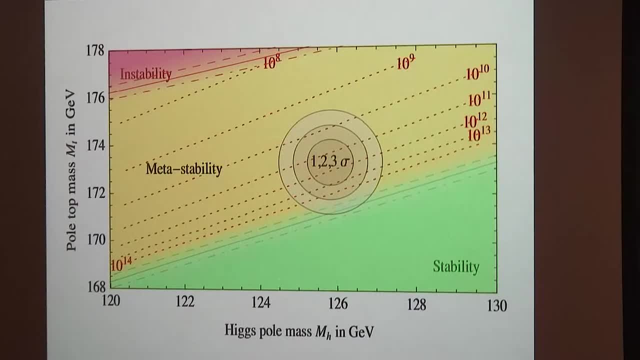 the other plot. All right. so this tells you that somehow we in the standard model, we are quite in quite a delicate situation. Okay, So if you look at this in a, in a blown up picture where we scan a little bit further, 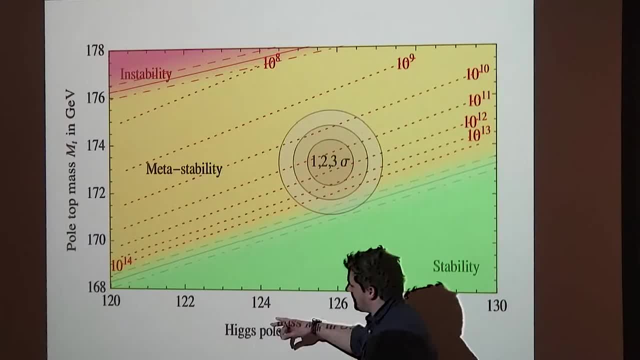 over the Higgs mass and the top mass. you can see that this is really a tiny end point in the between the stability region and the and the and the instability region. So therefore, these, these are the, of course. 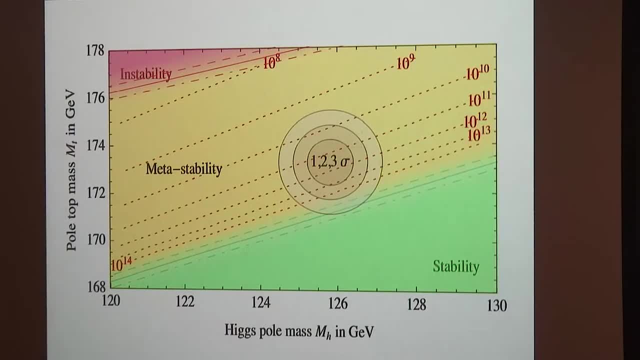 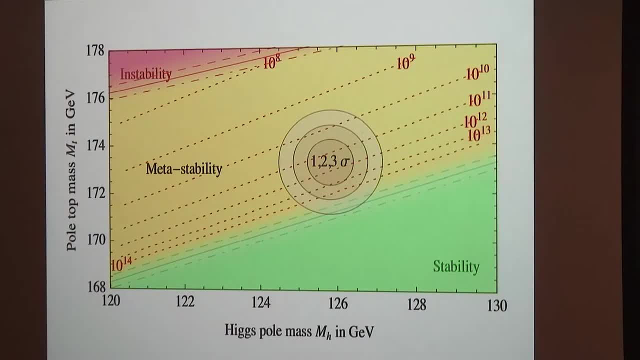 There is no new thresholds between the vacuum ex, between the Velyf scale essentially, and you know, 10 to the 13,, 10 to the 16,, whatever GeV And plant scale essentially. But if that's the case, 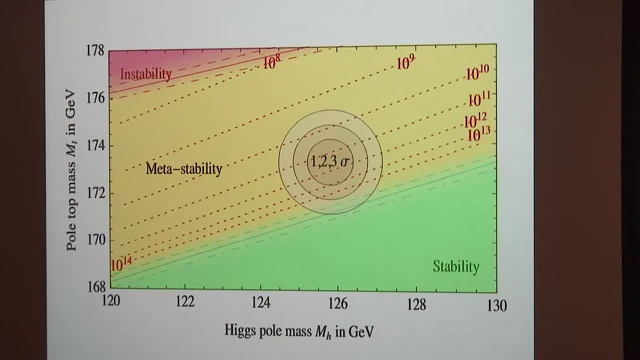 then someday we will not have this conversation anymore, Future generations will not have this conversation anymore, But the hope is, of course, that something will happen before we start exploring 10 to the 19 GeV. and how this will hopefully come about we'll talk about tomorrow. we talked. 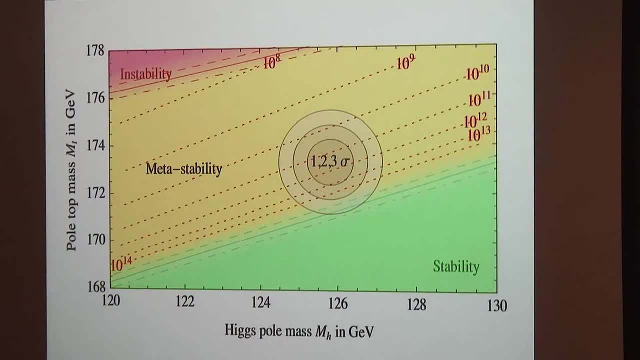 really about Higgs physics at the LHC and how we can measure stuff and how we measured stuff in particular, and what the implications are in with all of this unitarity violation business and so on and so forth. yeah, depends, I mean you, you can get threshold contributions to this. so, especially in 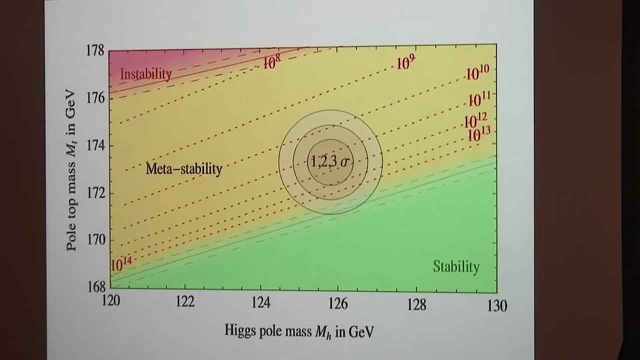 the singlet model you can get a positive contribution to lambda. just, I mean, the Higgs potential, for instance, allows you to have couplings like this: H 1, H 1 to H 2. so if you integrate that guy out, you get a new contribution to a to the quartic. 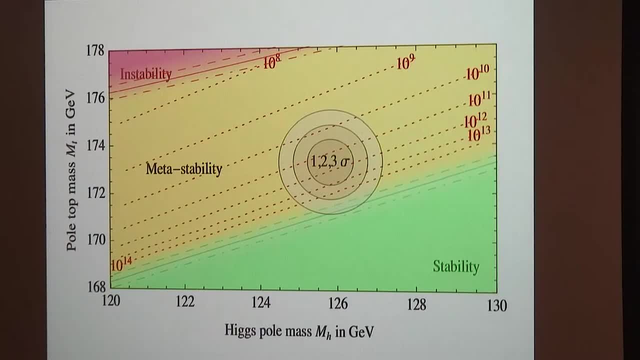 so if you have thresholds, then you can shoot yourself into the positive lambda regime and thereby essentially getting back into the stability region. so if you have new mass scales, they can alter both the RGE flow. obviously above the mass scale is relevant, but there are also threshold corrections that need to be. 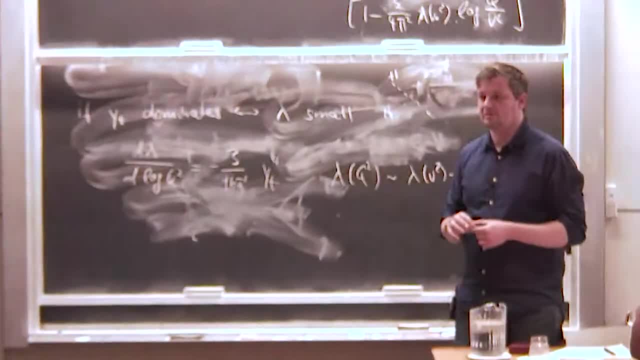 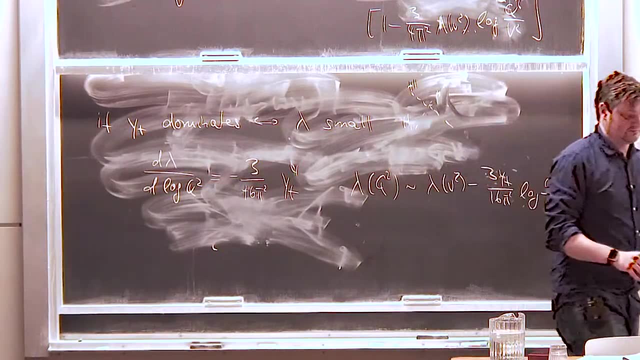 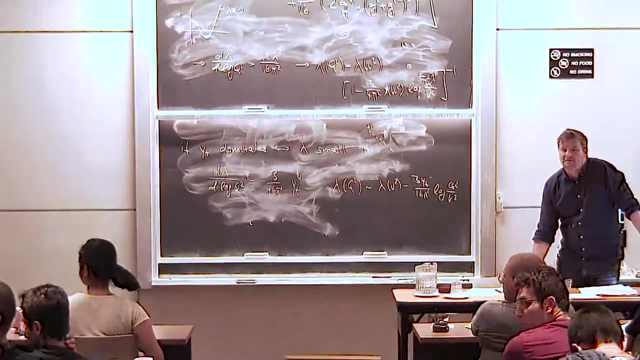 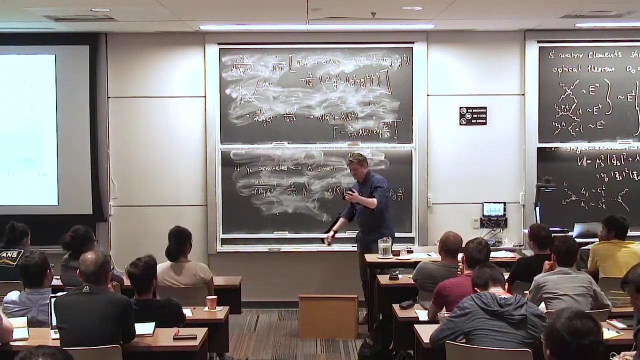 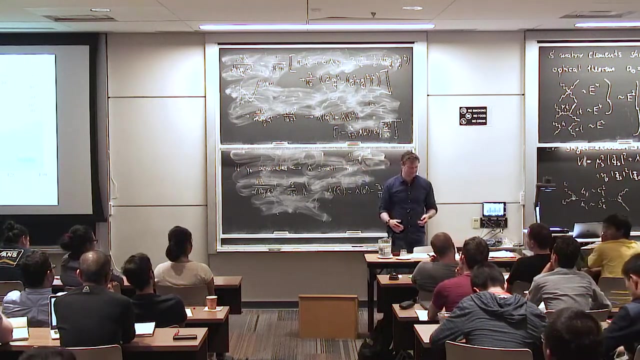 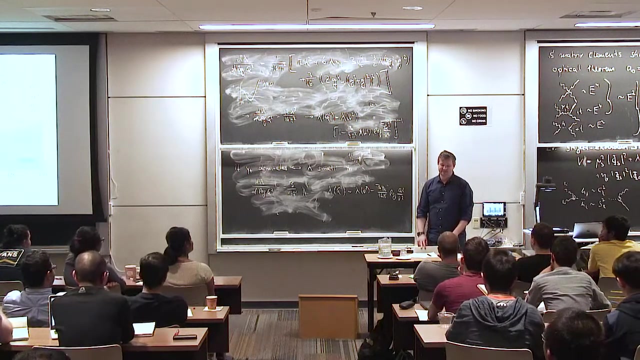 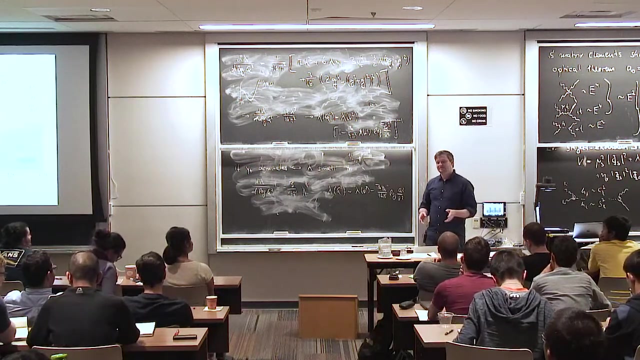 taken into account. yeah, that's one to look. yeah, yeah, the explosion, I mean the youth. there was a paper yesterday right by a York Tillman's colleague and a good friend of ours. so I think my opinion is that the is probably wrong And a very simple argument. I mean, I can't pinpoint it why, And I think 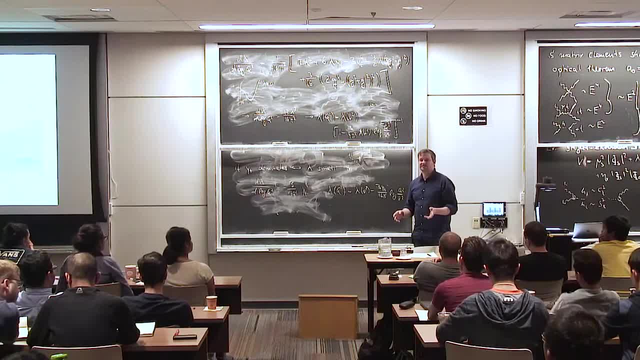 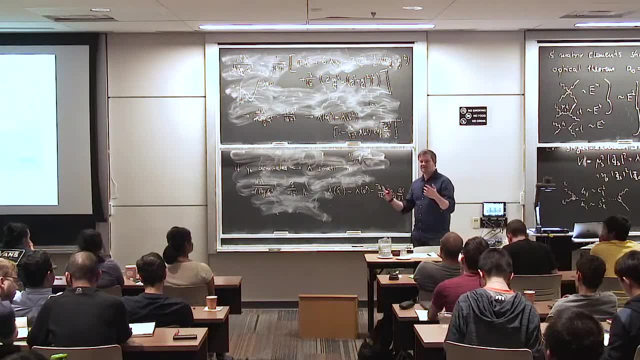 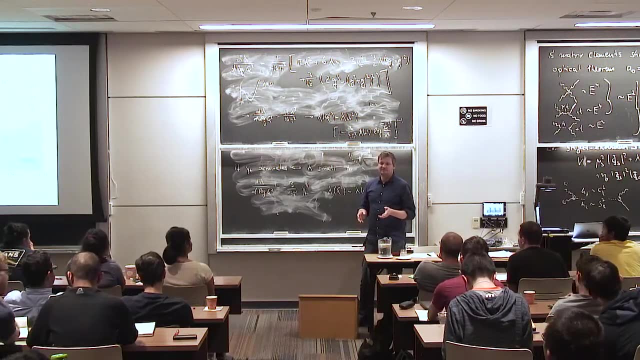 if you talk to Valya and you talk to Michael, they will agree that this looks kind of weird, But nobody can really identify what's going wrong, because these exploding amplitudes with the number of legs that you have is really a semi-classical feature and that has been. 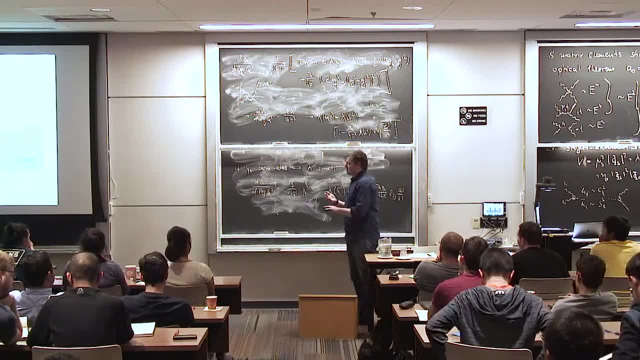 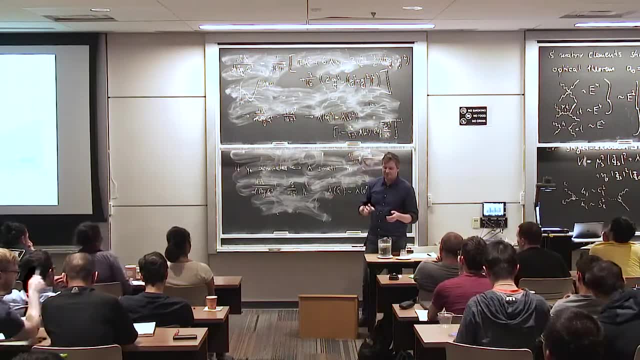 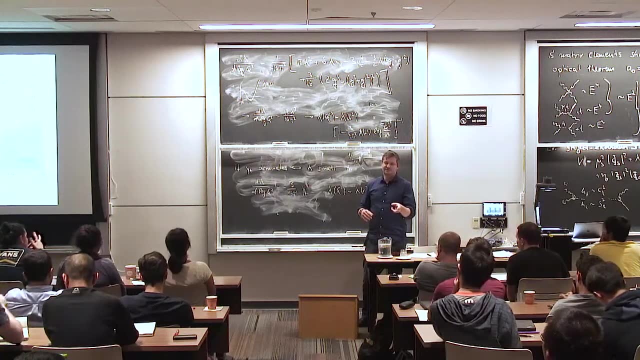 around for a very long time. So my naïve idea of how this can be sort of circumvented is- and that's pretty much what Jörg did in the context of quantum mechanics, not really quantum field theory: is that the approximation that you do, that you do perturbation theory? 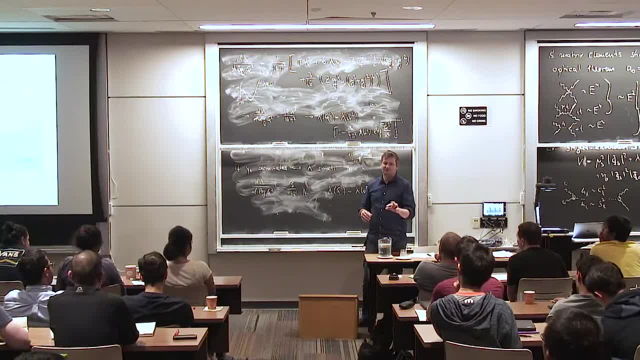 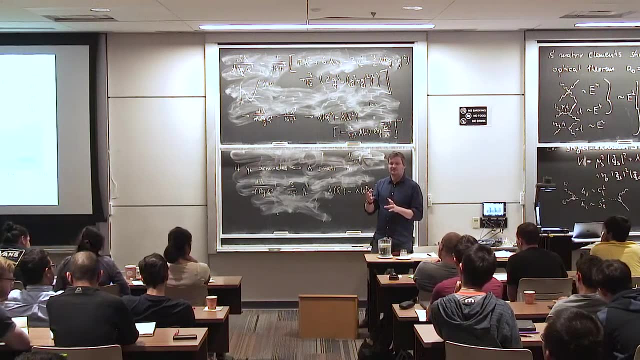 in the coupling constant is not really the appropriate one anymore, So it's a little bit like the Toft-Large-End limit. So maybe there are other quantities and Jörg identified- and Jörg and his student, I should say, identify one particular quantity that exponentiated. 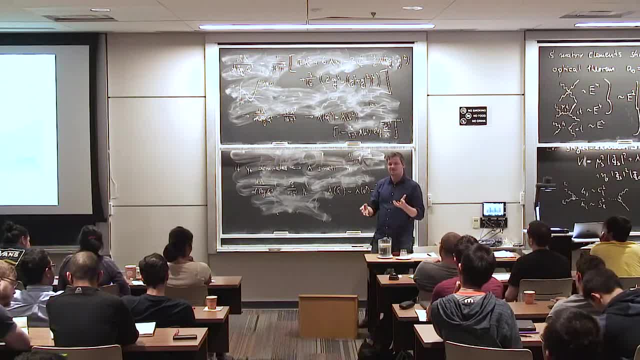 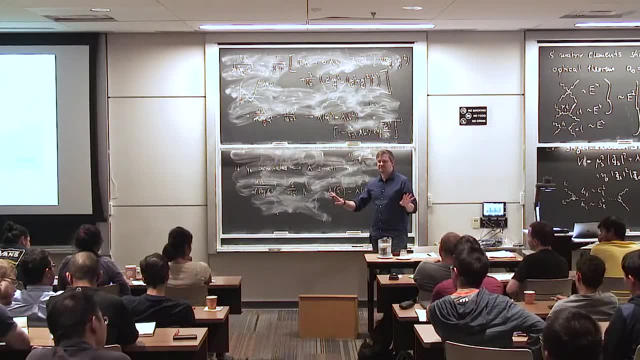 and just stems out. I mean, if you change, for instance, the way you quantize your theory, maybe this will vanish in the asymptotic states of the S-matrix. So you would get this exponential damping. So one could. next step, would you know? can you actually come up with a Boguliubov? 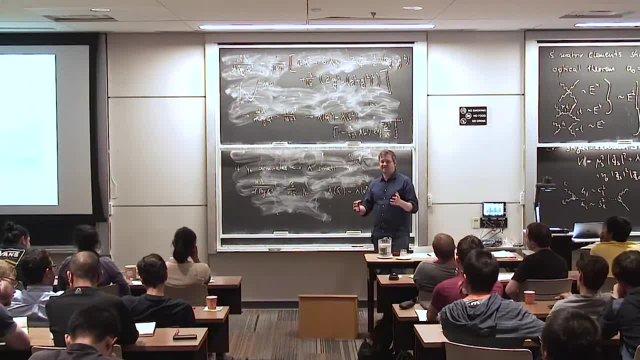 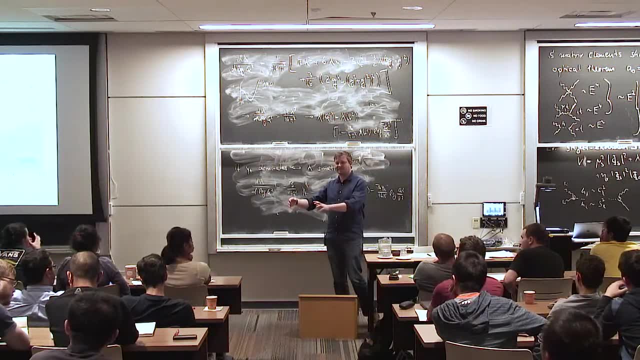 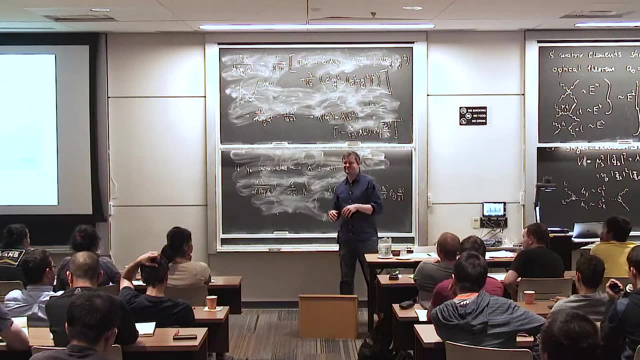 transformation that changes the quantization conditions such that you can take Jörg's ideas really to the Fourier mode decomposition of the scalar sector. and if you've managed to do that, then that's the end of it. But of course there's more work that's required there.